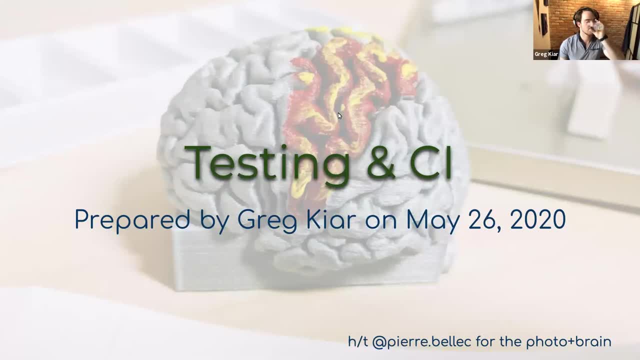 Thank you for watching. Thank you for watching. Thank you for watching. That is a good backup. Okay, I guess we can start Greg. All right, cool, All right. Hi, everybody, Hope you're doing well. So I'm going to be talking to you all today about testing and continuous integration. 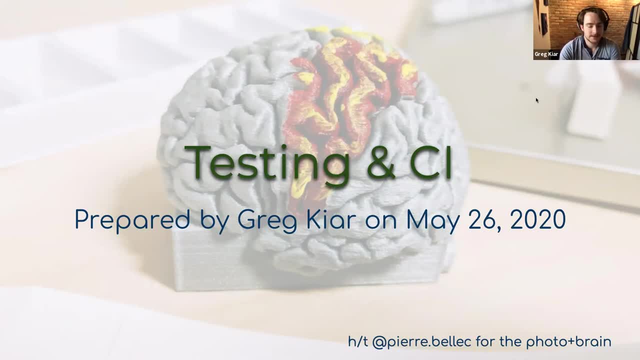 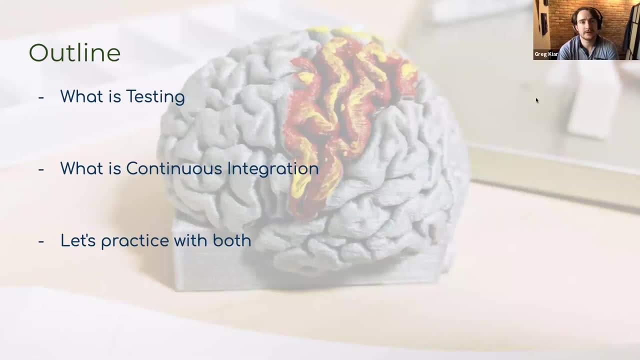 or CI as I put it in the title here. So basically the outline is pretty much as follows. I'm going to do a bit of an introduction on what is testing, what are some different types of testing? why do we do them? 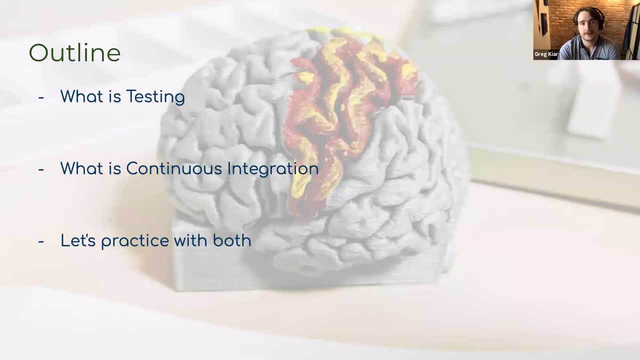 Same thing with continuous integration, And then we're just going to start practicing. So I basically created like the stub of a project And I haven't set up testing or continuous integration for it. And we are going to do that together And I again, deliberately, have not prepared. 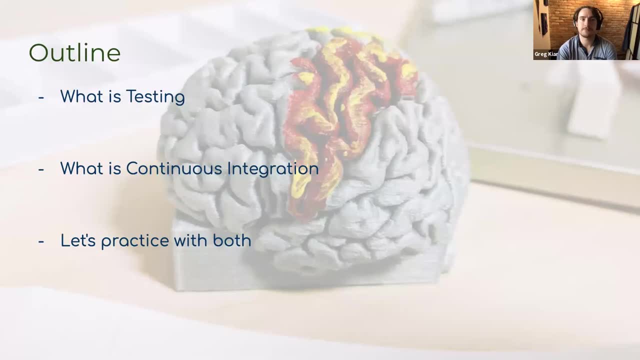 So that you can see which parts of this you know, I remember, and which parts I don't. And one thing that you'll quickly find is that the important thing to remember is more of the process. You don't need to memorize: you know all the syntax for all the little libraries. 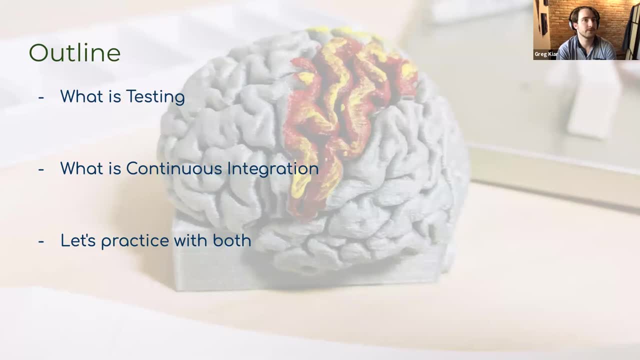 all that kind of stuff. It's very easy to find answers to all those when you need them. So this is more about the concepts of testing and continuous integration rather than any particular tool. I happen, to you know, be using whatever libraries and platforms I'm using. 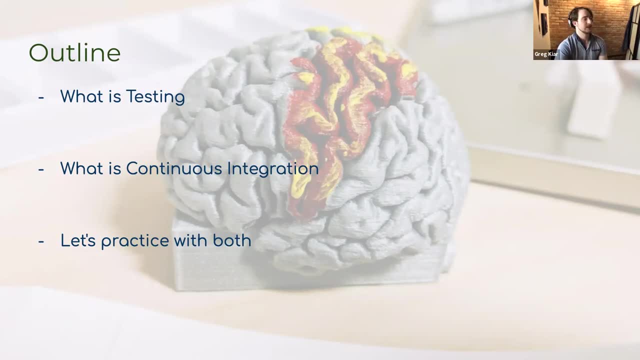 but that's deliberately not the point. Cool, So let's start with testing. So can people in the chat, or unmute yourselves, give me some ideas as to what the purpose of testing is? If you just had to guess based on you know the name of it. 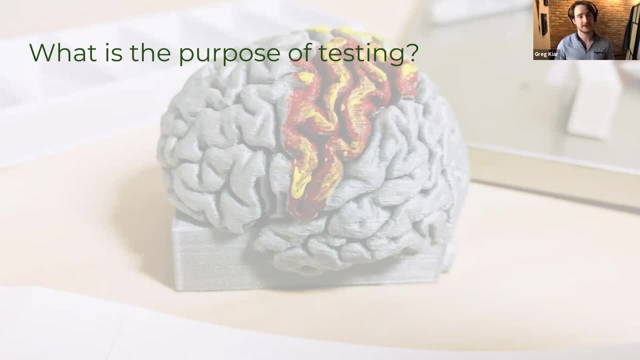 Feel free to unmute yourselves. Otherwise, just comment in the chat. I'll give you guys a few seconds to do so, depending which one you're doing, But please don't leave me hanging, guys. Um, can you hear me? Yep, I guess to validate what you wanted to work is working, something like this: 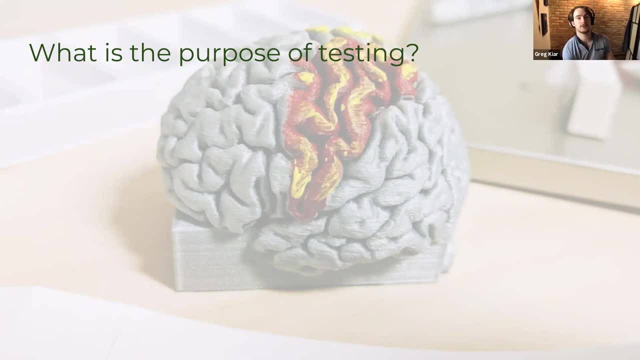 Yep, Absolutely, To validate exactly what you want to work, what you want to see working for sure. Um, and I mean that can be broad right, That can be, uh, you know, saying I want my entire end to end pipeline from you know. 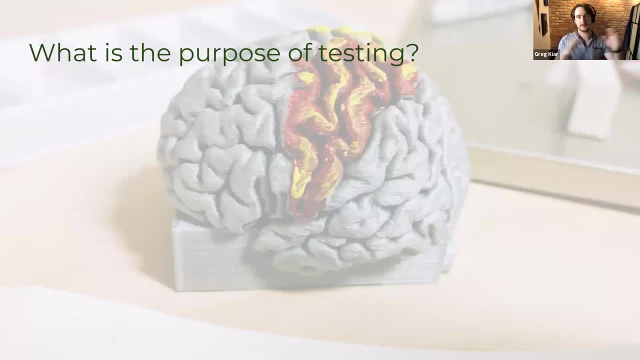 data acquisition and pre-processing all the way to my statistical analysis, to be working- or that can be any of you know, the little pieces along the way. And working is also, you know, kind of ill-defined Um, so you know it can mean that our tool doesn't crash. 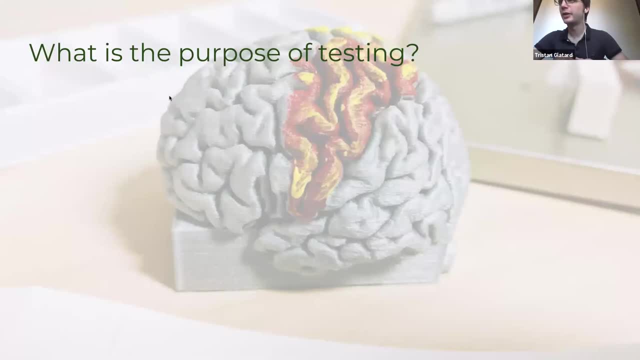 We have other. sorry, Greg, we have other answers in the chat. Oh please, Yeah, I can't see it. Make sure there's no bug. Yeah, Finding errors, Yep, And learning, Absolutely, It's mighty. 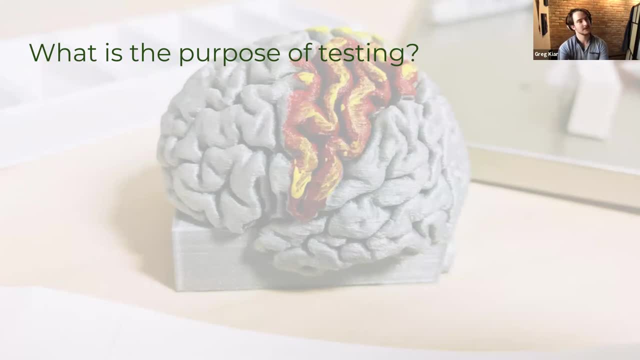 Those are all great. I particularly liked the learning one. That's awesome. Yeah, Yeah, Yeah, Yeah, That's awesome. Um so, yeah, I mean those are all great reasons and there's tons of them. So I just jotted down a few. 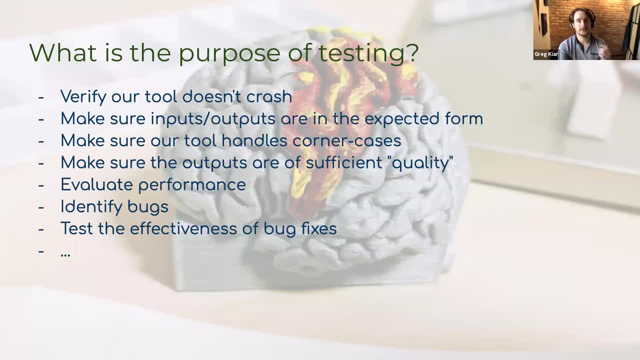 So, yes, identifying bugs is one, Um, you know, once you patch your bugs, testing the effectiveness of those bug fixes, um, you know, verifying that your tool doesn't crash because you know working can mean that your tool simply runs end to end. 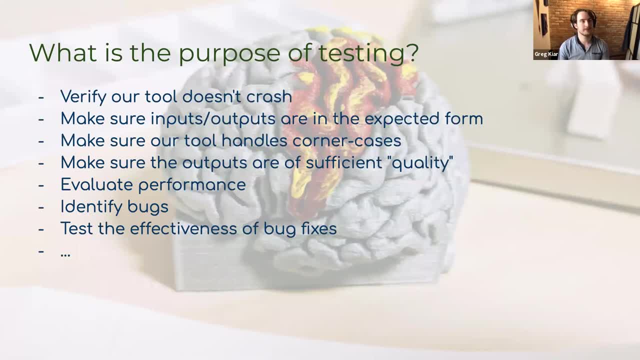 That seems like the lowest bar for working. Um, but then you know, beyond that is, they can make sure that the outputs and inputs, while it didn't crash, they're being produced and they are the right thing. So, for instance, if you're working on a project, you're working on a project, you're working. 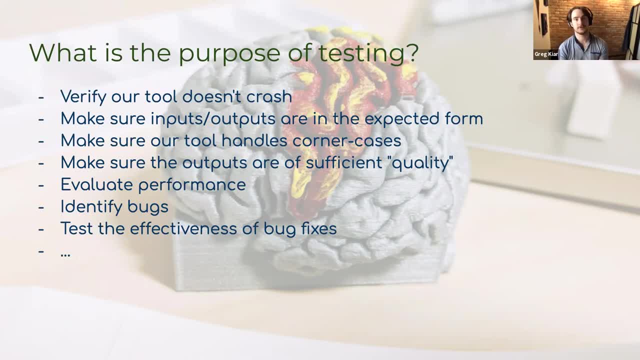 on a project. So if you're working on a project, you're working on a project. So your pipeline was supposed to pre-process a, you know, a structural MRI, And at the end of it you were just given an empty image. 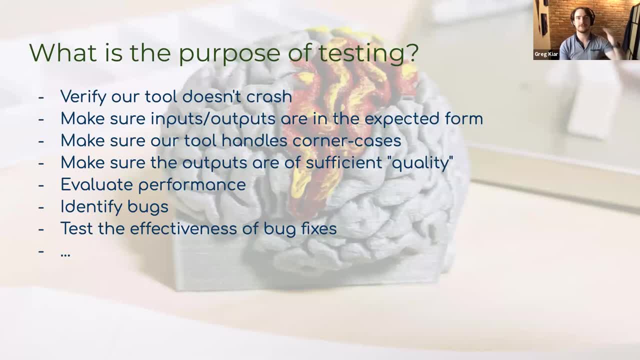 Well, that's not you know, that's. you don't have a different test to write than just if the tool crashed, versus if it's giving you like an actual, you know, three-dimensional image or something. um, you know, makes it make sure it handles corner cases. 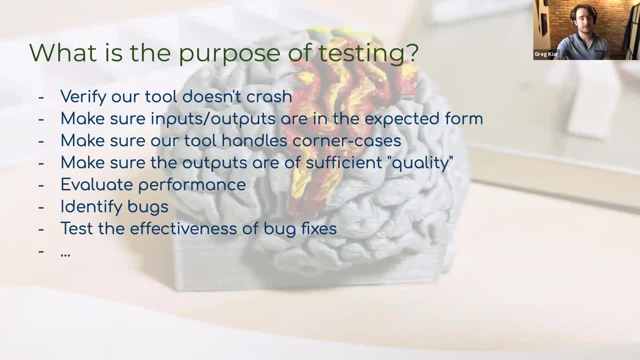 So that means you know situations where that are known to cause exceptions. Um and uh. you know doing some quality assurance, as everyone does in their pipelines, evaluating performance. What I mean by performance It's kind of like the resource requirements. 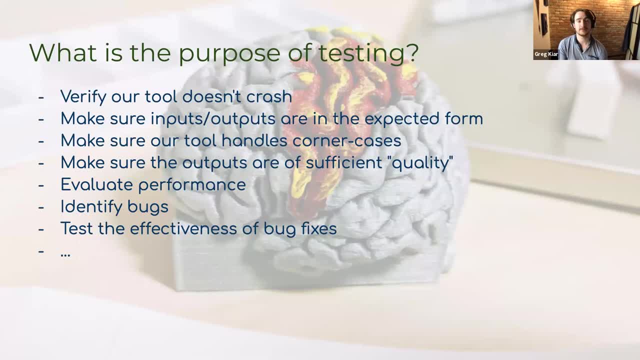 So how much you know um, memory and CPU, uh, demand the pipeline or tool is putting on your computer, and so on. So there's a lot of good reasons to test Um, but it's really yet to learn about your tool, um and uh, to try and understand it. 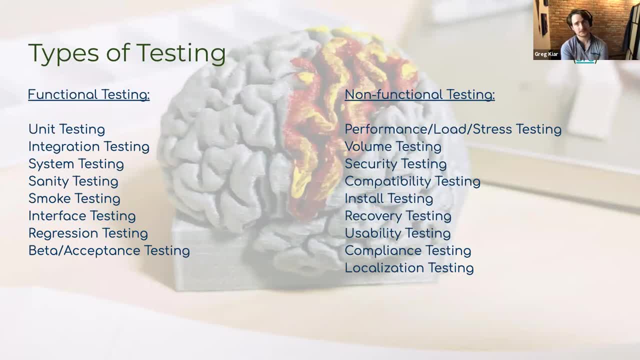 So here are a bunch of different types of testing. Um, really there's. I just got this list from some Google search, but I feel like it's pretty descriptive. Um, there's. so again two broad categories you can think of, uh, in terms of testing. 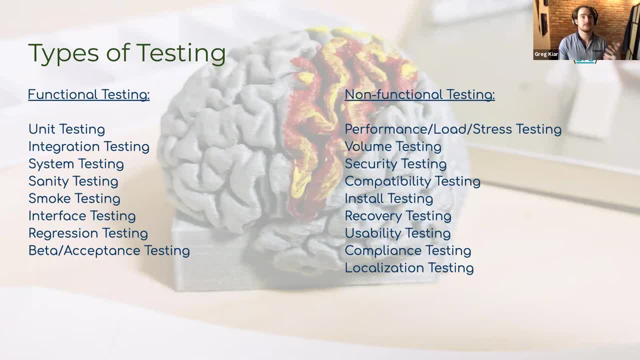 we have functional testing, which is testing, you know, the function of our, of our pipeline or our tool, And there's non-functional testing, which is more testing things that are around it. So this is again like where I said: um, like resource requirements and things like that. 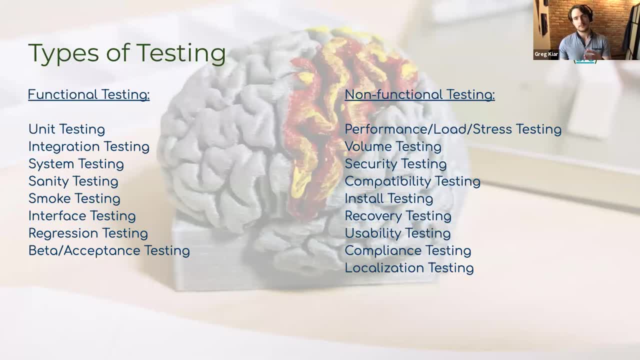 This is more in the non-functional category, because it's not testing that your tools are doing the right thing. It's simply testing what is the demand imposed by this tool. Um so, So, in terms of you know all these- there's a few that I've highlighted that we're going- 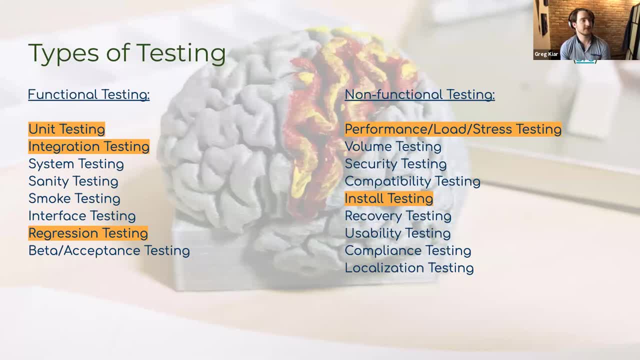 to be um working with in particular and looking at um. so we're going to be talking about unit testing, integration testing, regression testing in terms of the functional types And then, for the non-functionals, we'll be doing install testing and then stress testing. 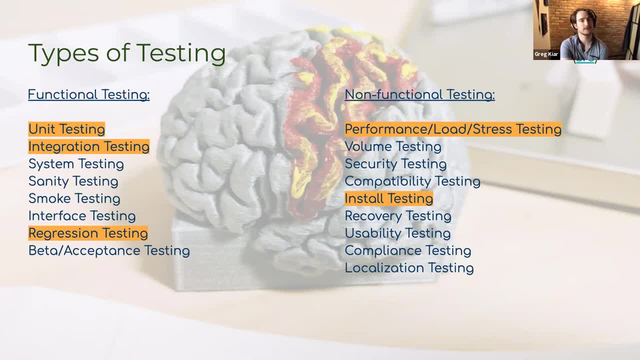 on performance load stress. They're all kind of interchangeably used. Um, Greg, uh, Ella. Ella commented in the chat saying to make sure that the program actually does what we, what we expect it to do. I think this is kind of important. 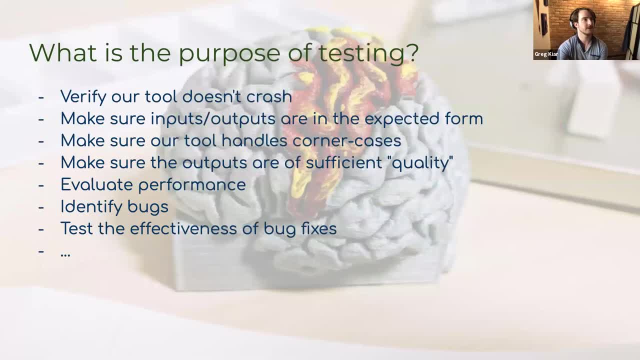 Yeah, absolutely So, right. So making sure that tool does what we're expecting to do is kind of- I'd probably put that in. Oh, I can't. let's see if I can turn on the pointer. I never had to know how to work these things. 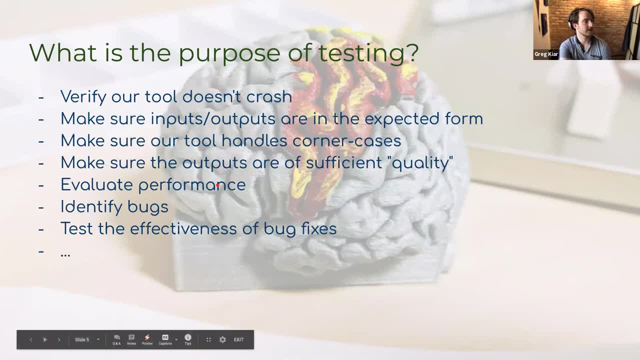 Um, I would kind of put that in. you know a bunch of these kind of span that topic. So, like inputs and outputs are in the expected form, The data is, you know, the right quality. It's not just like dumping out an empty image, but we're dumping out, you know, if we have a tool. say we're writing a tool that does skull stripping for a brain. 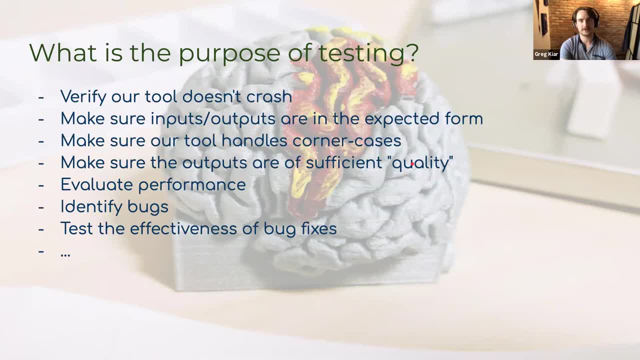 Um, we wouldn't want the output to just be the skull, We'd want the output to be the brain. So it's things like there's a bunch of different types of tests you can, you can make And, again, depending on the, on what you're evaluating, it can be easier or harder to write those. 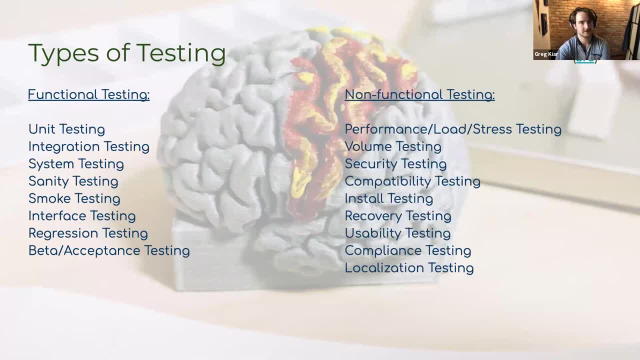 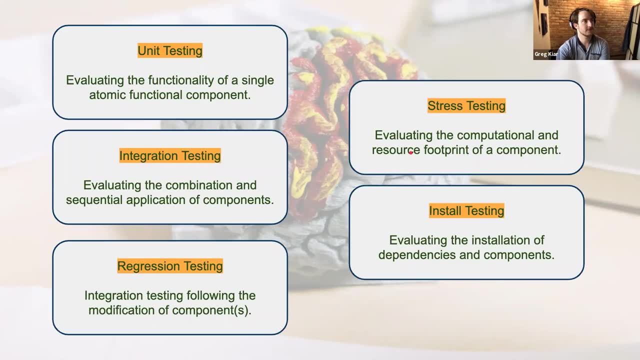 Um, but yeah, that's exactly right. It's to try and make sure that your test, your tool, is doing what you want, Um, and so there's different ways in which, uh, we can look at this, So I'm just going to give a bit of an explanation for each of these. 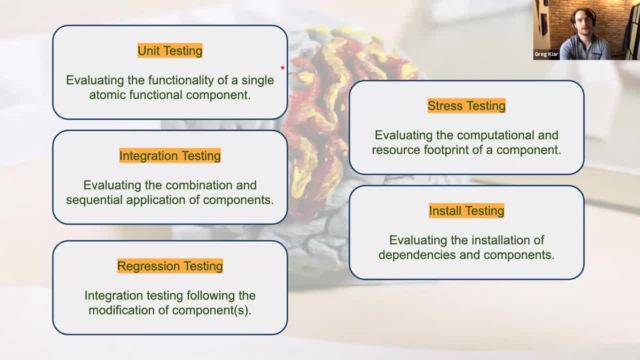 Um, so unit testing Is kind of the most basic building block of um, of testing. You have a single component, you have a single safe function and you were just testing that it performs as expected. Um, you know, you've given, say, a function that again takes a number and it's supposed to just square it. 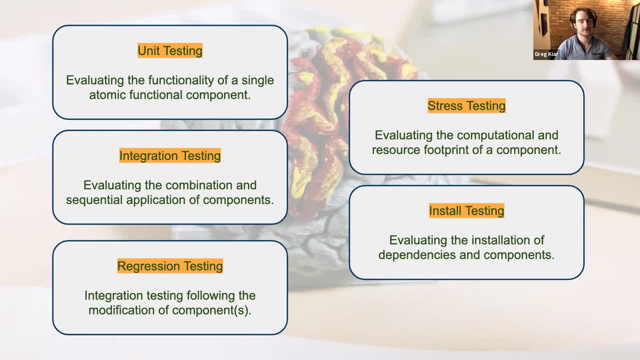 You pass it a number, you get the output, you verify that it is what you expect it to be. Um integration testing is when you essentially combine um different Units together and verify that they're not only both functioning as their independent units, but uh, but they function in the integration. 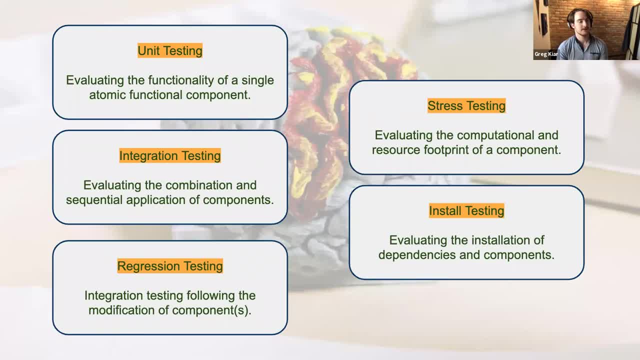 Um, there's this great, uh, this is great, Jeff, that, um, I now- I wish I pulled it up ahead of time- Um, that some of you may have seen. there's this picture that, uh, it's on the. it was on Twitter like a year ago, and it was going around where, basically, it was, um, you know, the hand dryers in, uh, in bathrooms. it was one of those placed directly above a trash bin. 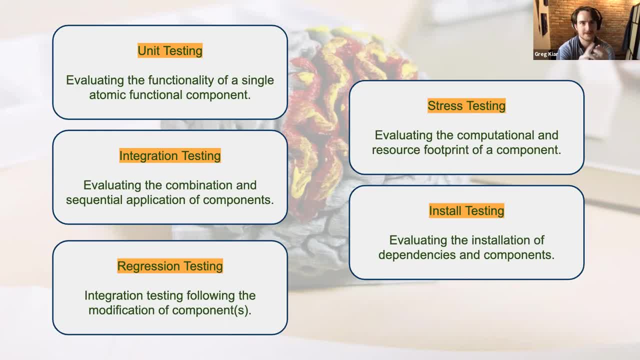 And it's a unit tests. both past integration tests failed because what was happening is when the blow dryer was on, it was knocking, it was blowing everything out of the garbage bin. So you know, independently, the garbage bin function, it contained all of the things. the hairdryer function or hand dryer functioned, it was blowing air. but when you put them together in that arrangement it did not give you what you wanted. 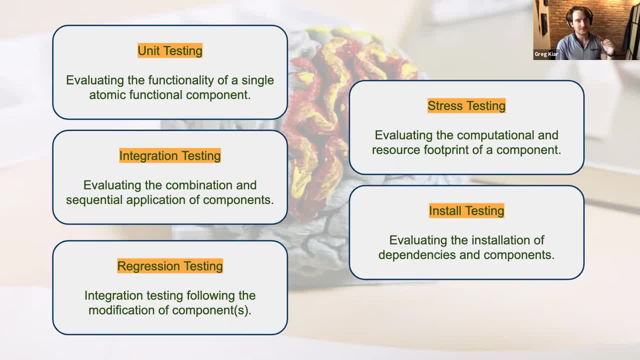 It was throwing garbage around the bathroom, Um. so that's really what integration testing is. It's using independent components, Um, and Putting them together and verifying that the result is actually what you want as well, Um. regression testing is, then, pretty much integration testing, but when you make a change, you are evaluating essentially the impact of that change, um on your pipeline and on your- on your performance. 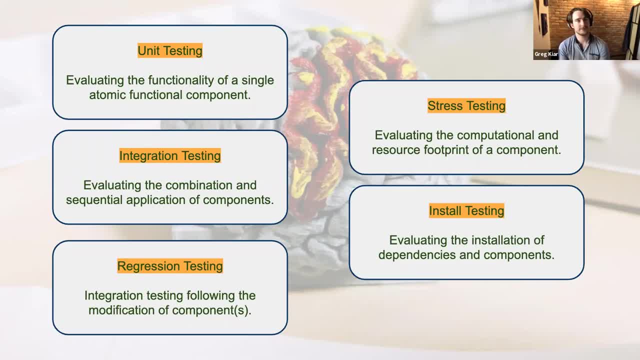 Does anyone have any questions about uh? the three kind of types of uh- functional testing- I've highlighted here. So maybe where would you put the test? Yeah, Let's say I'm writing a pipeline with the testing of a complete pipeline. 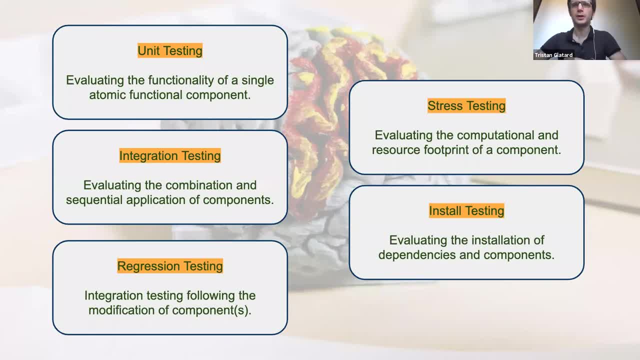 Let's say, to take brain masking for instance. Um, I'm writing a pipeline that's supposed to do brain masking. I want you know. I have a few images to test on Right Part of my test suites. would it be integration testing or unit testing? 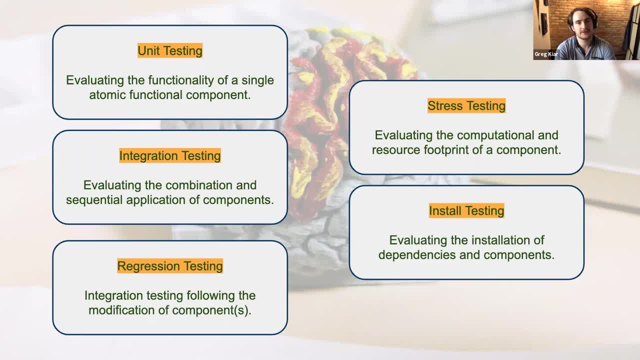 Yeah, So, um. So again, I think this is a matter of uh resolution, what resolution you're looking at. So, if you are, simply Imagine you're the Okay their extraction tool, You would probably have many independent individual components that go. 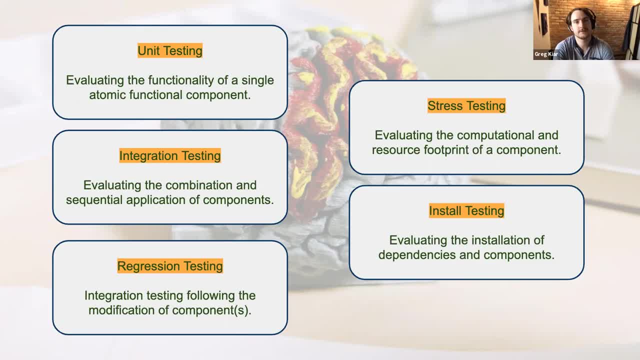 into BET and you would want to do a unit test on each of those components and then the integration test would be the entire BET pipeline. However, if what you're doing is you're taking BET for granted and you are doing other things around it and maybe adding a step before, a step after, 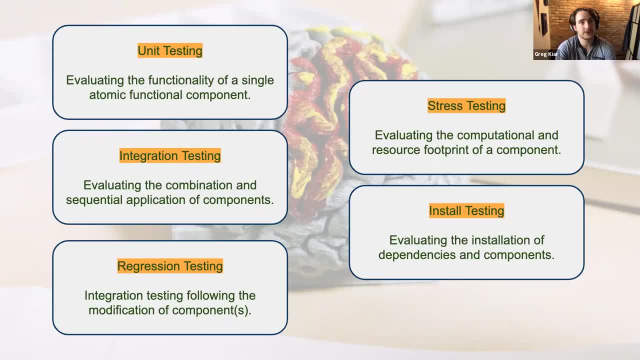 or maybe in this case, in this context, BET is a single unit for you and other steps are also single units, in which case your entire little pipeline is the integration. So I think whether something is a unit test or an integration test is really a matter of resolution. If you are. 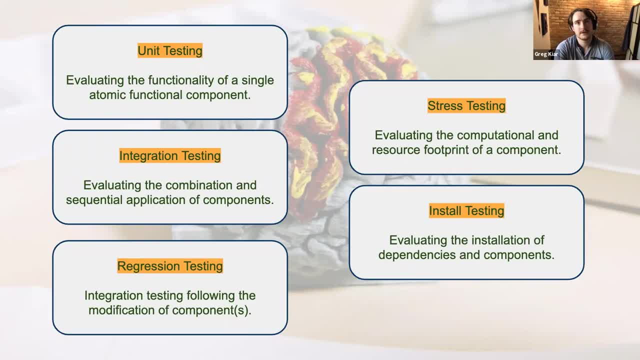 the way I'd almost describe it is a unit test should be performing a single, you know, unique function. each unit should be, rather, that you have, you know, the ability to change independently. So, for instance, again, if I wasn't an FSL developer, I would still probably. 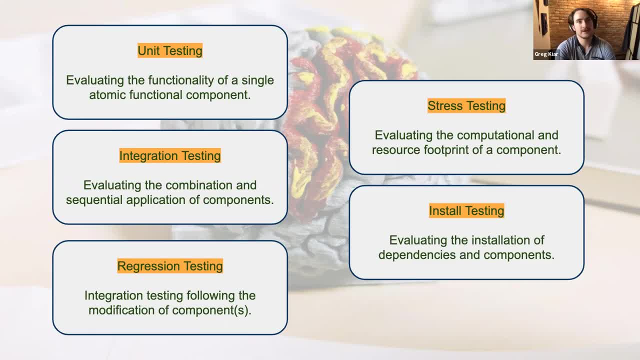 put, I would put the- you know BET as one unit in my little sub-pipeline, because if it's not working properly I can either tweak the parameters or I can use a different tool for that step or so on. But that's really what I think is as close as you can get to an atomic function per. 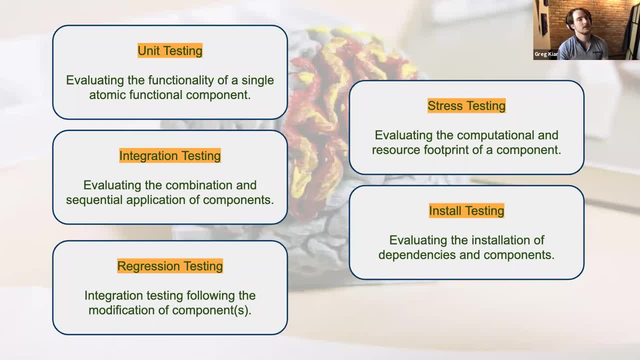 component is what you would call a unit in this testing framework. Cool, Yeah, thanks. We have another question In the chat from Nadia. could you possibly give an example of regression testing to better differentiate it from integration testing? Absolutely, When you write a program, why do you? 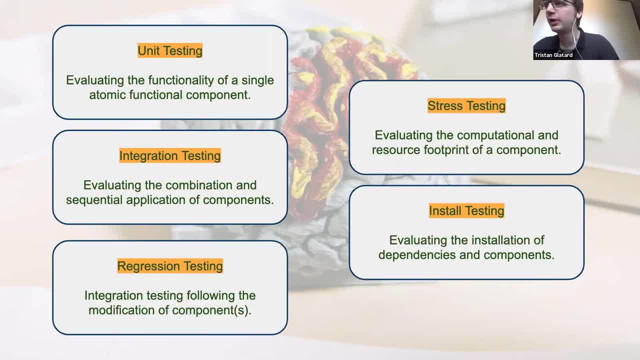 need to make sure that the program resists the modification of itself if modifying itself isn't its original function. Okay, so imagine you have this pipeline. I think I understood that. Imagine you have a pipeline that is say, generating structural or functional connectivity. 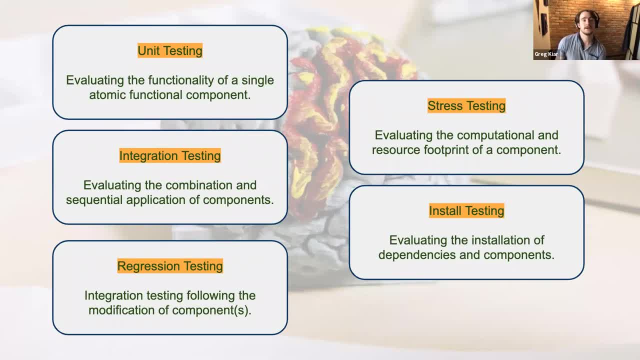 matrices doesn't really matter. Okay, so you start, let's say, the last step of your pipeline, you are doing some thresholding, And or, sorry, maybe the second last. you're doing some thresholding And then the last step is computing statistics on the resulting connectomes. If you say tweak the threshold, you're 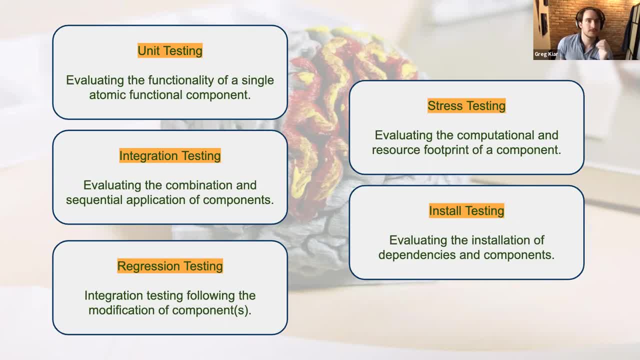 using, you will certainly be affecting things downstream from that, And how? is not necessarily obvious unless you do something like a regression test, because, again so a regression test isn't necessarily. I added this new component to that following test, but time and time again, the 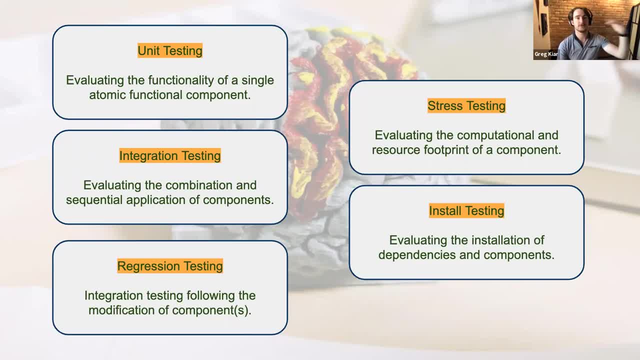 tests are necessary. So all of that comes down to how much you train your system. Okay, component, and compare it to the previous iteration that didn't have that component. It's more like I changed something and I'm comparing apples to apples. I'm comparing, you know, the statistics on my connectomes to the statistics on my. 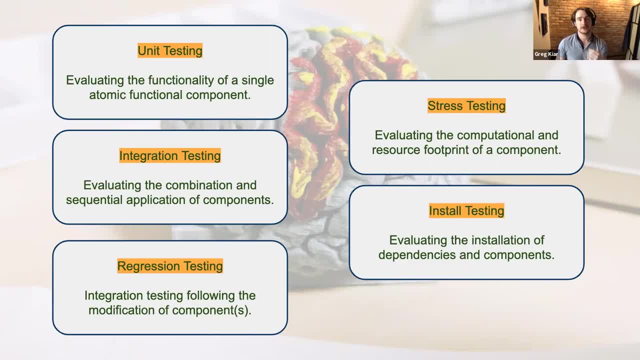 connectomes with something different in the middle that you know a consumer or a user of my tool wouldn't necessarily notice. Does that make sense, Tristan? you're muted at the moment, or at least I can't hear you. Uh, she says. uh, oh, so it has to be resistance to like parameter tuning, and then yeah. 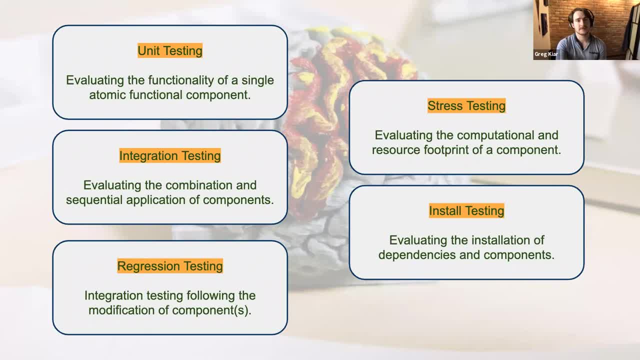 Thanks, Um, yeah, So I mean it depends what the goal is. I'm not- I wouldn't necessarily even use the word resistant- um, because sometimes you know you want a change. that's why you made it. um, it's simply understanding. 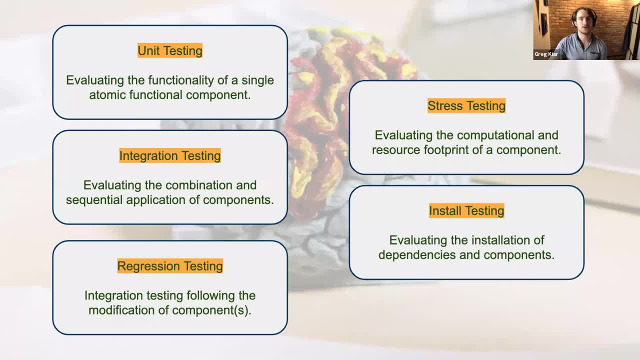 what that change or the impact of that change. So, again, the goal isn't always for it to have the outputs of like a regression test, to be no difference Again. in fact, that's often not the goal, It's just to understand. 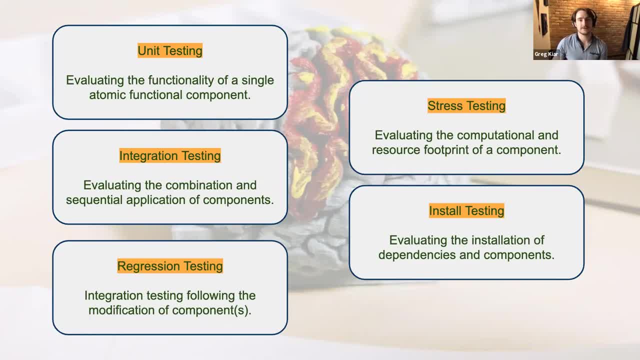 What those changes were and the impact of each of these kinds of- um modifications have on that. So, again, this could be the hyper parameters. This could be to swapping one registration algorithm for another one. Um, this could be doing all sorts of things like that, but uh, the point is 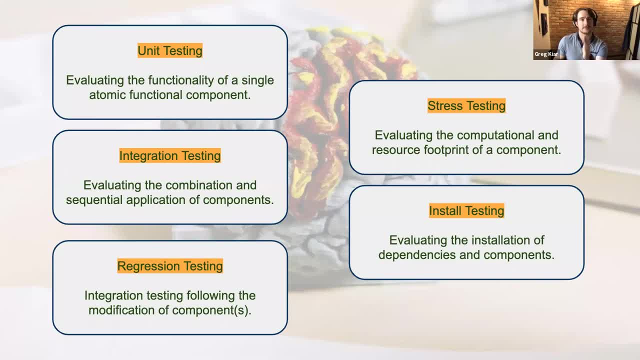 really that you are comparing apples to apples. You are comparing the same things at the end of the pipeline. Um, that again, your users would want to be comparing themselves. Does that make sense? No, you said yes, Thanks, So I guess it does perfect. 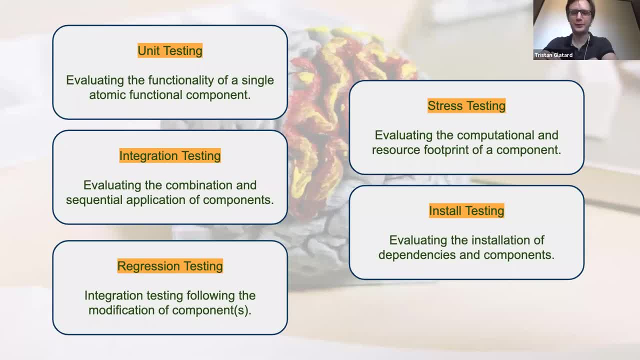 Maybe an example at a lower level. Uh, imagine you have, I don't know, two feature, three features, existing features in your pipeline, and one of them reads a number from the standard outputs. Okay, Maybe it would just, you know, read the volume of a brain region from the console, and then 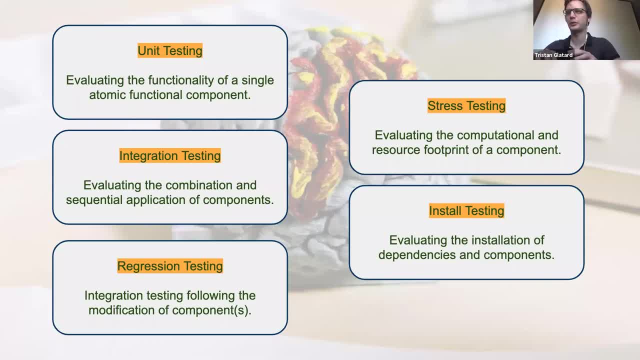 you add a verbose option to your pipeline- dash, dash verbose so that it prints more information, you know, and more messages to help people debug and understand what's going on. If you don't test, it's well possible that that feature that read from the standard outputs would be just broken by your 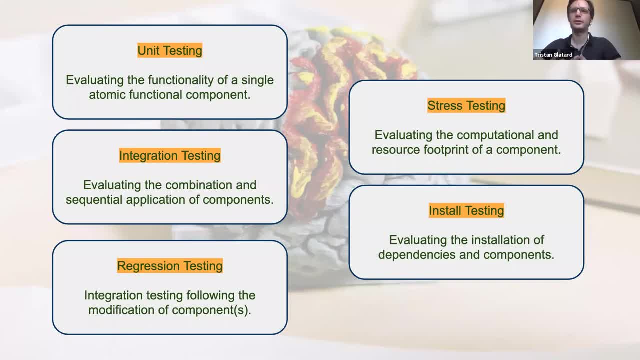 audition of verbose. And you wouldn't even realize that until you know. you would try the feature again and see: oh no, now it's not parsing a number from the STD art, It's passing, you know, whatever information string. 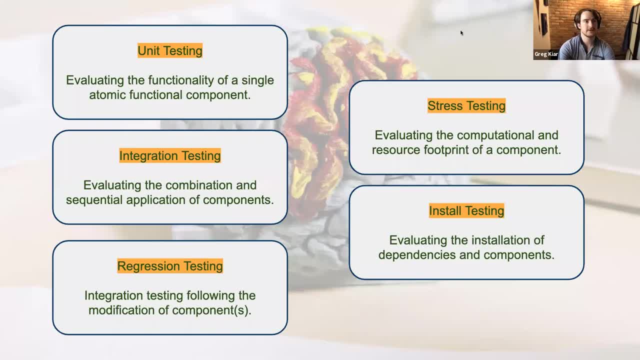 Yeah, that's a great example And I think it's important. It importantly illustrates that um, you know the uh, the changes don't have to be Yeah, Meaningful, like deliberately meaningful changes in your pipeline, And it's impossible to know whether or not they will be without testing. 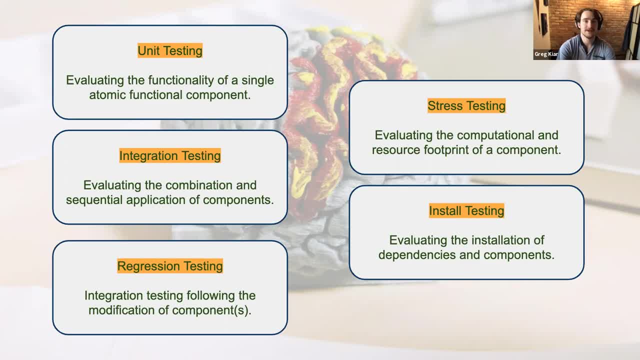 Um, because right, little things like adding a verbose option, um, that changes the alignment of texts, Um or like: if, for instance, you're saving a data frame and you um basically say like index equals false and where before it was true. 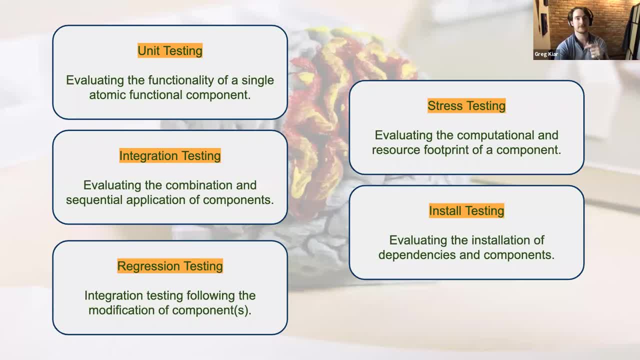 So you're no longer printing the index column. Well then, if you have another thing, that's reading a CSV file manually, maybe? Um, you will be grabbing from the wrong column than you were before because there's one fewer columns in the table. 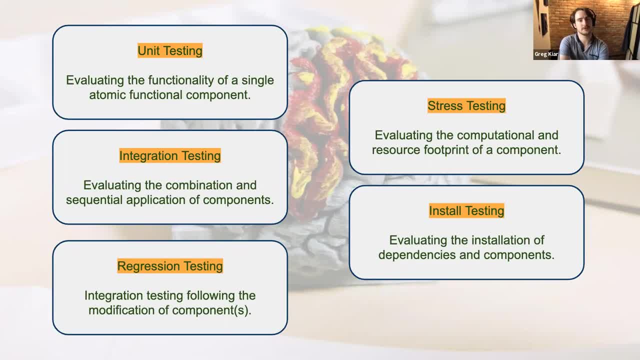 So there's a bunch of things like that. that it's just. you know, there's a lot of moving parts when you start building multi-step pipelines and processing tools and things like that. Um, and really the only way to know which pieces impact other pieces is by testing every combination that you can think of and always um doing things like regression tests, which is again where continuous integration comes in. 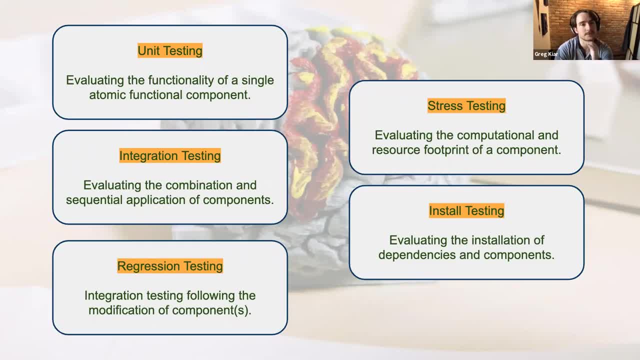 And I'll get to a little bit later. Isabel is saying: to just think of a software update. um has like this is an an example too, right? And I think, of course, yeah, software updates Exactly From a different version of a library. 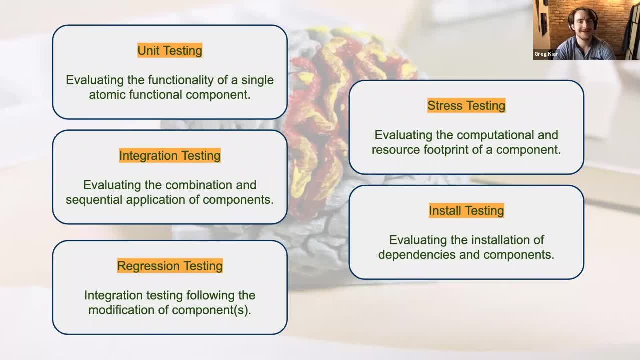 Um, that's exactly what's happening, And they will have done, hopefully, uh, regression tests and say: well, you know this feature no longer works as expected, You know this will give a slightly different output, So on and so forth. 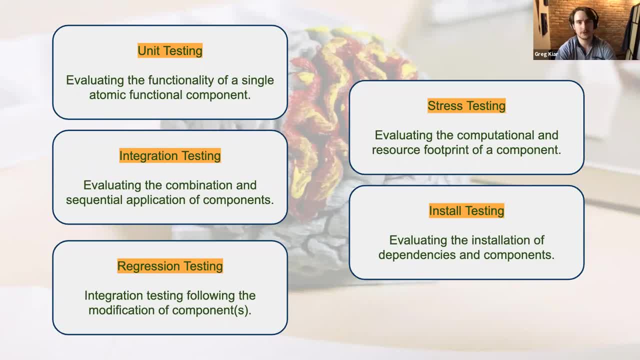 And hopefully these are well-described in like a release notes type thing where it says: you know our latest version now with whatever Um, but uh, but yeah, this is. it's exactly for the purpose of versioning Um and again, as a scientific consumer, this is particularly important, you know, if it's for like a plotting library, you know who really cares. 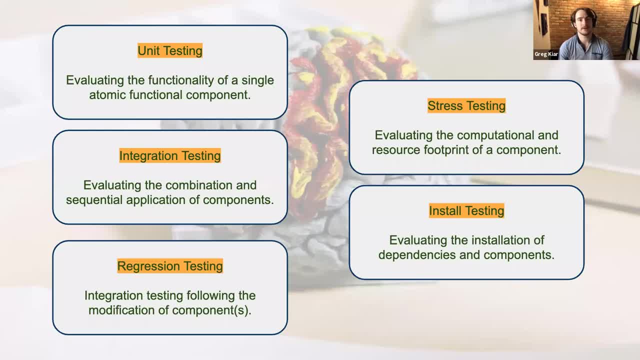 We'll switch to the new syntax. We'll, you know, update and accommodate and follow along. but from a scientific perspective, if you know, we're processing our data a certain way and let's say, Let's say we came to a, you know positive results, um, meaning, like you know a significant P value or whatever that means in our context. 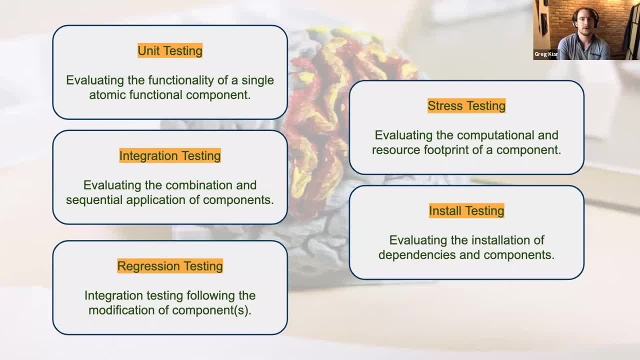 And then we update our tool and now it doesn't. the result is no longer significant. Maybe that bug fix? maybe it was a bug fix. That means we didn't have a real result before. Maybe it's just a processing choice That isn't necessarily a bug fix, but just a change, um, like a lateral move. 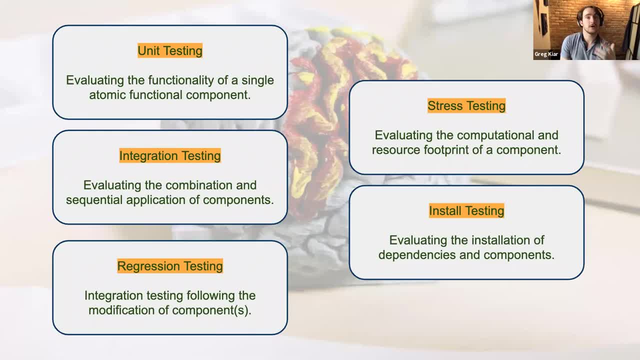 And it's important to understand again what those changes are and What impact they have on our um, on our results. So, as scientific users, it's really important to do things like regression testing, Um, cool. So then, um, just to go into the non-functional types of testing and, by the way, keep asking questions and, Trisana Valerie, thank you for reading them to me. 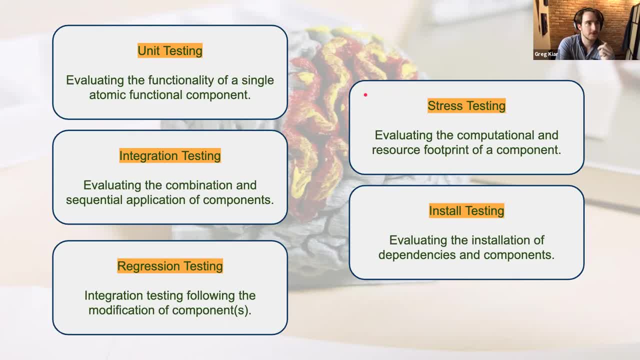 Um, but uh, but yeah. so um, to the non-functional types of testing, and I don't know if any of you have spoken to Valerie about her work, but it kind of falls a lot into the realm of trying to optimize for really high. 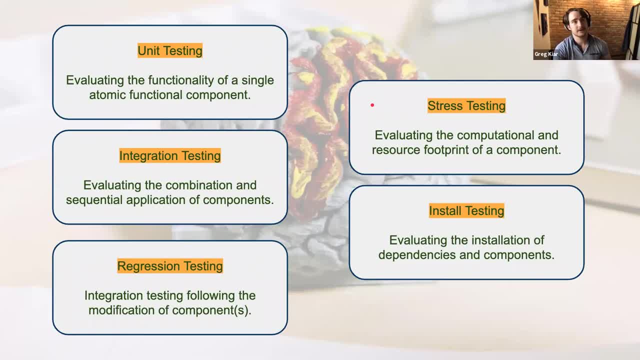 Start Stress type workflows. Um, so stress testing is again evaluating what is the footprint of um, of your uh, your tool. So again say you're working on a massive dataset, you know a terabyte large uh image or or something like that. 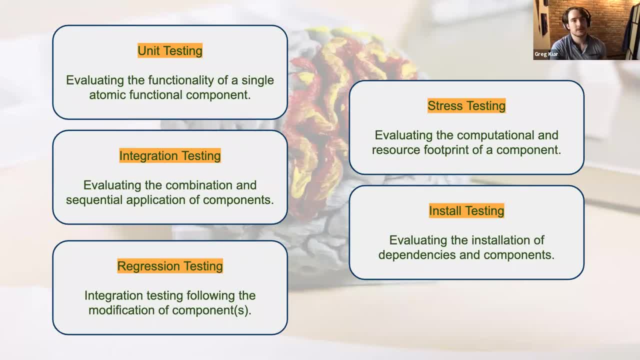 Is there a way that you can process this in memory? Is there a way that you can understand how many resources are being used at a time? How long is this going to take? and all this stuff, And you know, as you guys have been- um slowly, I think- getting introduced to the concepts like high performance computing. 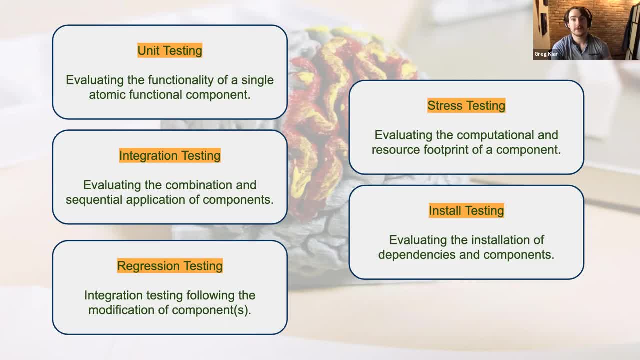 And using compute Canada and all that. um, it's very important to understand the stress of your tool because then you know how many resources to request on uh, on shared systems, and you can be like a good computing citizen basically. 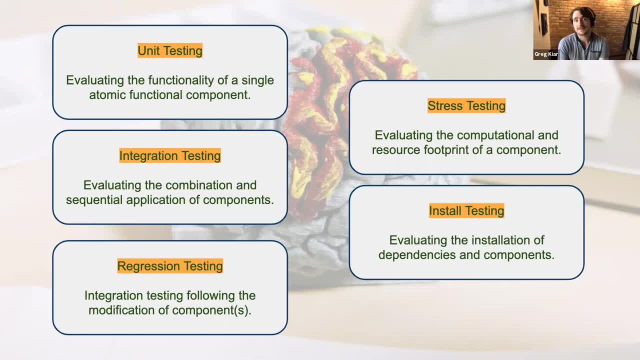 Um, and then, of course, the last one is the most obvious: install testing, making sure that you don't have conflicting versions of dependencies. making sure that you know if I need a really old version of NumPy, because I really liked the way that they implemented a function then, but I need a really new version of psychic learn because 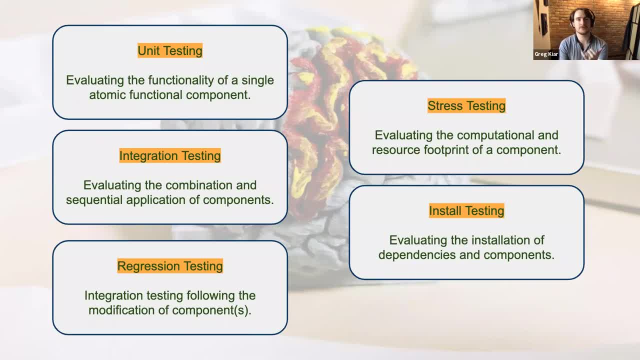 They just implemented a new algorithm. If those are mutually exclusive or not like if, for instance, I could learn requires a newer version of NumPy or whatever it is, um install testing as a way just to resolve all of that and make sure that at any moment when you make changes, your tool can still be installed successfully. 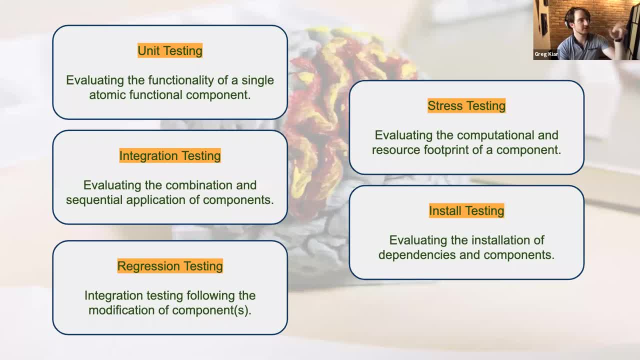 Um, so we are going to do some version of all of these. um, granted, uh, we get through it all in time. um, on this little kind of dummy project I made at the end. Um, but, uh, again, keep firing off questions about testing in the chat before. uh, before we move on. 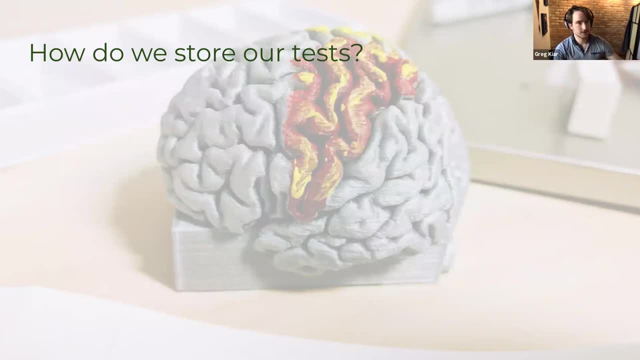 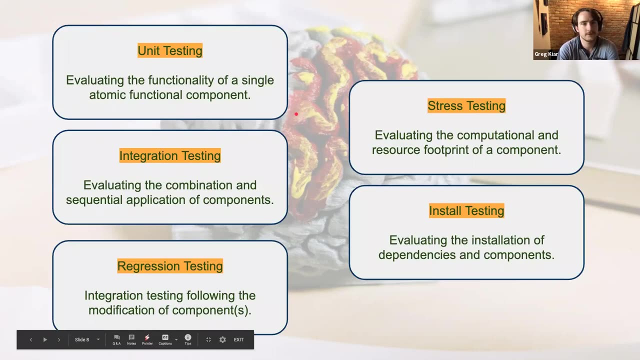 But, um, but then the next question is: really: you know, given that we know now to some extent what types of tests we want to run, you know, I want to test, you know, my skull stripping algorithm. I want to test my entire pipeline. 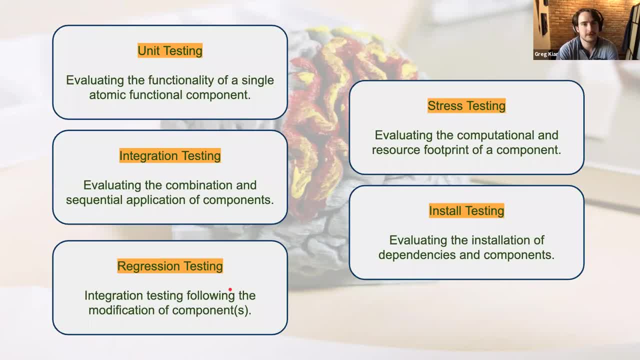 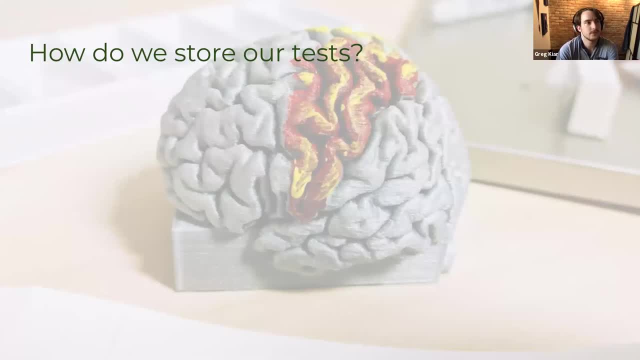 You know, I want to see how changing my thresholds affects my result. Um, you know how do we store these tests? There's a bunch of like, there's a many different Ways and it's you know, in one, in one way. you know we could store it as a as a function. 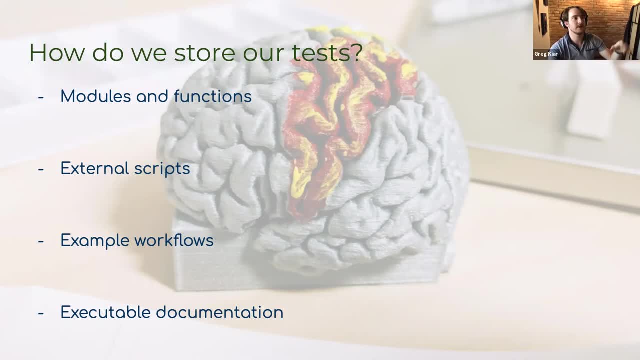 We can simply have a function that calls our entire pipeline, and there it's another module that basically calls our tests. We can have external scripts, we can have example workflows, we can have executable documentation. So there's many different ways you can write tests that will effectively do the same thing. 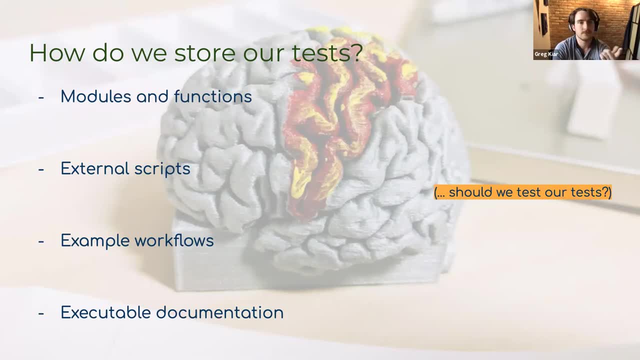 And um, and this is also an interesting point which begs that if we're writing functions and scripts and workflows for our tests, The point of having this slide is, then should we test our tests and this so there's a rabbit hole kind of that you can fall down? 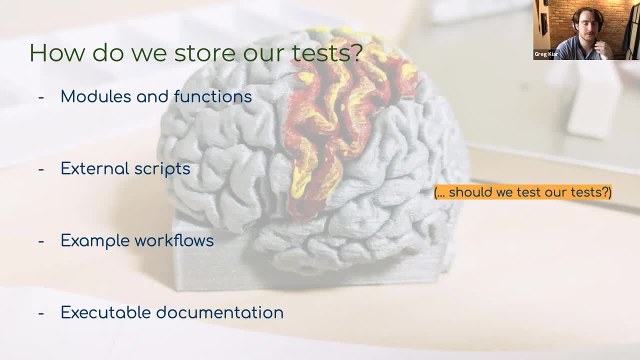 Um, and there's something that I won't probably get to today, Um, but it's worth looking into. That's basically code coverage and there's a bunch of different other tools like this Um, but pretty much what they said. what they allow you to do is say, well, this tests, you know, um covered a hundred lines of your module. 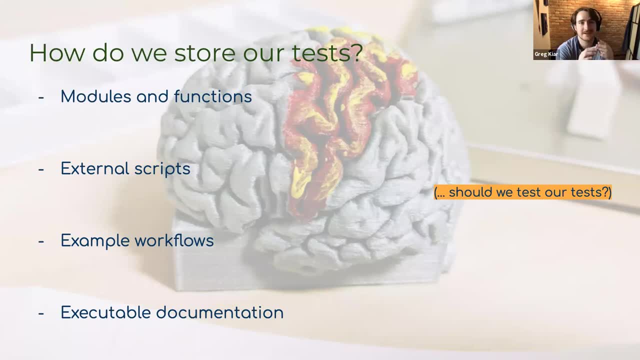 Um, this you know, just in general, you were testing 85% of the lines. Okay, You know, each line is, on average, being tested five times or two times or or whatever. Um, and so you can get like good summary statistics about how well your tests are actually. um, you know, spanning the the library that you're working on, 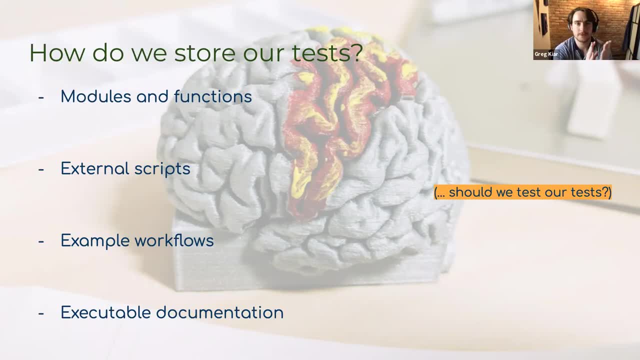 Um and uh. and, by the way, in case anyone's really curious about this type of stuff, I've got the on the last slide um, and I'll post these in content if I haven't yet. I think I haven't yet. 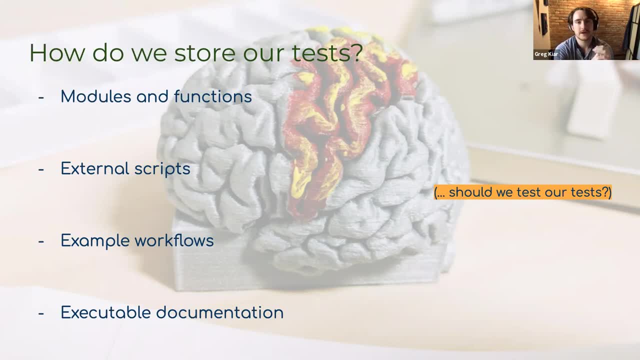 Um, but uh. I've posted examples on the last slide that Um showcase, you know, projects that have these types of integration and send testing suites and have like coverage reports. You can get a sense of different libraries that you can use to evaluate your tests themselves. 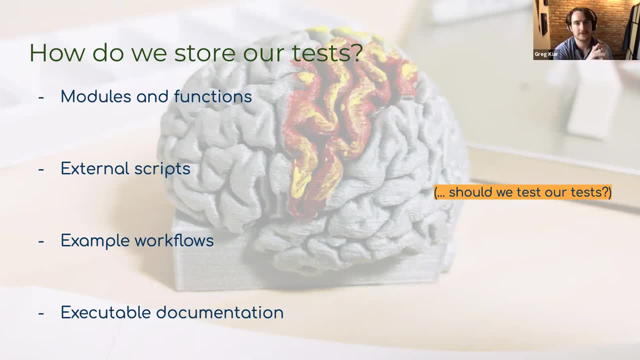 Um, you know, run them and uh and get a sense of: am I really doing a good job at evaluating my um, my tools, And some of these are, of course, harder to. you know there's a limit to this and that I can't necessarily have a good test that I'm able to say with certainty. 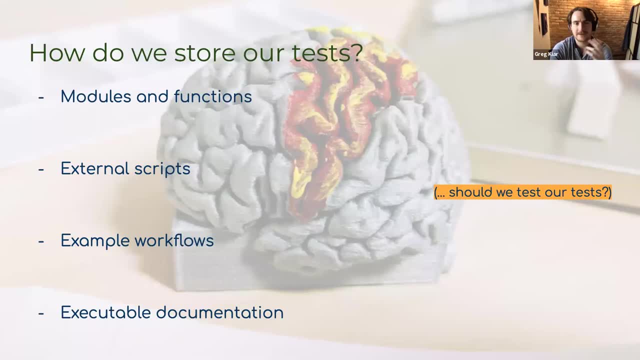 It's an effective regression test. Um, scientifically again, like I wouldn't, it's, it's conceptually. we need then some theory about: oh, is it conceptually meaningful that? um, you know, my graph is now more sparse because I changed the threshold, or something like that. 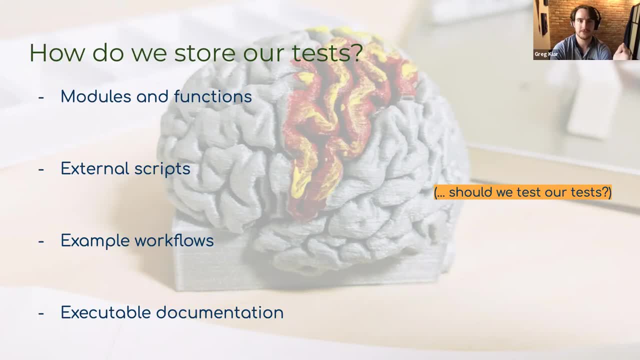 So, of course, there's a limit to where this reaches the bounds of like this is now science and no longer like software development, Um, but in general, this will get you most of the way for um, for practical purposes. So then, I guess this all kind of begs the question that we've talked about. 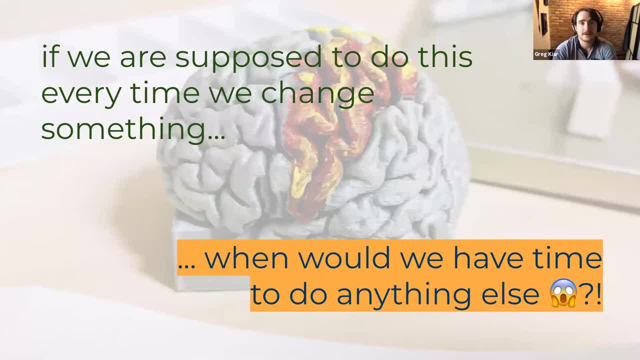 We've got a lot of different types of testing and lots of different ways we can encode- uh, encode them- And then lots of ways that we have to even test them. So if we're supposed to do this, every single time we change something, add a new function, whatever- will we ever have time to do something else? 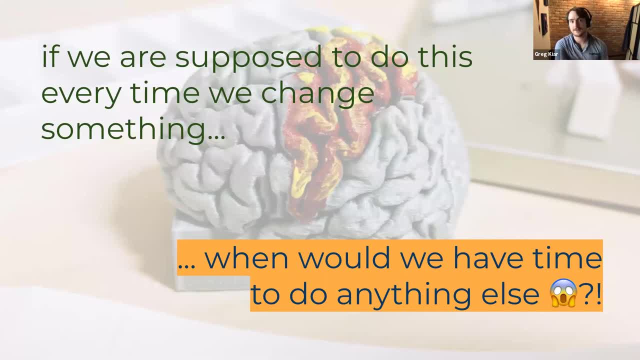 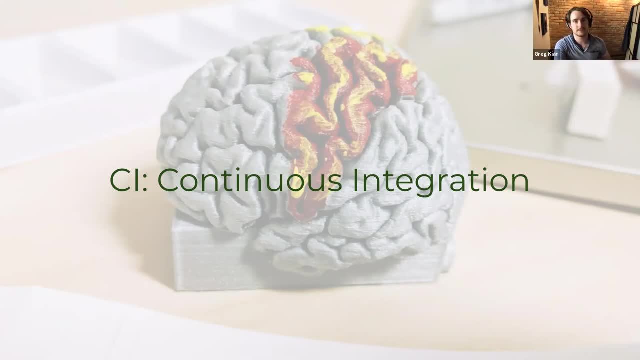 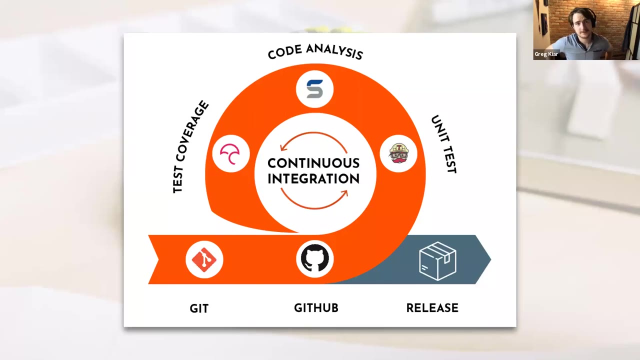 And that is essentially why continuous integration exists. So CI, continuous integration- I will jump back and forth between the names as well. Everyone who talks about them, Um, so get used to seeing both Um. but what's a continuous integration essentially means is that if you have some repository- so we are, have all been, you know, experts in get at this point. 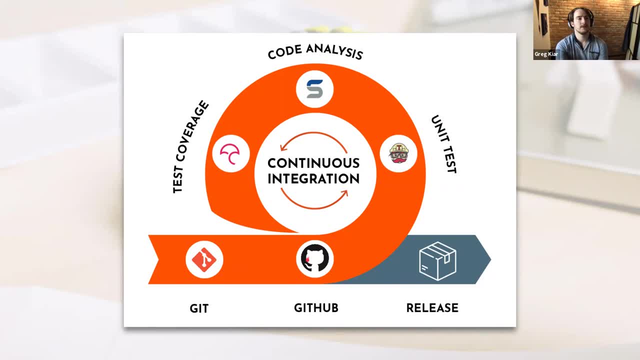 Um, and we know we store, store our code on GitHub. What we then do is we can integrate it to some platform that runs our tests for us. It'll again potentially do our like analysis of our code or test coverage that I was talking about, and then it'll give us a report. 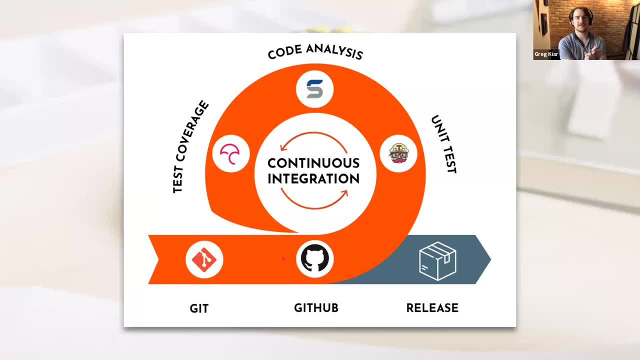 And what that report will say is: you know all of your tests passed and your code coverage. you're testing a hundred percent of your code and, my goodness, your code is written to an eight plus plus standard. Look at this amazing formatting. yada, yada, yada. 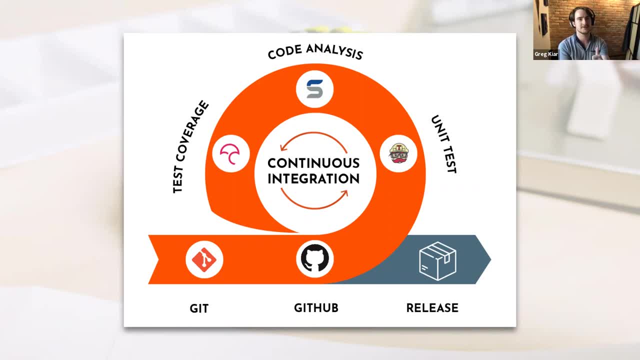 Um, by the way, I've never once gotten a report even close to that good, so don't worry, Um, but uh, but then it'll give you all these reports and you can really understand. okay, you know what has changed from my last version to my new version. 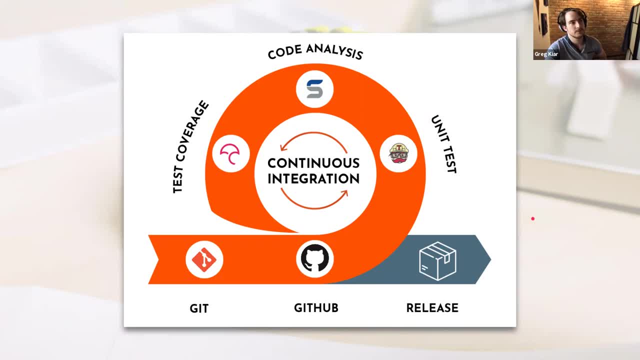 Um, and then you can go forward with releasing it So, um, so again. the nice thing here is It gives you a way to kind of have, uh, an asynchronous feedback loop. You can develop some feature, you can push your changes up to get out of. you can keep developing. 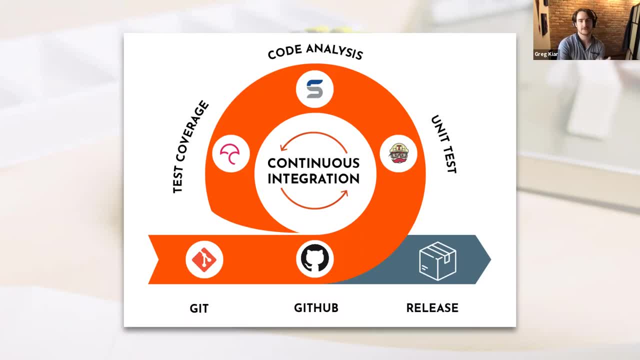 And while you're working, or working on a different project or something, um, at some point you'll get an email or a GitHub notification, or however you set up your notification preferences, Um, to say your tests are all done. come look at the report and, uh, it'll often say: you know, this feature broke, or or what have you? 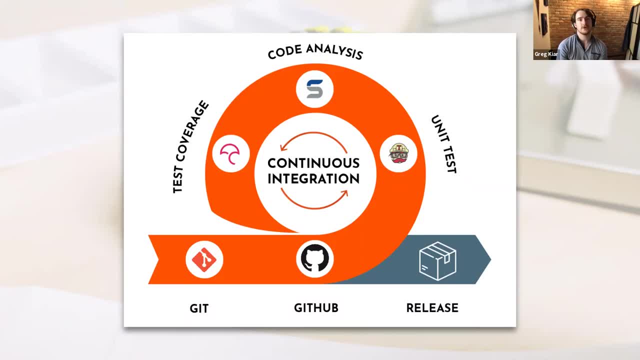 Um, and it allows you to Again, before ever releasing code, before ever sending it off to a user, to say, um, oh, I want to use my pipeline. or or even again sending it to like a cluster yourself, for I'm not going to use this version of my tool in my in my next paper. 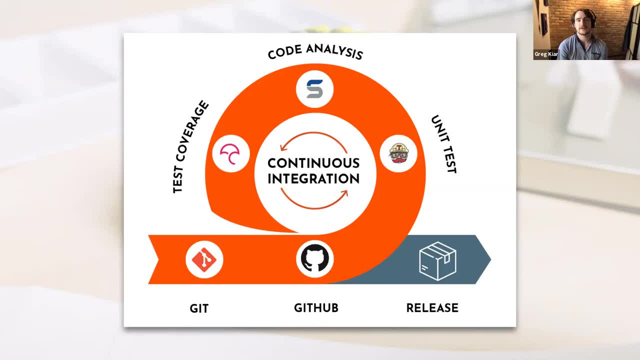 Um, you are, you know, making sure that it's doing what you expect it to do and reducing the amount of time that you spend creating, running, finding a problem, debugging, fixing, then running, And you know, Because you know resources are expensive. 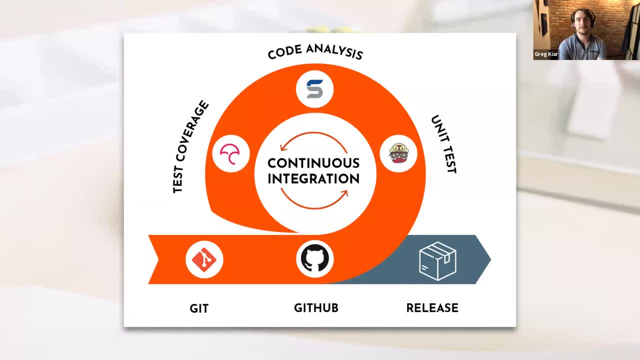 This is the stress test. is, you know, meaningless if you have to run your code a thousand times? Um, so, uh, so, really, this is meant to have a tight feedback loop between the features you're developing and their evaluation. Um, does anyone have any questions about kind of this um workflow? 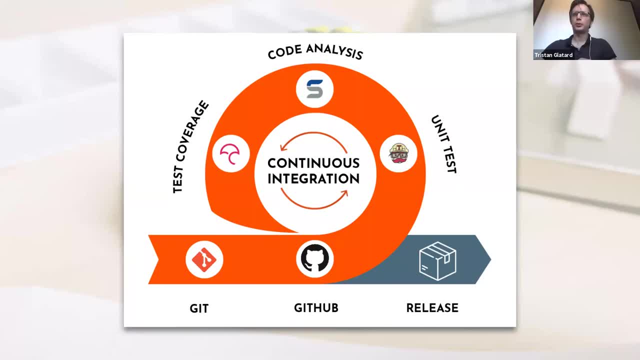 Maybe a brief one. So just to um, to try to touch on um scientific data testing. So imagine you have some data here, like like I mean, obviously if you're testing a pipeline, you you would need some, some testing data. 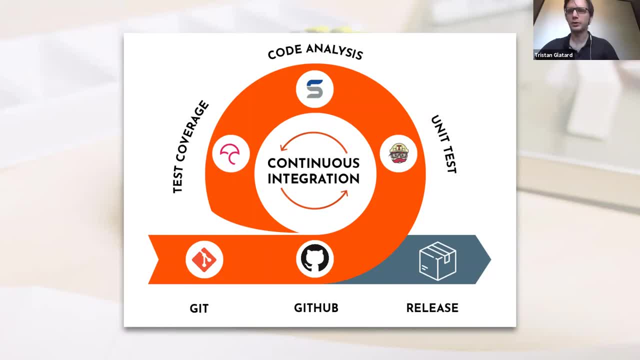 Uh, it's usually not good practice to put it in GitHub or in a Git repo. So how'd you do that? Where do you put the data? So that's a great question. So there's a bunch of solutions, So One that is very tightly coupled to GitHub um is actually get LFS. 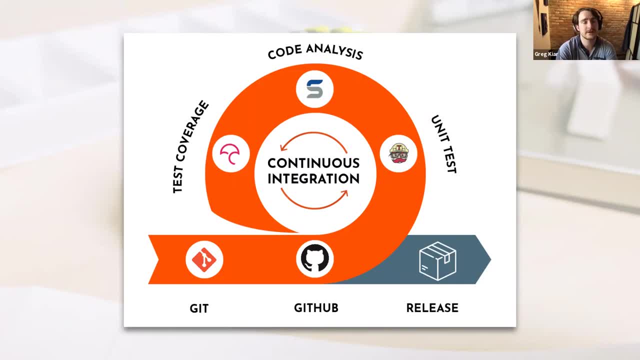 I don't know if anyone is familiar with that yet or has been introduced to it. Get LFS is get large file storage. Um, GitHub has, uh, by default, um, some plan for this that allows you to Like a hundred gigabytes of data on your free projects. 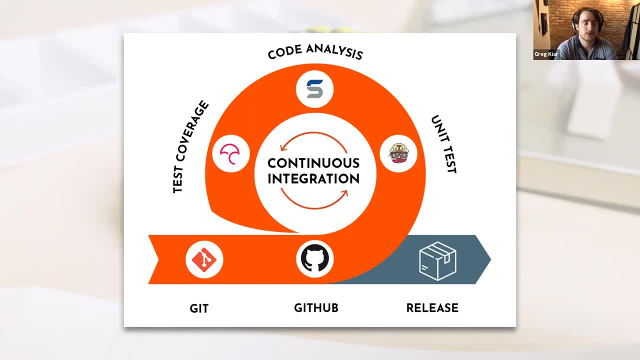 Um, so that's one option. Another thing is, you know platforms like Google drive or open science framework or really any public data repository, And then You можно usar como si es un sitio de aplicación, que se puede utilizar en cada sitio de aplicación. 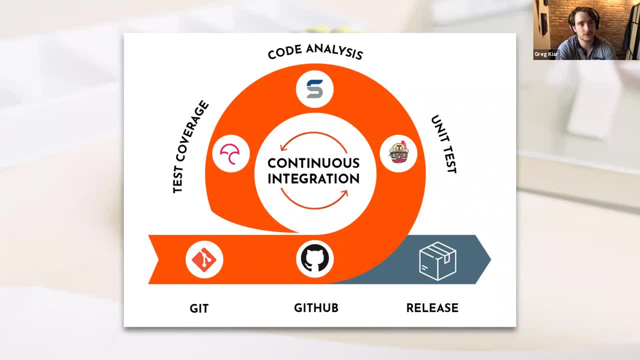 Uh, this is a tool called Travis. This is also part of your configuration in your um continuous integration suite. This is a tool called Travis That'll show you in a in a moment Um you can download your data and do whatever setup you need before testing your tool. 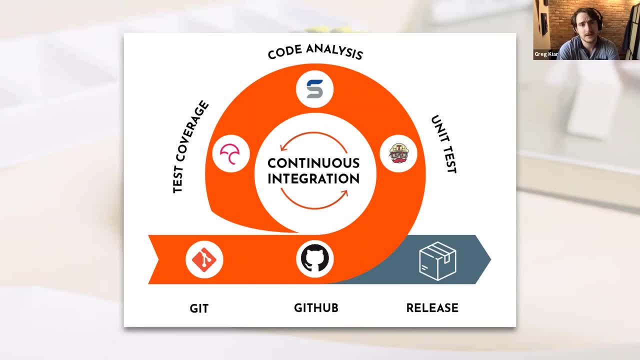 So there's different, like kind of what they call bill stages, And so again, what you can do is say, okay, great, I, you know my continuous integration, I'm going to get my new version of code, Great. 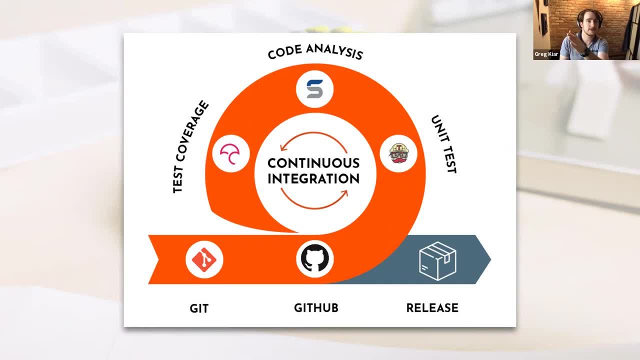 Once it installs successfully, download the data that I want to test it with. Once the download is done, then run my tests. If my tests are done, say congratulations and give yourself a pat on the back So you can set up these continuous integration suites to do all of this well, and you can. 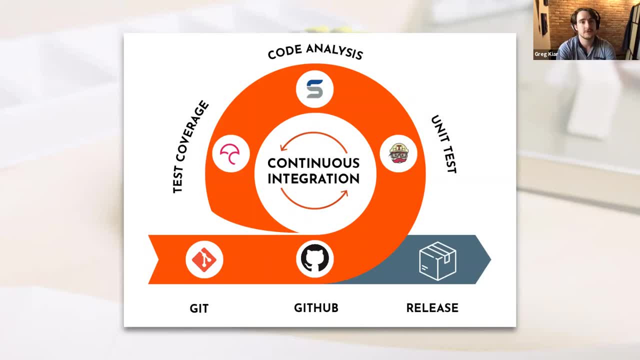 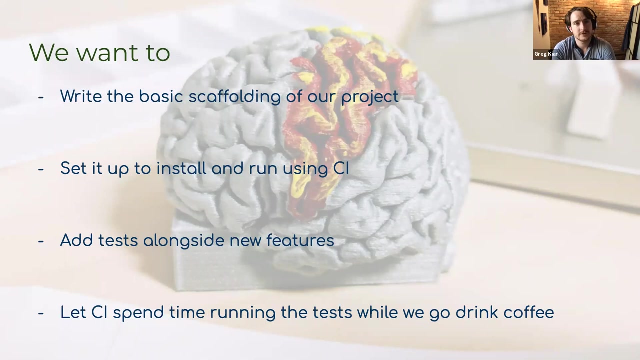 even make different steps run in parallel. So, for instance, you could download your data in one step and then run three parallel jobs after that that are testing it differently, for example. But yeah, that's a great question, Cool. So, basically, what we are going to do in terms of, or the way I'm going to what I'm going, 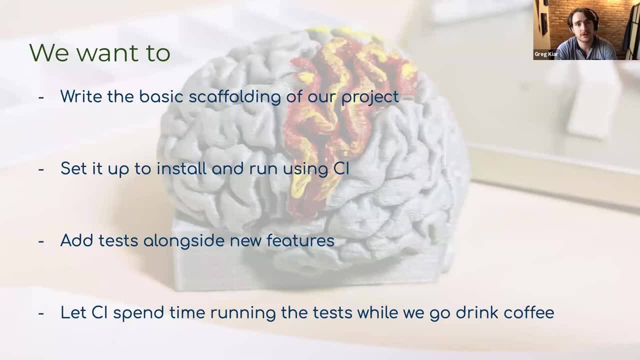 to advocate for? rather, in terms of tool development for our projects- and I know a lot of you are kind of making different tools, is that? in general, the way I try and develop is by making the scaffolding of a project, So basically the broad strokes. I approximately am going to have a layout, something like this: 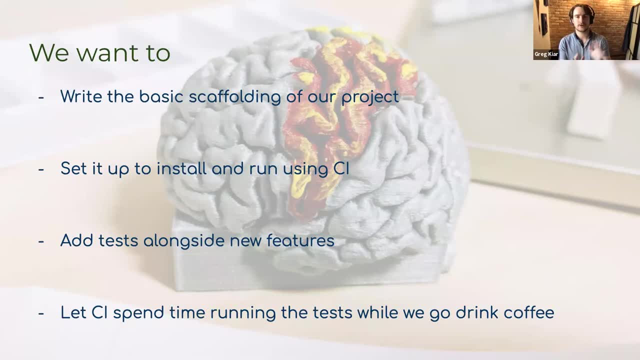 I'm going to have these, These types of functions. they're going to be, you know, working together in this way. And as soon as there's enough that it exists, I'm going to set up continuous integration immediately. And once we have continuous integration set up, every single time I add a new feature. 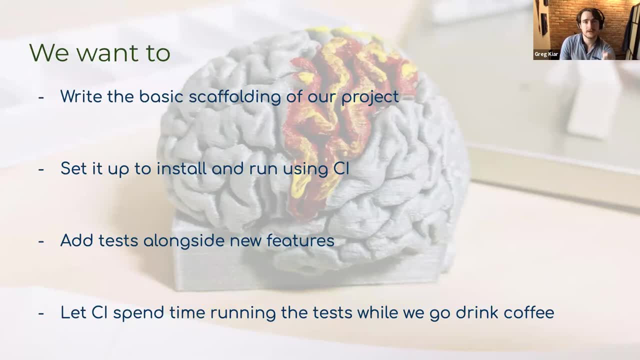 I am going to write a test for that feature And once my test is written for that feature I can push that to CI as well alongside my code, So I can do the same project And then make sure that every new feature as I'm developing it is working as I expect. 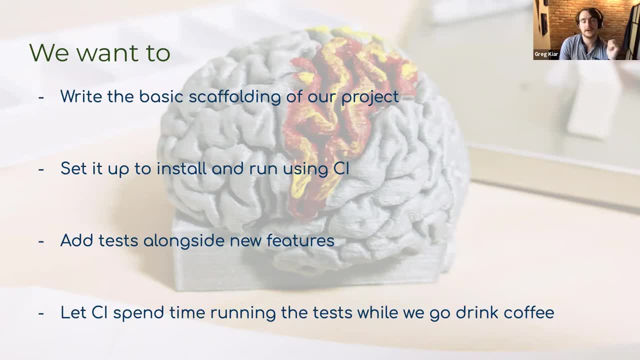 it to. So at least I have unit tests for every single feature as I go, And then it's much easier at the end of the day to add an integration test. And one thing, a phrase that you may have heard, is test-driven development. 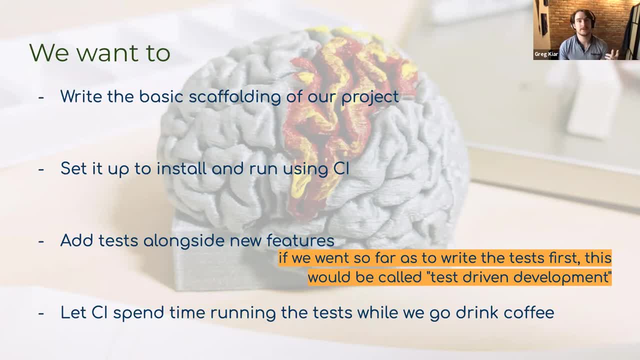 So if we went so far as to develop our tests before even developing our tools, that is what's called test-driven development, And this is a very common practice nowadays, Where, again, we simply say: you know what I have say a CSV file and I want to perform function X on that CSV file. 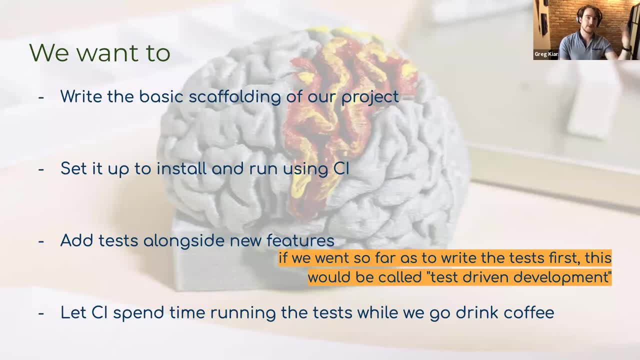 Well, I'm going to create a template CSV file. I'm going to call this stub of an application or a function that doesn't exist yet, And then I'm going to compare the expected results to what actually that function is returning, And then that's kind of a way that you almost set the goalposts in terms of when you're 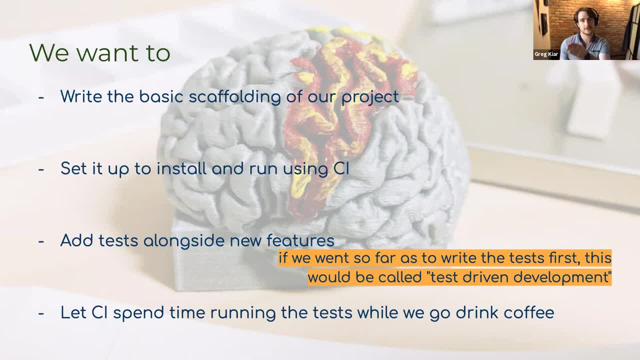 done. developing that feature: Yeah. So if you start by setting the test, if you start by saying this is what is required to pass, then you can develop with that goalpost in mind. So, again, this is test-driven development. It's a great practice. 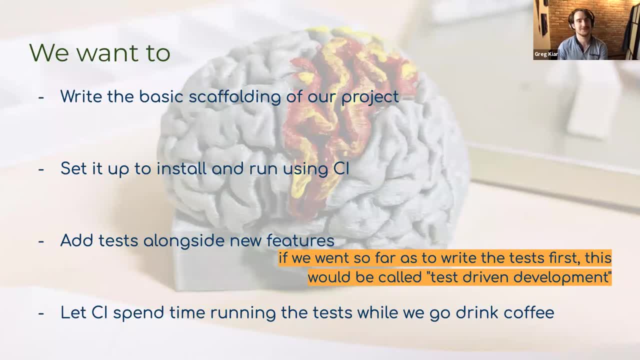 I think it's harder to keep yourself accountable on than would be ideal. I think it's. I don't think I've ever been fully effective at actually doing that. I think in general, I get too excited about the features I'm developing. 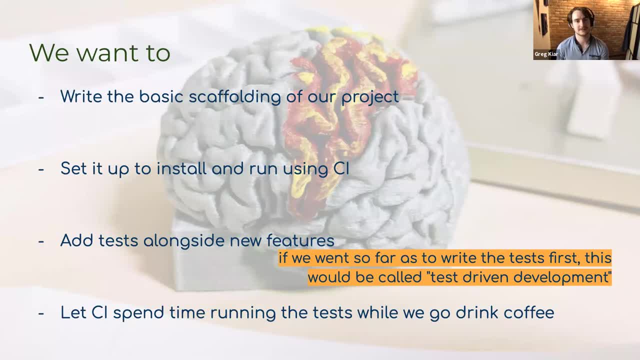 I develop them and then I go write tests later, And I think that that's probably not uncommon. Again, if you want to try and hold yourself to doing things like test-driven development, that would be wonderful. But just know that it's not just you if you're failing to actually follow through on that. 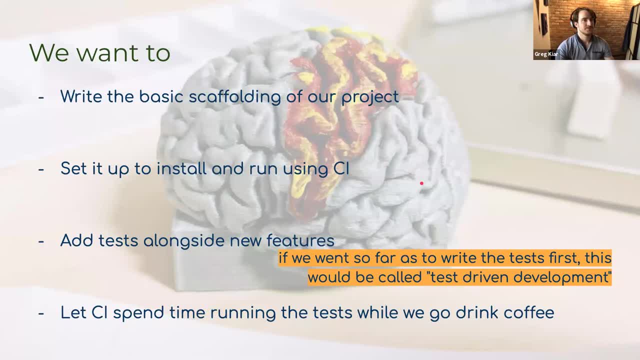 It's a hard thing to do. It's also the type of things that you can do throughout the project. I mean, even if you didn't start with test-driven development at some point you could say, you know, for the next three features I'm going to write tests first. 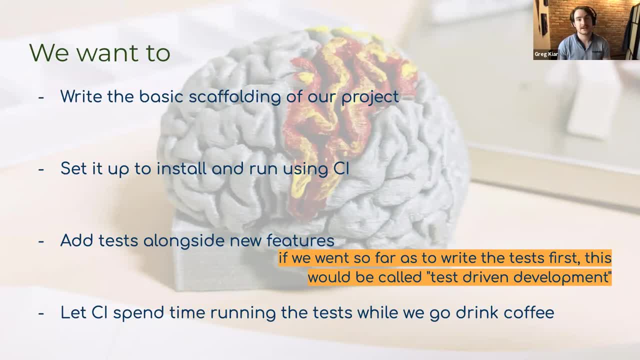 Absolutely, And then if you give up on it, it's totally fine. Exactly Right. There's no particular order. these things need to be done in because, at the end of the day, your code doesn't care when the test was written for it. 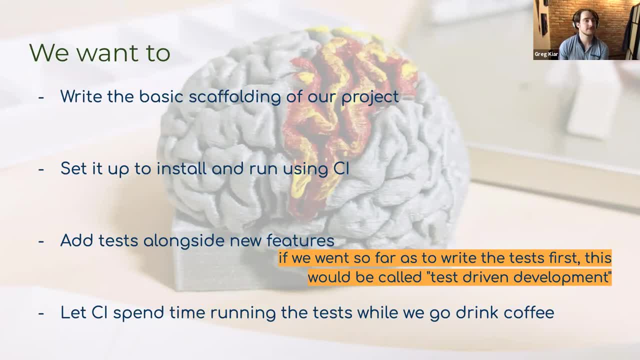 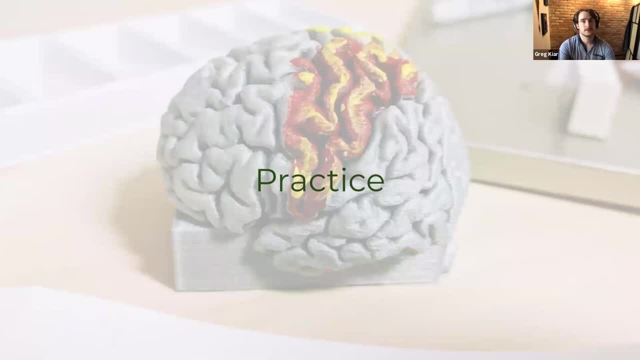 It just needs to have a test. So that's basically the idea. Again, this is just one particular order in which you could do that. So if anyone, I mean we can. I'll pause in a second, but I'll first tell you what we're. 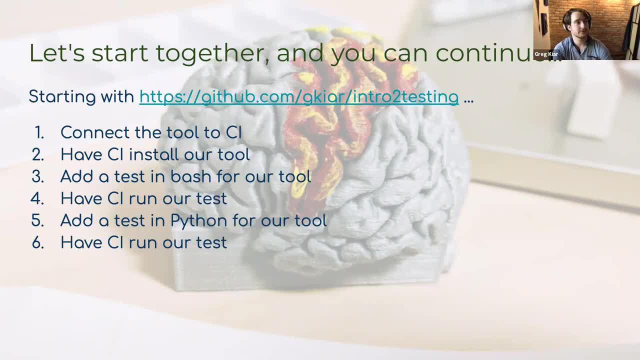 going to do, But if anyone has questions, feel free to start writing them. But basically what we're going to do is So we've created this kind of template repo that we'll go to in a second. We are going to set up continuous integration for this. 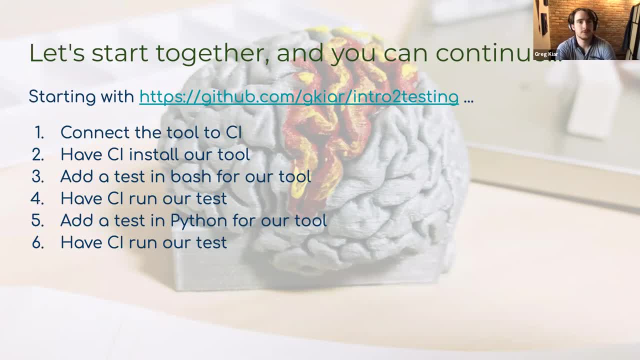 We are going to have it install our tool and its dependencies. We're going to write like a little bash script to test our tool, make sure it runs. We're going to make sure continuous integration is running that test. Then we're going to add another one in Python and make sure it's running that test. 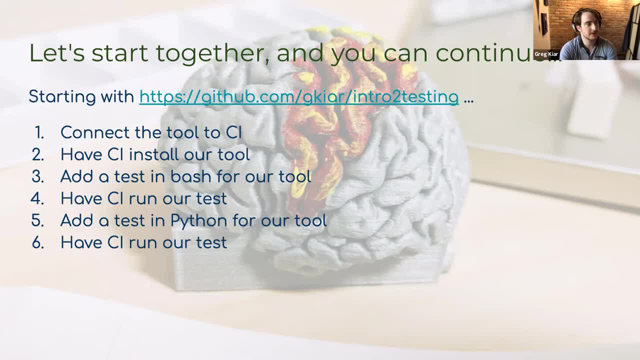 And as far as we get we'll be. you know, as far as we get, But let's get started. So the idea is just, we'll show you a couple of ways of how to set up CI using this platform and then a couple of possible ways of writing tests. 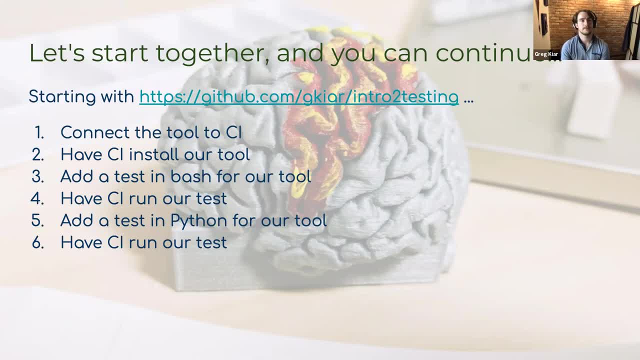 Because, again, at the end of the day, a test doesn't need to be anything other than a way that you are simply, you know, running a piece of your code in a way that you are providing some inputs, have an expected output. And again, what we talked about at the beginning, rather, is that this can be as simple as making. 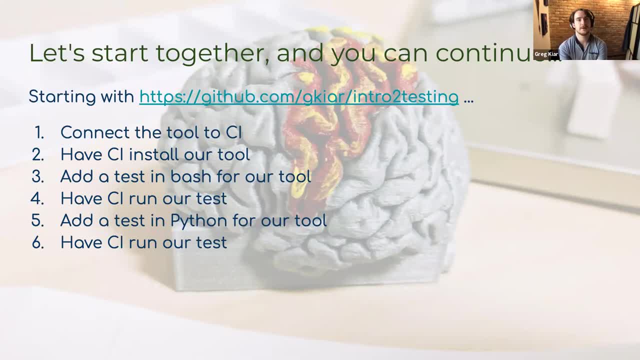 sure the tool doesn't crash in some cases, And this can be as complicated as expecting that a specific output is going to be running, And again, we talked about that at the beginning. rather, is that this can be as simple as making sure the tool doesn't crash in some cases, And this can be as complicated as expecting that. 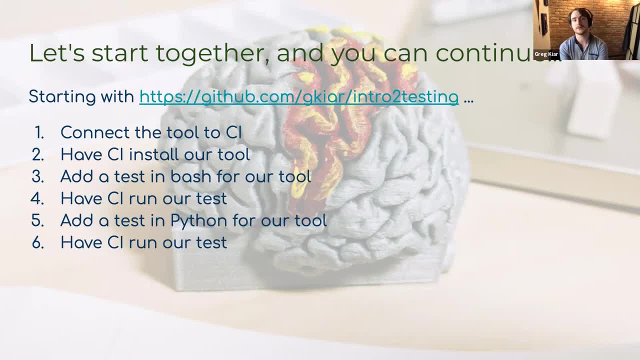 a specific value in a specific row or cell of a data frame or image is the value you want it to be. So there's going to be a huge gamut of things And again we'll try and write a couple of each category here. 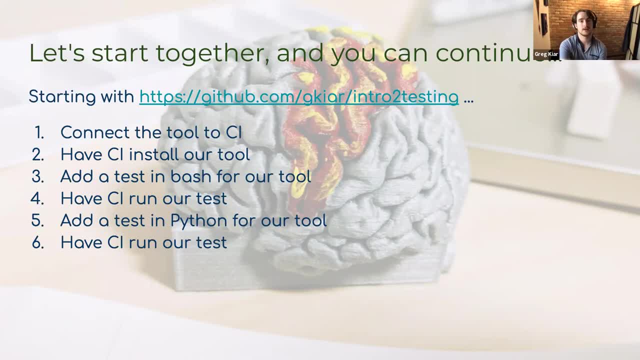 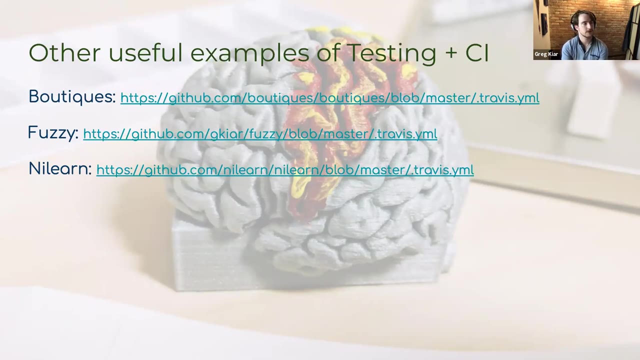 So does anyone have any questions before we get started on that? Cool, And again, as I promised, I'll link these slides so everyone has the link to it. But here are three different projects of different complexities in terms of their Travis. Travis is the continuous integration tool I mentioned. 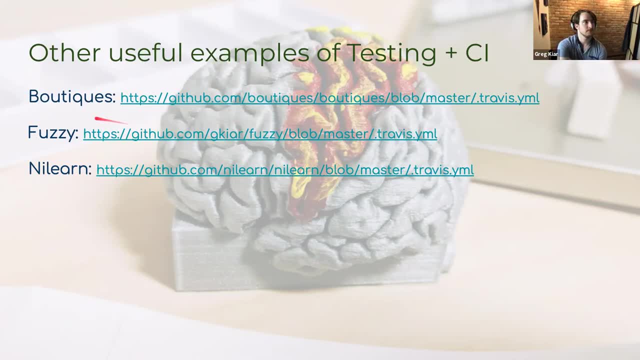 In terms of their configuration for continuous integration. Boutiques is a project of Tristan's and mine, and Fuzzy is a project also of ours, and Nylern you've all heard of, And they all have very different setups in terms of how they use the Travis, the continuous 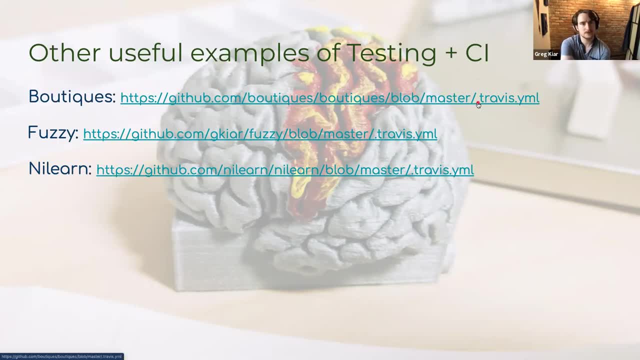 integration tools. I'd say that Boutiques is the simplest one In terms of how it's set up. Fuzzy has a lot of nice parallelization, and so does Nylern, But they both set up their parallelization stuff very differently. 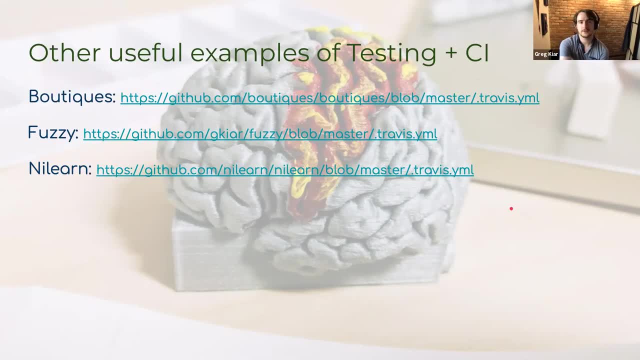 So these are just a few examples, And there's so many more And there's even other tools. There's another tool called CircleCI and there's one called AppVeyor. There's tons of them. So, again, what is important is- I'm not trying to pigeonhole you- to all use Travis. 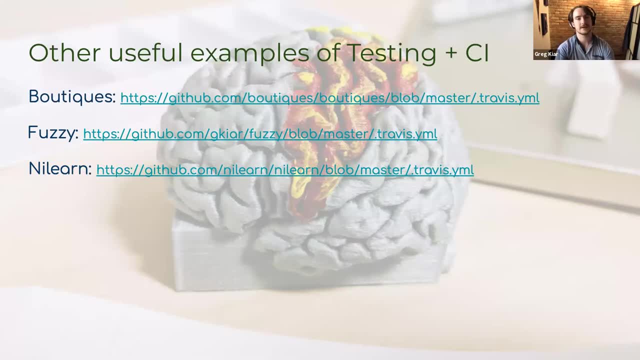 I think Travis is probably the lowest barrier to entry. It's the easiest CI to get started with. It's been around a while, And so that's why we're starting there. But this is really the concept is the most important thing here. 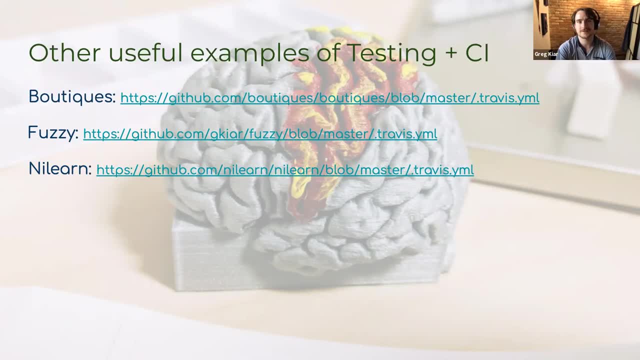 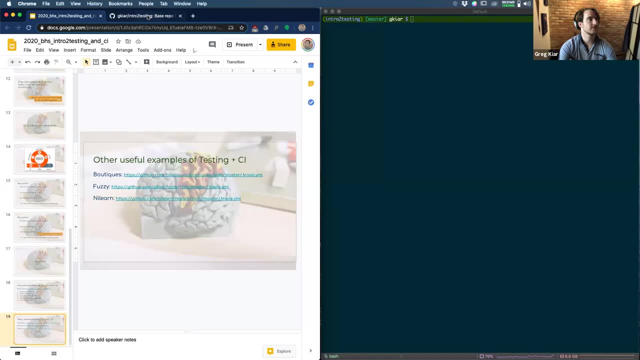 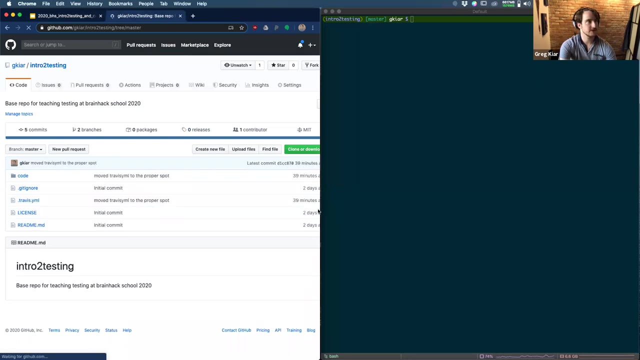 Don't ever worry about memorizing Travis's syntax or things like that, Cool. So unless people have questions, we should get started. Let's see if that, so you guys can still see my screen right. Yep, Yeah, Perfect. 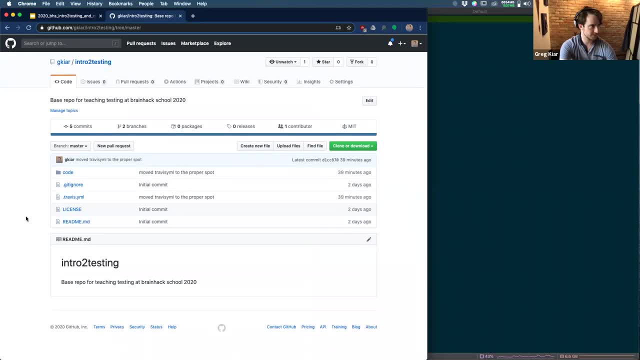 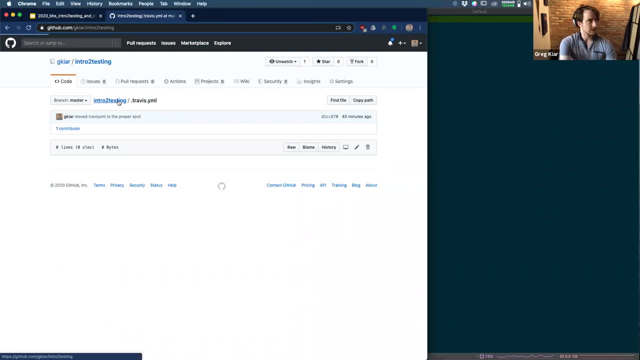 So this is the GitHub repository that I linked is where we'll start from. There's a little gitignore file, a Travis file, but there's actually nothing in it yet. Let's see the gitignore file. I picked just the Python one because my script happens to 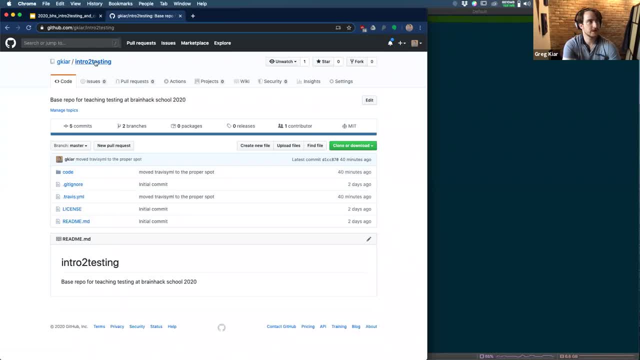 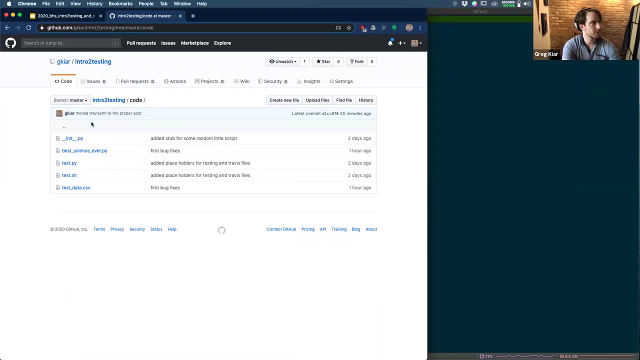 be Python- I'm not sure if you guys are familiar, but when creating a repository you can again pick like a default license, you can pick a default language for your tool and things like that Instant. So let's see. So inside this code folder we have a few things. 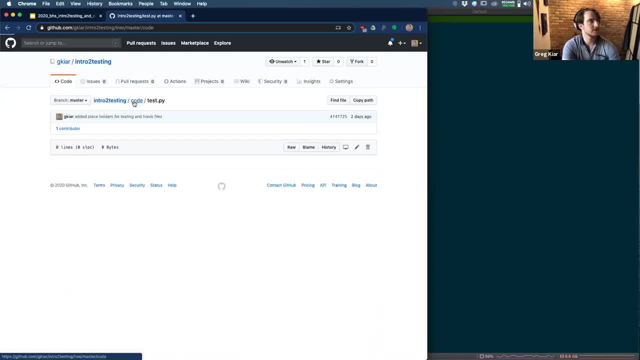 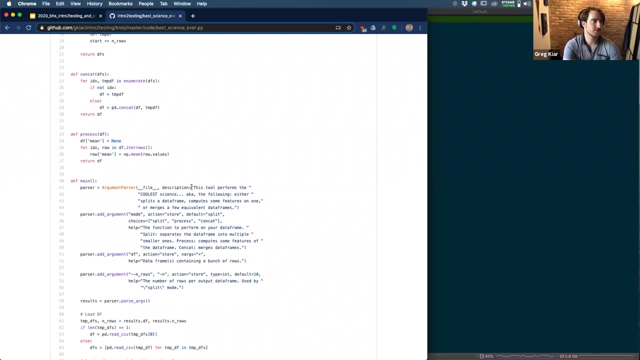 We have testpy, which is currently empty. We have testsh, which is currently empty. We have best-science-everpy, which is our amazing tool that we're going to write tests for. So the function of this tool, it is the coolest science ever. 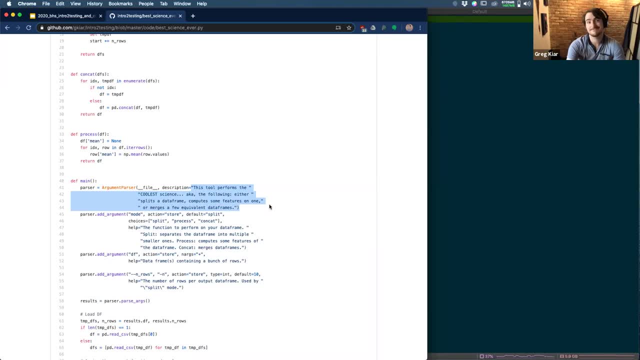 It splits a data frame, It will compute the mean on the column, Or it will merge a few data frames with the same columns. It's outstanding. No cooler science exists on the face of the Earth as far as I'm concerned. Of course I'm kidding. 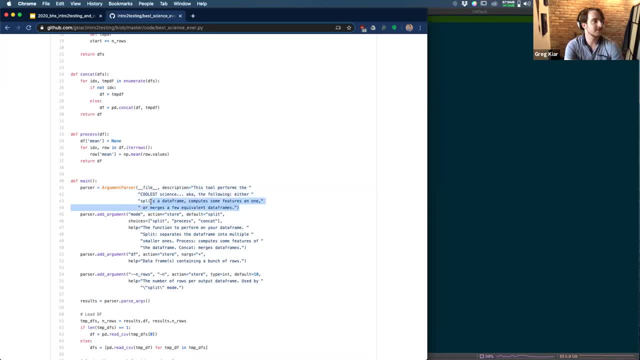 But I basically took this as an example of something that I needed to do recently. You may think: well, why is this a relevant thing? So an example of justification for why I tool like this needs to exist or could exist is—so, for instance, I have a few thousand graphs. 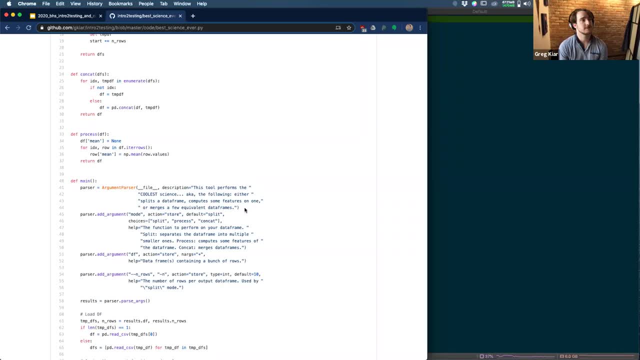 That's good. I need to know how many more graphs I need to learn to do this, graphs that I need to process. I need to compute a bunch of- you know- univariate and multivariate statistics on them. Some of those statistics take a long time to compute If I were to do them all. 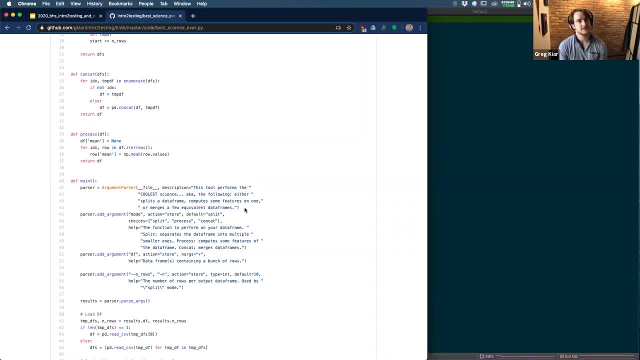 one after another, for you know my thousands of graphs. it would take me about a year. So what I do is I split my data frame into batches of 10, and then I have 400-ish data frames that are each 10 rows instead of 4,000, and then I run all of those in parallel. 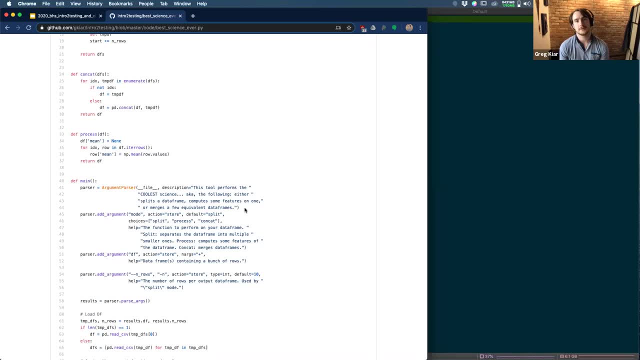 which takes much, much, much less time, and instead of waiting a year so I can continue my experiments, I'm waiting, you know, a few minutes. So that's just a bit of a justification as to why this super simple, seemingly useless tool has a scientific need. So what we're going? 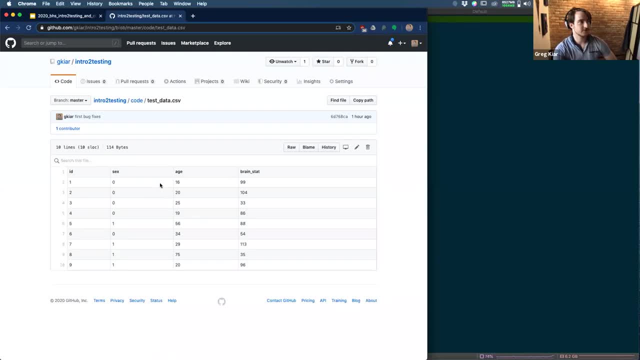 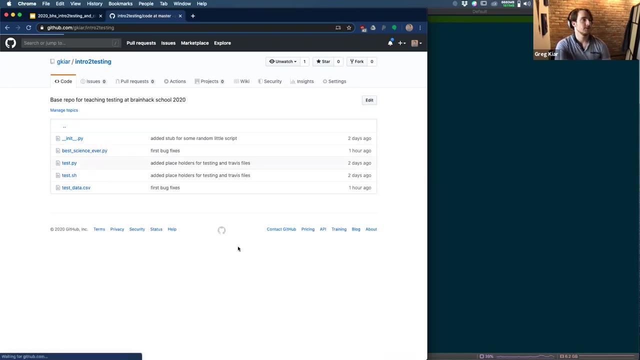 to do is with some- you know- test dataset, which is just some CSV that I made up a few minutes ago. we're going to go ahead and write some tests for it and set it up so that continuous integration continues to test it for us. So, and again, please continue to throughout this whole process. 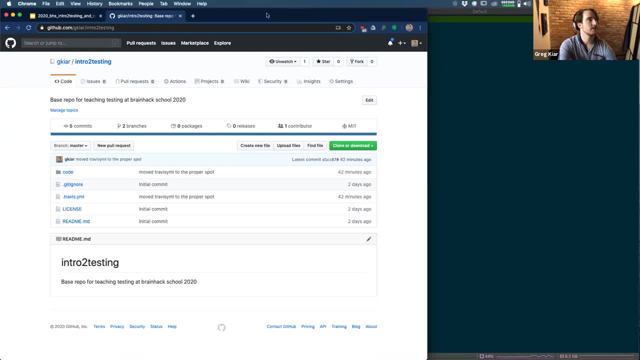 be, you know, writing questions in the chat window. Let's see if, now that I'm not in full screen, I can see the chat thing I can't seem to. I can find participants but can't seem to see the chat. Oh, there it is. There's behind the 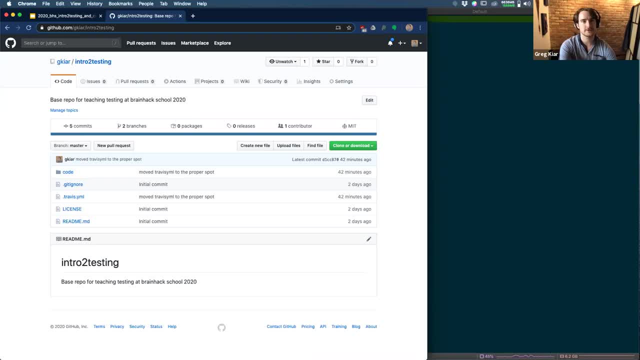 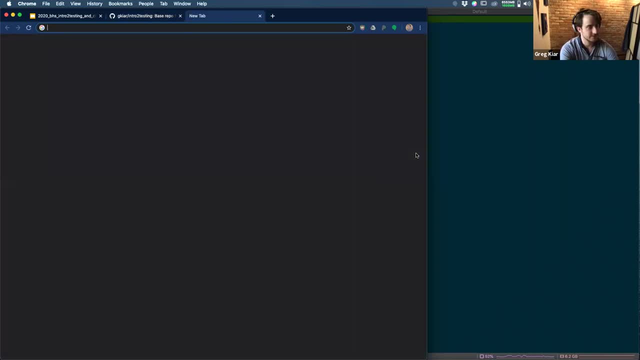 – found it. Never mind, I just don't know how to make computers work Cool. So what we're going to do is go to Travis thref, Travis Thri, Travis Travis, as I mentioned, is this great continuous. 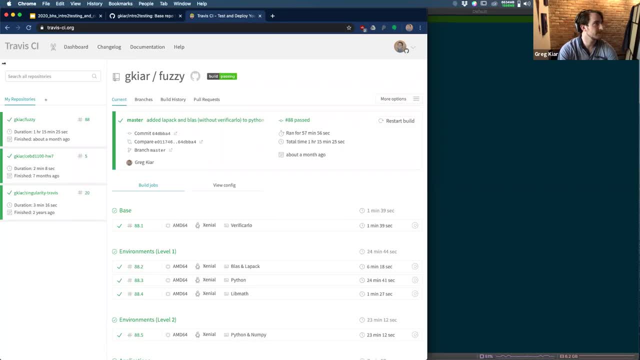 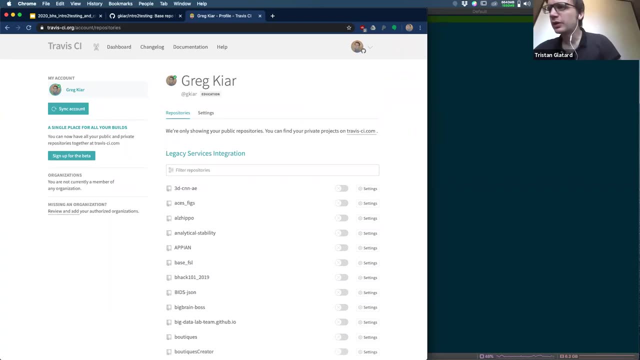 integration and I happen to be logged in, so it's telling me about some projects. You're going to go to Fuzzy, but what I'm going to do is I'm going to. –. Greg Isobel is asking if the link to the notebook is shared. 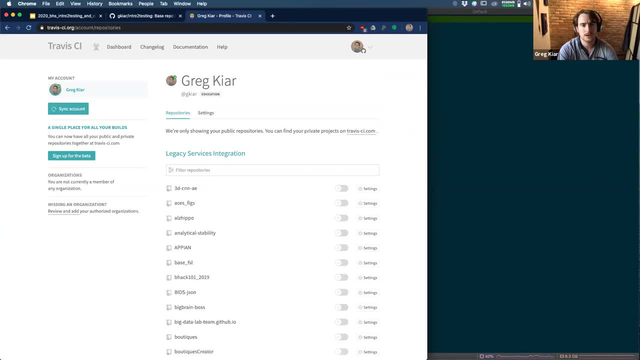 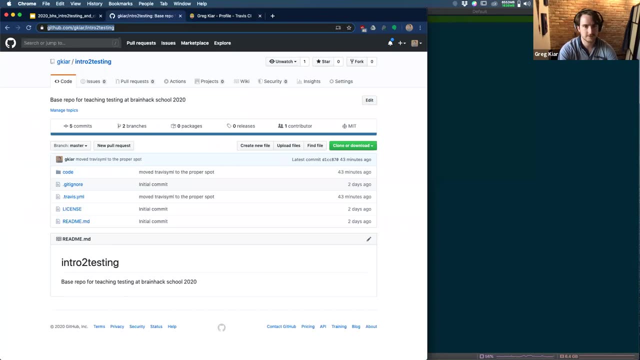 Notebook, I guess the GitHub repo. Sure, Oh right, of course the repo. I'll just post it in content right now and here, But it's in the slides as well. Thanks, No worries, Isobel, And then I'll also just quickly grab the link for the slides and share those in content too, in case anyone wants to. you know, check up on them while we're going through this. 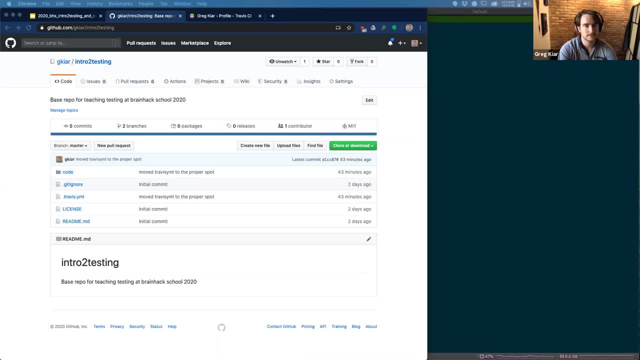 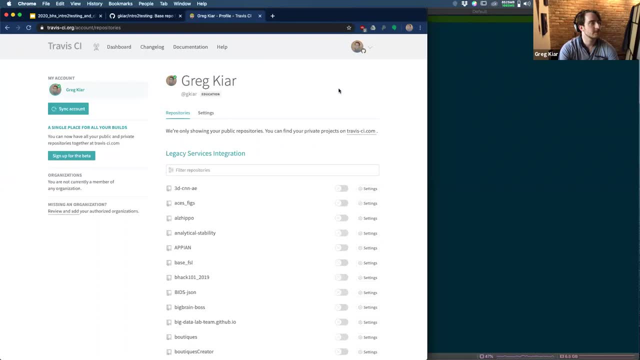 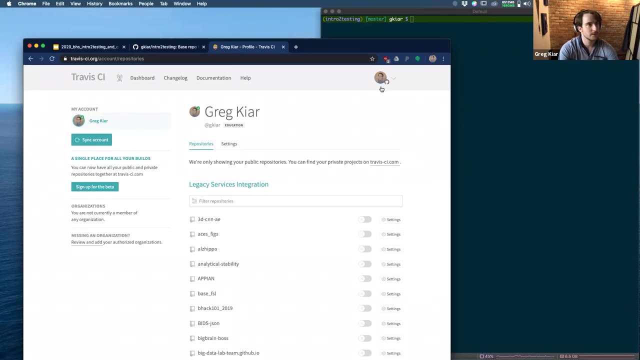 Cool, Sweet. Thanks for asking, Isobel, So what I'm going to do. so I mentioned that I went to travisciorg, Yeah, Travisciorg. Then I went to basically my little settings thing on the right. If you haven't logged in, you may need to log in. 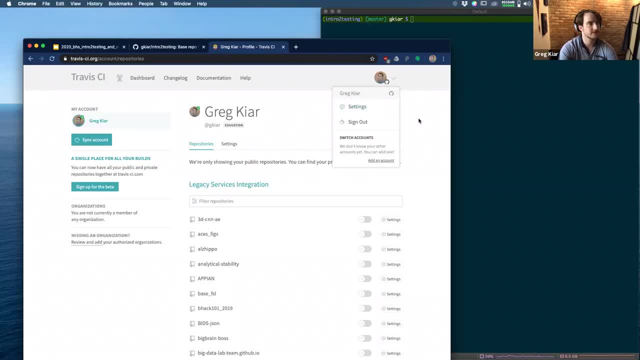 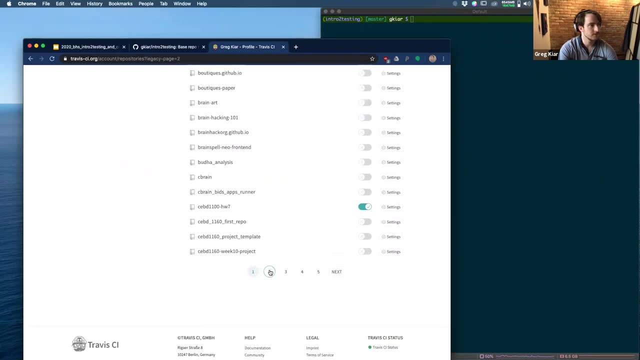 If you log in with GitHub it will automatically recognize different projects that you have. So then it shows a bunch of my repositories here So you can see where the check mark is on. some of those have continuous integration already set up and some don't. 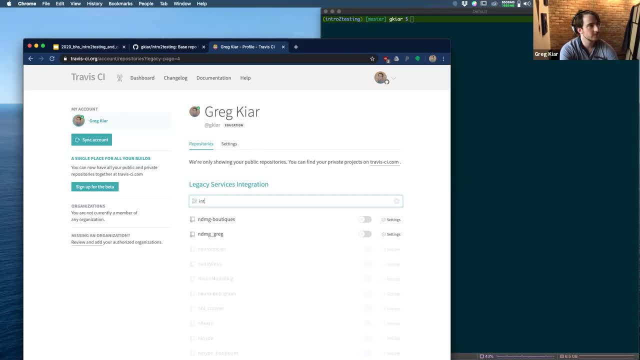 But you can actually, instead of scrolling through them, just search. So I think I called this intro to testing. Okay, Let's see. Hmm, But it doesn't seem to exist Repositories Sync account. Maybe I should do that. 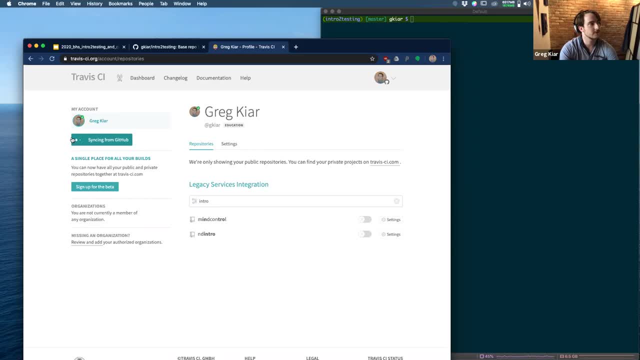 Syncing from GitHub. So I just pressed this again, this little button on the left, in case people can't see my mouse. It seems that maybe it didn't automatically recognize my repo And again, part of the reason why I'm going through this and I didn't have it, you know, already set up is just so you guys can understand that the process is. you know it's not going to work. 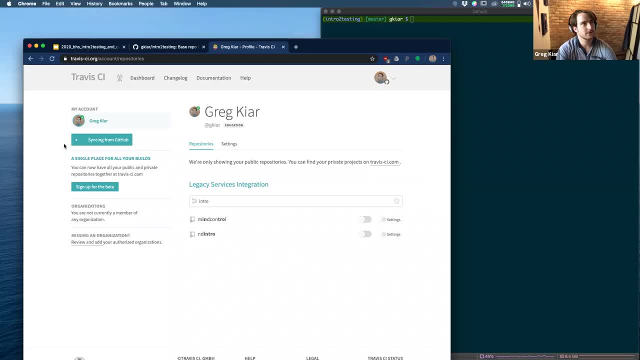 It's just a matter of finding, you know, the right buttons. So I think it's more valuable for you to see how I struggle and solve the problems than to just see something magically finished in front of you and be expected to get there. 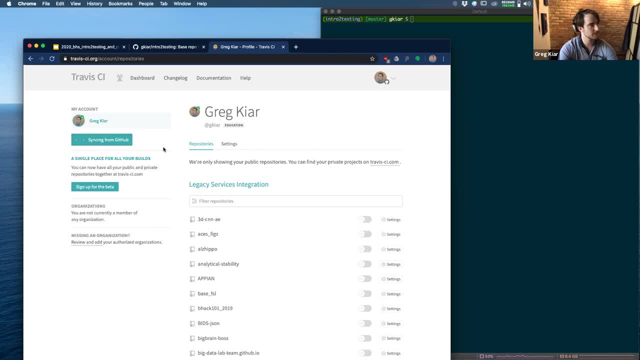 So let's see Syncing. It's taking a while. Maybe I'll refresh the page and break it. Let's see if it wants to show up now Intro. It doesn't want to show up, That's fun, Okay. 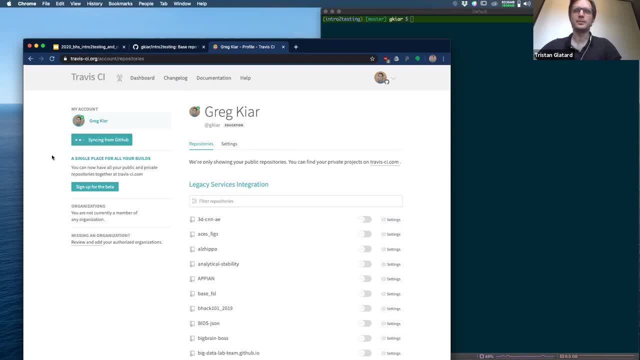 So Try to sync again. I've had similar issues recently. Yeah, You could also go to the com version, So Travis CI. one thing that I'll note while this is happening is: so there's travisciorg, which is like the free version. 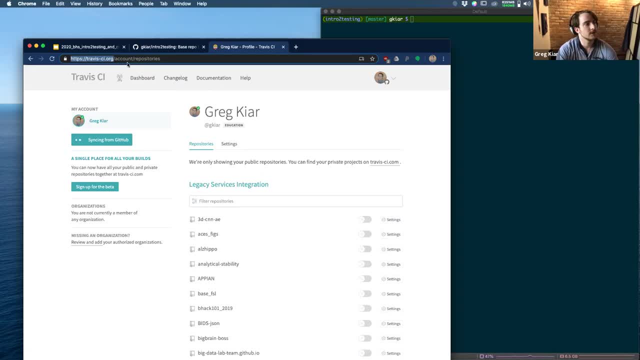 And then traviscicom is the like corporate version. They have some more features. They have better support for things that are like private projects. It's basically the same service just plus plus And sometimes again depending on the nature of your projects. if you have a private repository you'd like to test, you need to use the com one. 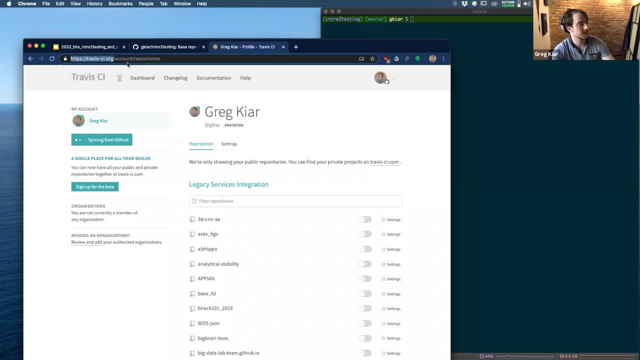 So it might just be again kind of bugging for some reason. Maybe they're, I don't know, making an update. Who knows How did you resolve the issues in the past, Tristan, with it not syncing quickly, Just waiting? 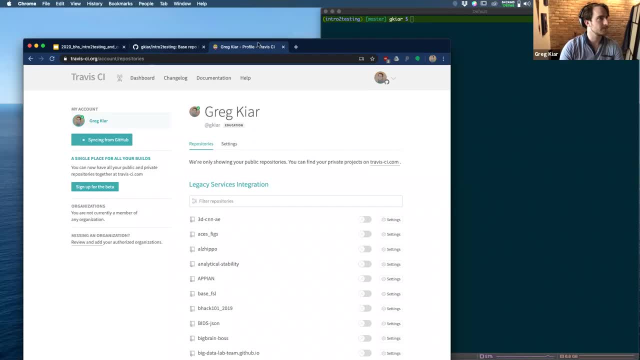 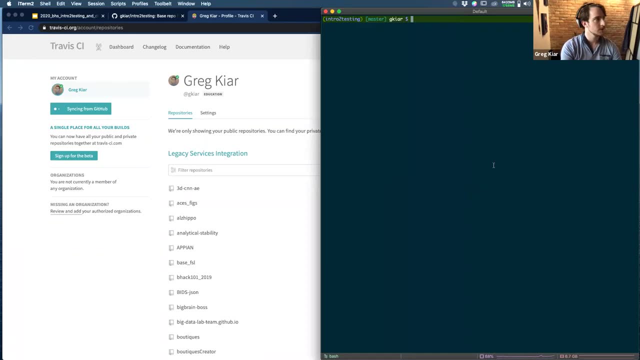 Okay, Just waiting, Cool, Sweet. So then I guess we'll go. while we're doing that, we'll start thinking about testing. So I'll leave this tab open and I'll go to my terminal. So this is just a cloned version of my repository. 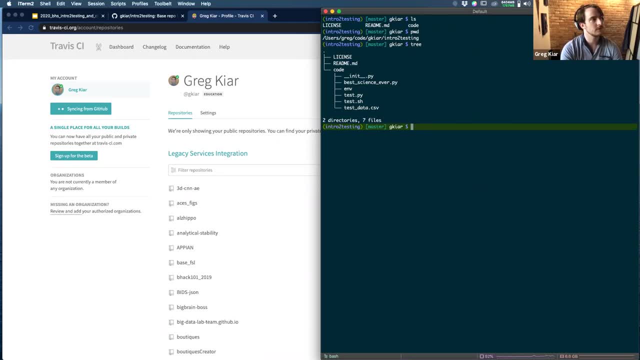 You know it has all the files there that I mentioned. So what we're going to do is actually I didn't mean to have an environment folder inside there. So what we're going to do is go and look at our code, Our tool. 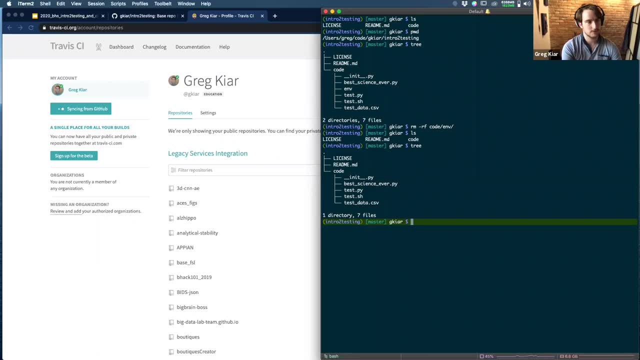 Well, actually, before running our tool, one thing that I know you guys have been introduced to well, both with Tristan yesterday from the perspective of containers, but, I believe, earlier with introduction to Python, is virtual environments. So what I'm going to do is I'm going to make an environment. 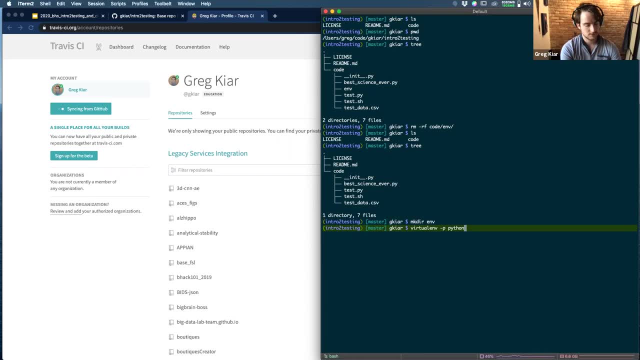 I'm going to use a tool called virtualenv, Make a Python 3 environment, Put it inside my env folder and call this Introduction Intro to testing seems like a reasonable name for my environment, And that way any tool that I need to install for this project will be in this one little. 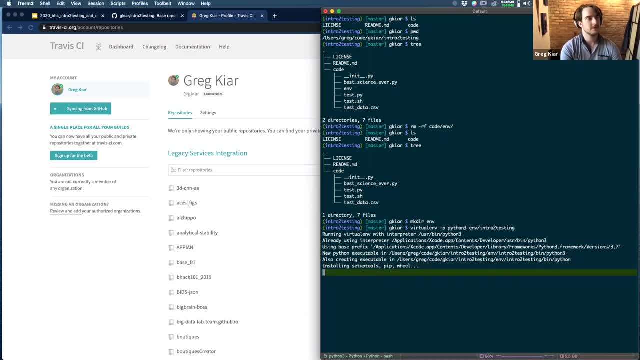 spot that's isolated from the rest of my Python installations, And that way, if I have versions that are conflicting with one another or other things like that, this is isolated from all of that. So I'm going to environment, And now we see this little red text bit on the side here. 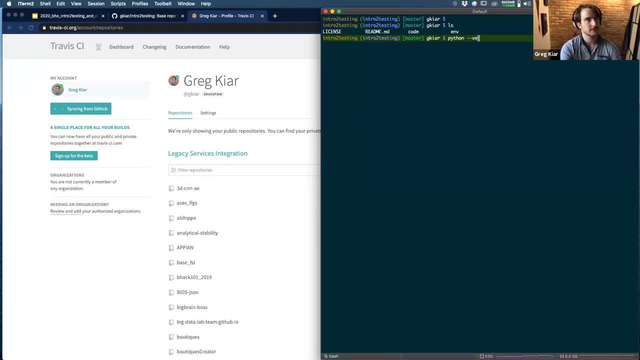 Cool. So now I'm going to just make sure you know I am using, indeed, Python 3.. Yep, Great, So I'm going to go inside my code folder Again. this is where our best science ever- Python script- is. 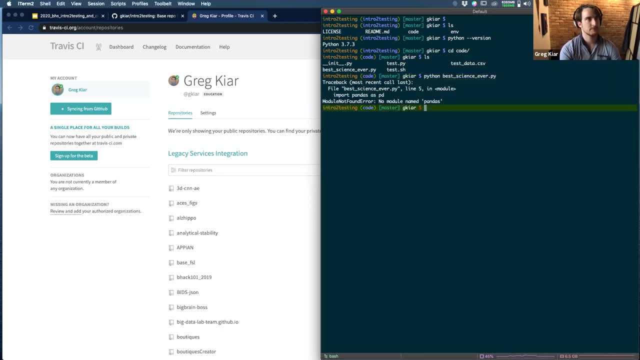 Best science everpy. And I'm going to run it and say: uh-oh, there's no module named pandas, So let's install pandas. I'm sure I'll get an error again, unless this installs another dependency, Because I also need numpy, I remember. 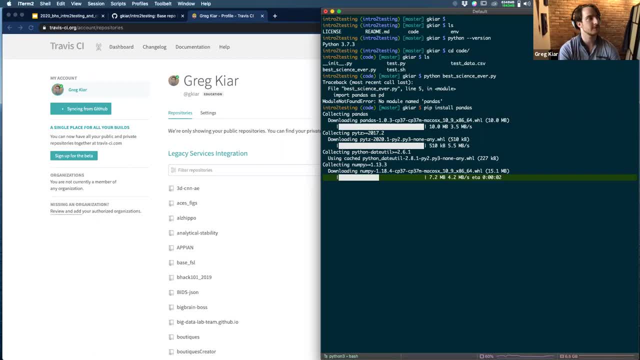 We'll see if pandas- oh, there we go, Pandas- is installing numpy for us, So we should be fine now. Okay, So now that we've done this, I mean, one thing we talked about was installation testing. So installation testing, you know, of course, is making sure that our tool can be run. 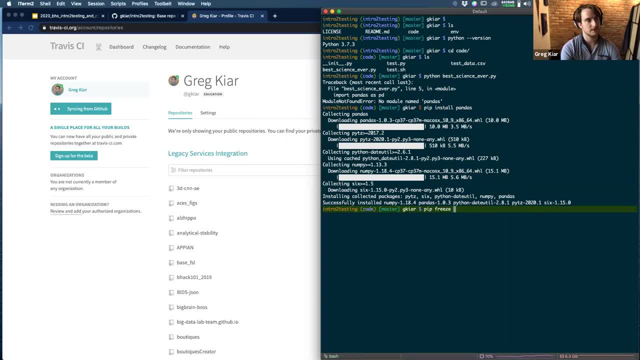 So let's see. So a way to get a sense of if our or what dependencies our tool needs is. I'm not sure if you guys have been introduced to the pip freeze command before, But what this shows you is everything that's installed in your current Python environment, the versions of them, and so on. 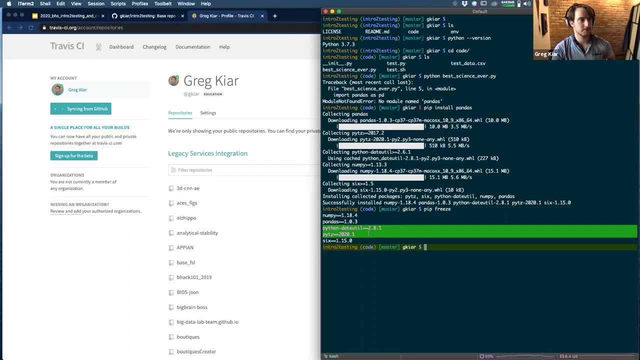 So in this case, you know, we don't really care about the version of date, util, PyTZ or six. These are all just dependencies of pandas. We'll let pandas resolve its own dependencies, But what we know is that we need or that our tool works. 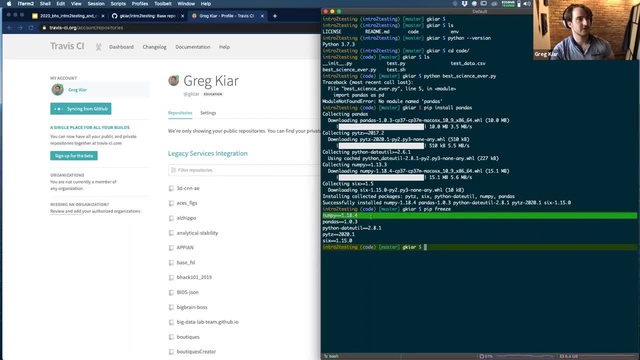 Or well, ostensibly should work with a version of numpy- that's this- and a version of pandas- that's this, And those two should hopefully be compatible with one another, Because, well, that version of pandas installed that version of numpy. So what we can do now is try our tool again. 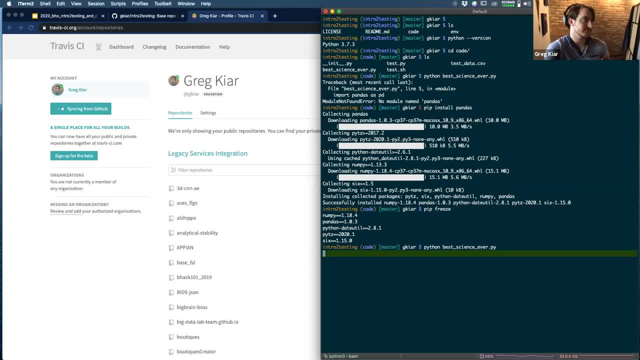 See best science ever. Let's see what happens. Taken a while, Aha, Error. The following arguments are required, So I'm just going to, you know, plug this in Print. a bit of help text to make our lives a little easier. 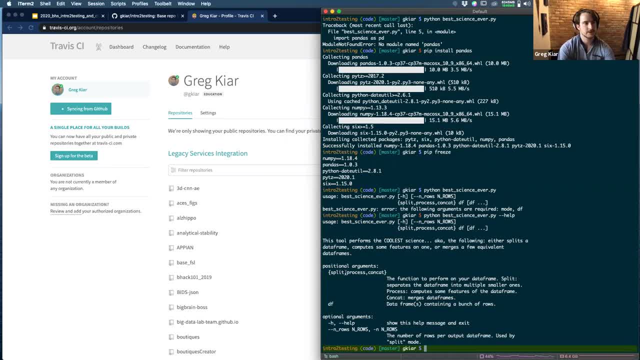 So there's a few modes here. So again, as I mentioned, we can either split our data frames, We can process them, which literally means taking the mean, Or we can concatenate them back together. And if we're splitting them, we have this optional extra argument, that is, how many rows we want per data frame. 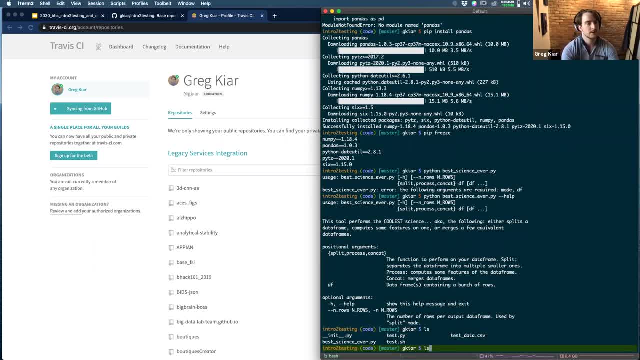 Sweet. So what I'm going to do is say: Python, best science ever. We want to do a split now because we have a single data frame, And let's just see what happens if we put in test data CSV. Okay, What happened? 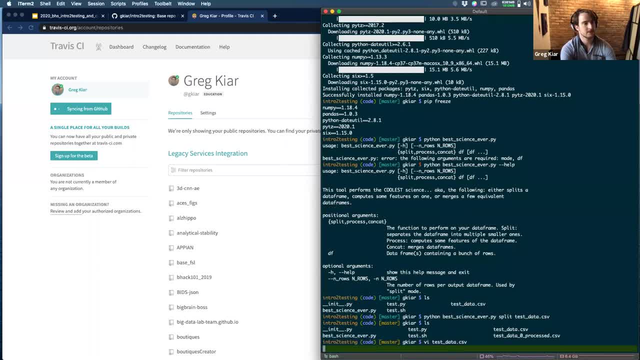 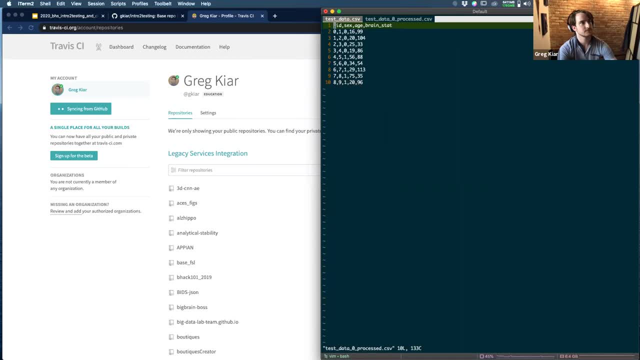 So let's, we're going to look at two things here We're going to look at. We're going to look at both our data frames, Okay, So first of all, I didn't provide an argument for One second. I'm just opening a second terminal there. 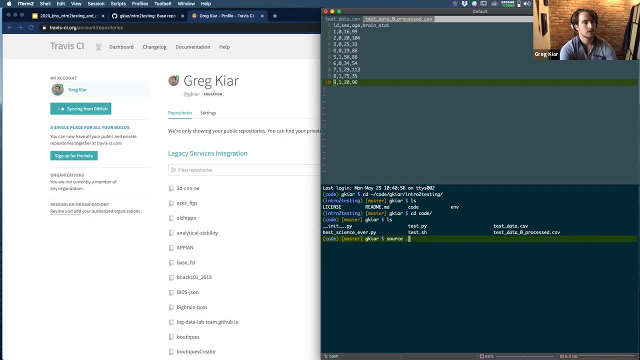 Cool. So we didn't provide an argument for the number of rows, So let's see Again what was our default for the number of rows. Let's see if our help text will show that for us. Oh, it doesn't. 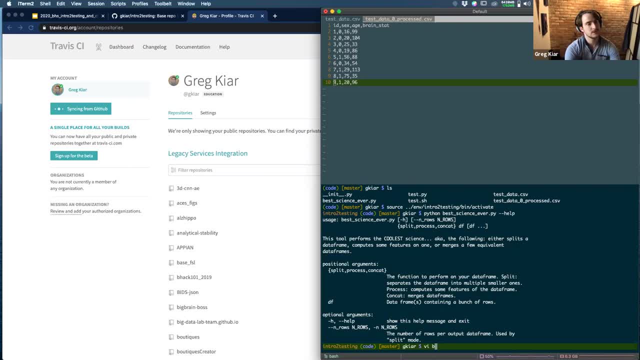 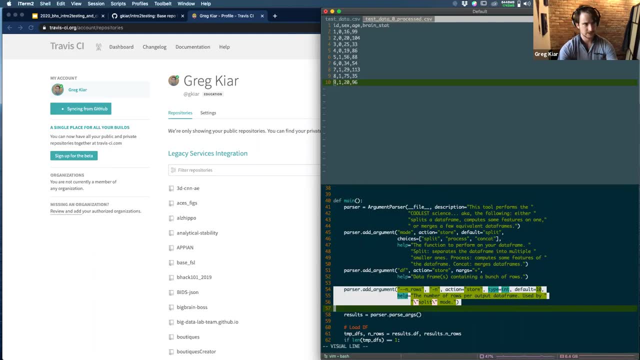 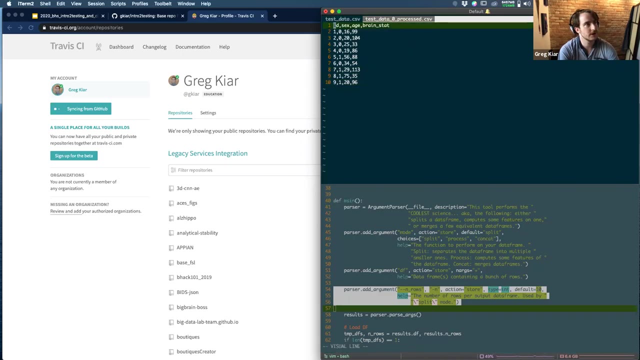 Okay, So maybe we need to look inside our file. The default number of rows is 10.. It's evidenced by this chunk. So what we did? here We have a data frame that appears to be, you know, nine lines long. 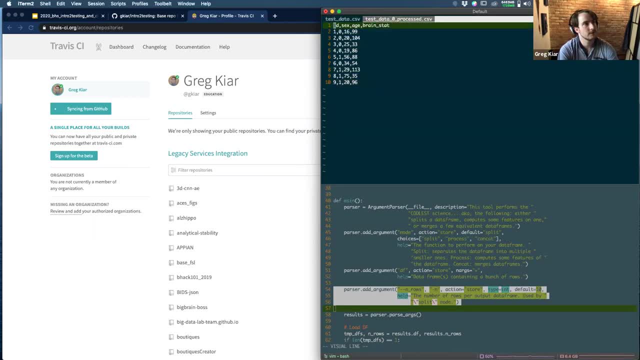 We split it, and Well, I didn't actually do anything useful, Because our entire data set is, You know, in here, And it also didn't give us the same Data frame out, because, as I'm just flicking back between these, as you notice, 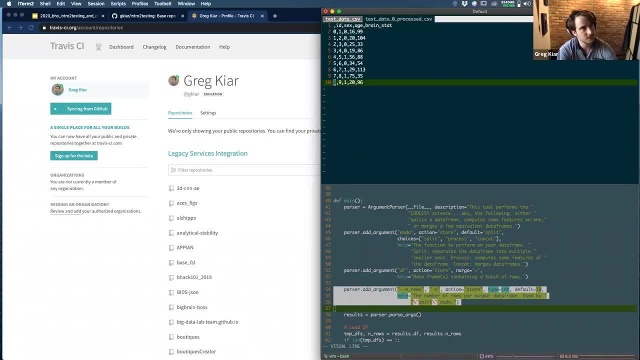 There's an extra column here on our left. So If we just had written a test that says: okay test, The tool runs, You know. to completion we could just say: you know, in our, in our little bash test. 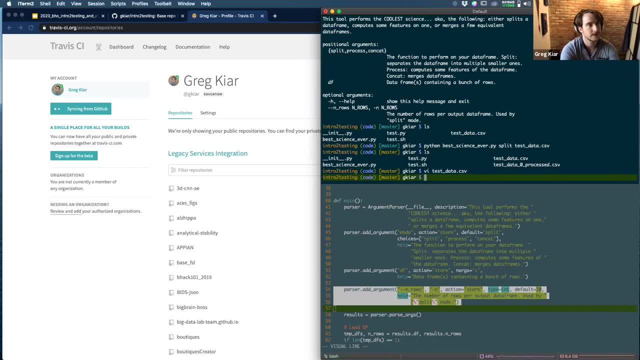 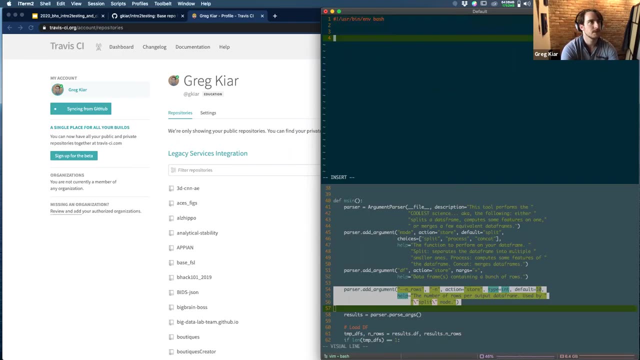 Whoops, There we go In our little test Sh. We could literally just copy paste This line And technically our tool would Pass this test. but what? everyone agree that our tool is doing exactly what we want in this case. 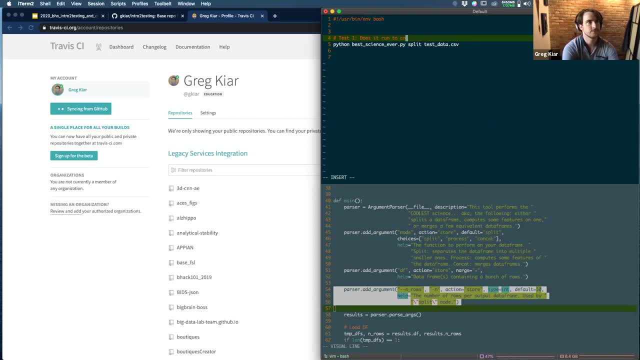 I mean, I I feel like that's the type of rhetorical question that works better in a live audience, But but I think we could all say no. So So so far This test is passing, but we agree that we aren't exactly getting what we want. 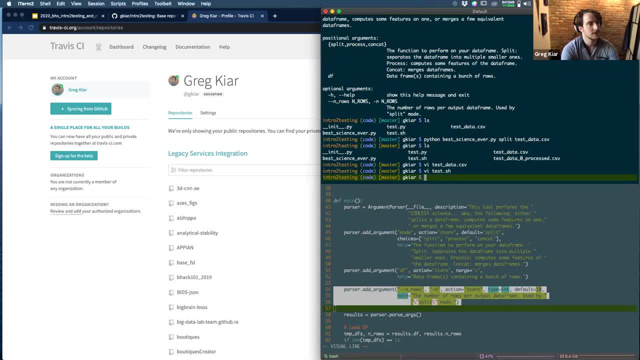 So let's think of a better test. So We know that, based on the way our tools currently written, The output of our Our Command wouldn't run like this. We'll be a new CSV file that looks like that. Maybe what we can do is look at the difference between those two. 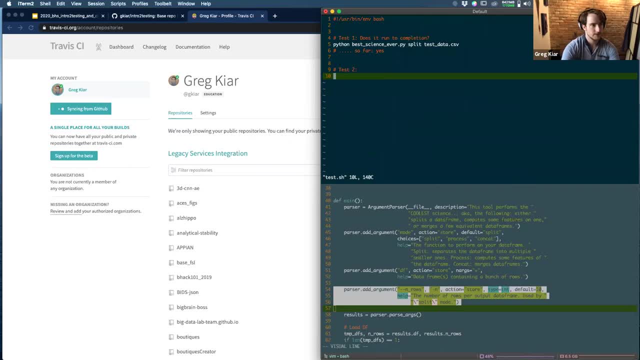 Right. So we can say: you know, in a perfect world, In a perfect world, Splitting with 10 rows greater than our original data frame, the input and output would be identical, And I think does everyone agree on that, hopefully. 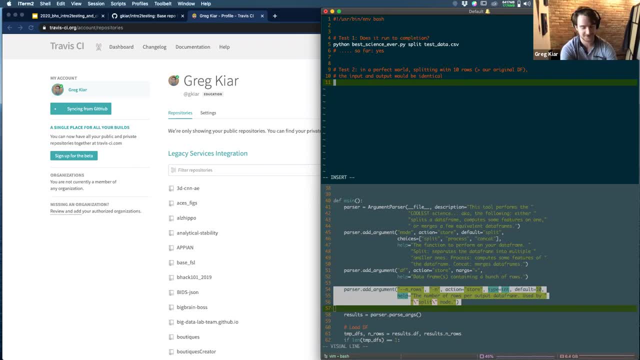 Yeah, Again, this is the type of rhetorical question that is better in a live audience, because I can see heads nodding, Apologies. So what I'm going to do is then try and run the same test And then, basically, what I'm going to do is ask: test diff- testdatacsv and the testdata process versioncsv. 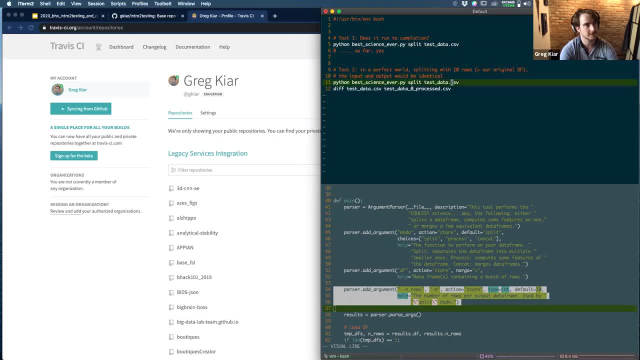 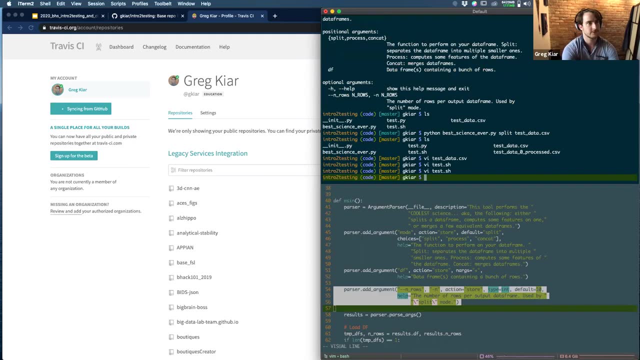 Although I actually don't need to rerun this because I'm just running the same thing, So I can actually run kind of two tests for the price of one execution. So I'm just going to do this. So now let's try and run this little test script. 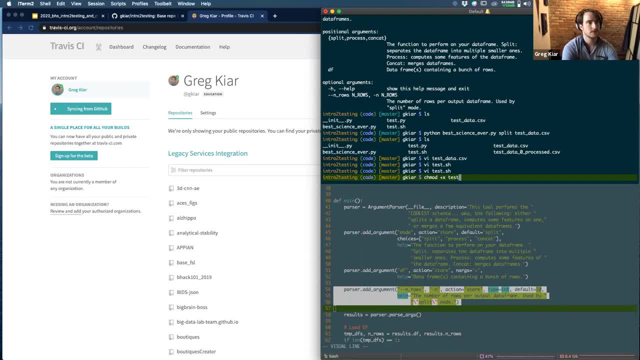 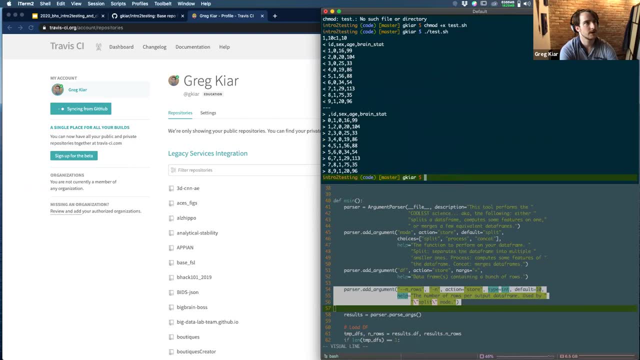 So I'm just going to make it Executable. Oh, whoops, There we go, And I'm going to write testsh. Aha, So this is not nothing. One thing that you know, one thing that this test was able to show us, is that, while our tool ran successfully, it wasn't, you know, giving us the result we wanted. 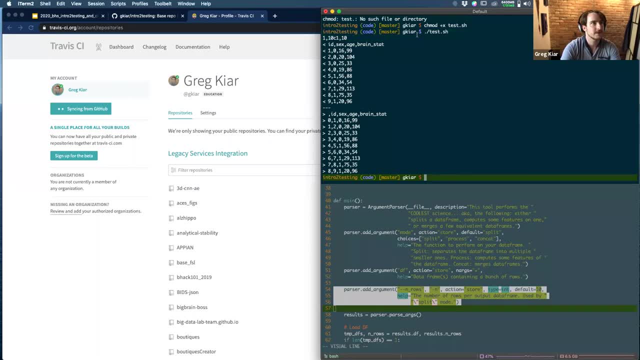 So Extended This device- kind of professionals actually did So. now A little word of the Word 04 or something like this: Does anyone notice something funny about my terminal between this line right here And this line right here? That's different about them. 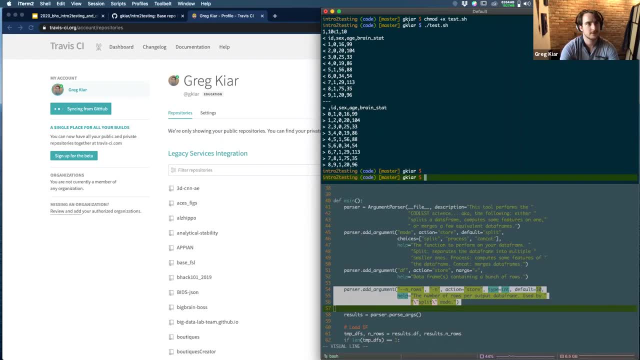 I'll press Enter once So you can see them more clearly. You can again type this or say this: It doesn't matter, There's a subtle difference between my, the way I've got my prompts set up here, my prompts out there. the color of the dollar sign. 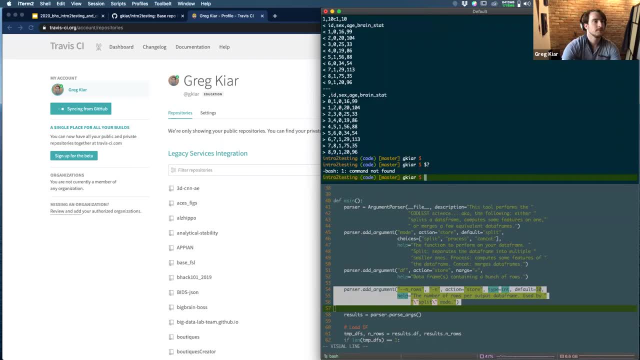 So Basically this is a little confused. So the you can see that it's here. I was using it. It was not in the rest of my code. Have you guys been introduced to exit codes yet Again, any yes or no in the 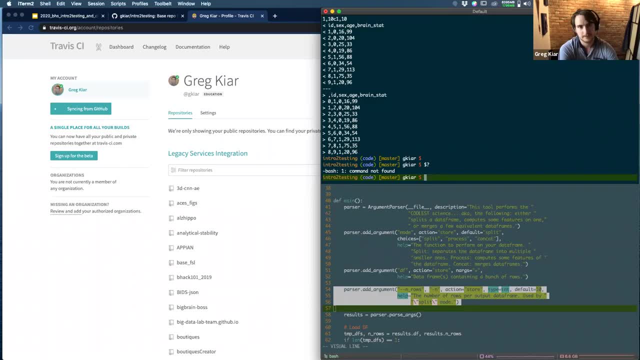 Okay, perfect. So every time a command in Linux- or pretty well every system, I think- runs, at its termination there will be some status. It will basically say: Yes, I ran properly, Don't worry about it, Or it'll say: No, I didn't run properly. 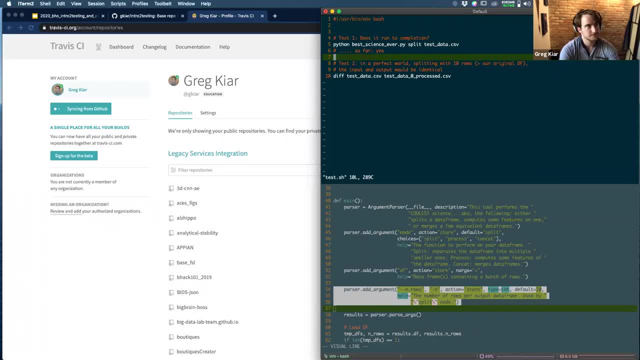 And this is conveyed through the exit code. So what I'm actually first going to do is I'm going to comment out this line and we're going to just run this test. So I'm going to do this again. It ran our test. 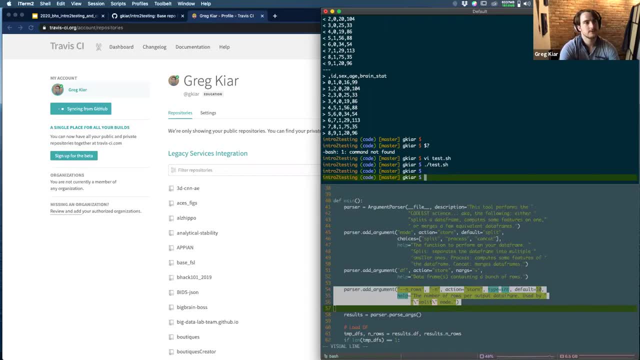 Voila. So in this case, the dollar sign stayed purple. The way I just happened to have my computer set up is that if the previous command errored, it gave an exit code that wasn't the one that everyone agrees is. everything ran fine, which is the number zero. 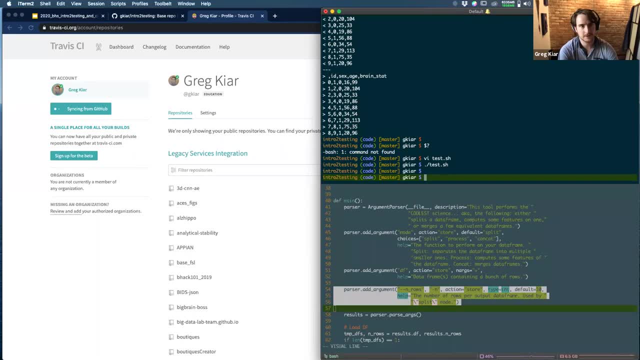 It will make the dollar sign a different color for me, just so that I notice that something failed. So what we're actually going to do is make our testing a little bit smarter, and we're going to have our script recognize that for us. 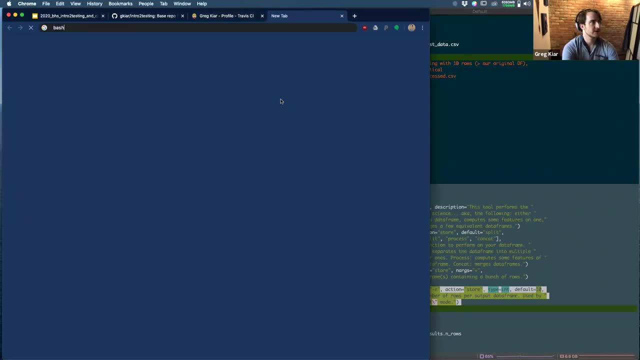 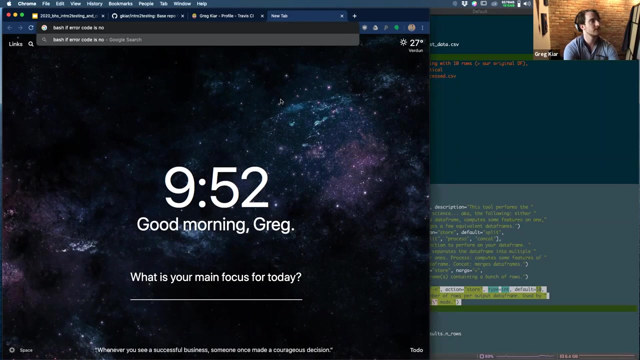 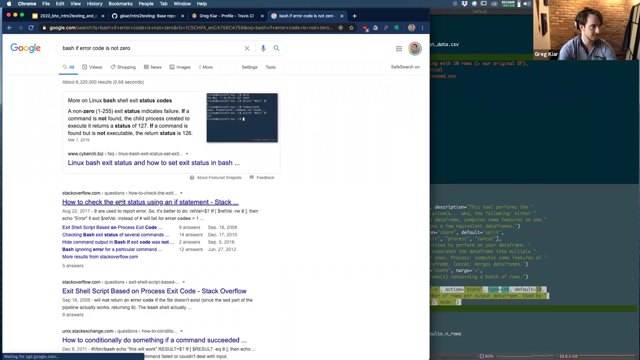 So here let's see How do we do that bash. look at, My keyboard is lagging. Look at error code. Well, actually I'm going to say look at If error code is not zero. So again, as I mentioned, there's always an error code. The universal value for everything's okay is to return zero. 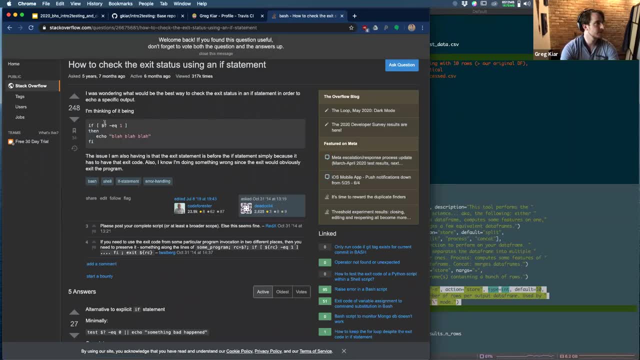 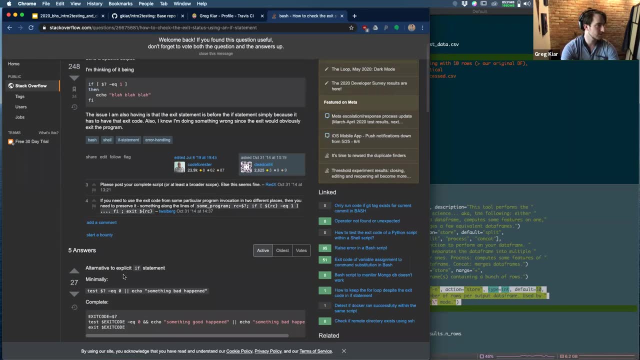 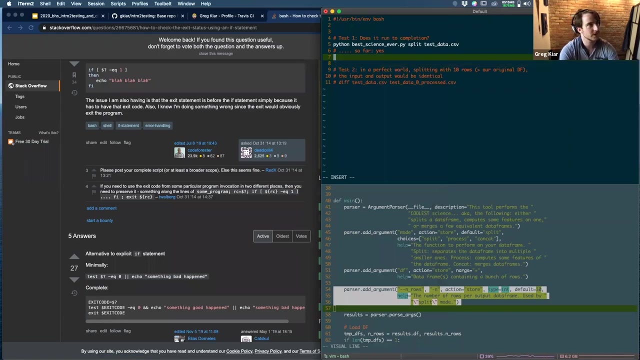 So let's see: Check the exit status using an if statement. if dollar sign question mark is is equal to one, So what I can say is: test if this is equal to zero, Otherwise something happened. This seems fine. So again, this is. I'm deliberately doing this on Stack Overflow and live in front of you guys so that you don't think there's any magic here. 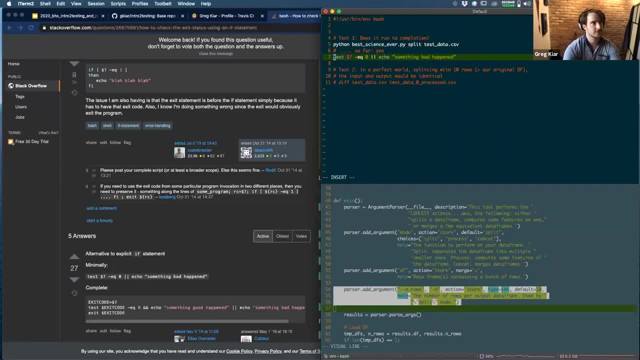 This is just like some idiosyncrasies of you know bash. There's many different ways we can do this. If you don't know the syntax, that's fine. It's just a matter of knowing how to learn it. 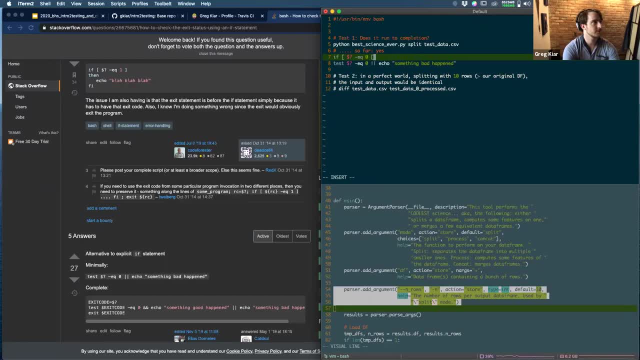 So if this is a сов form of, I want to do that and then. So if this is like I'm actually going to do is copy the other command from bracket, then And so people, I'm going to push all these changes as I do them. um, just so that anybody 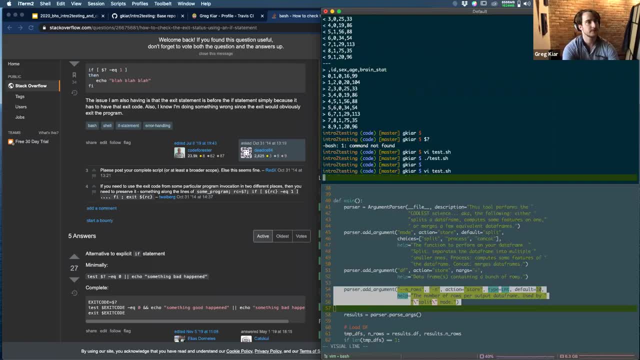 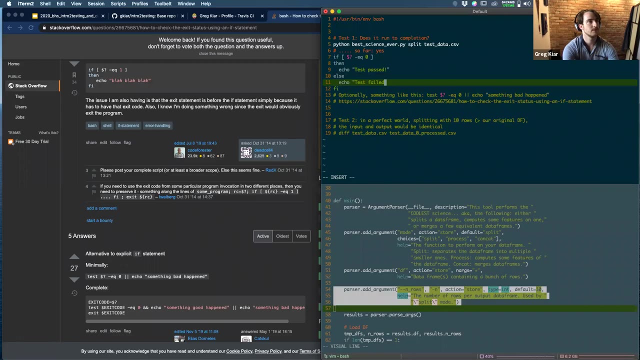 can see, uh, what happened or how we got there before, So I'll test this out. I'm going to do this here. Test passed, Woo hoo. So now what I could probably do is something like: uh, test failed as well. 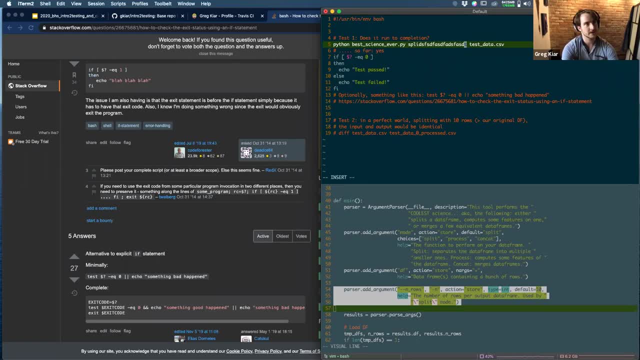 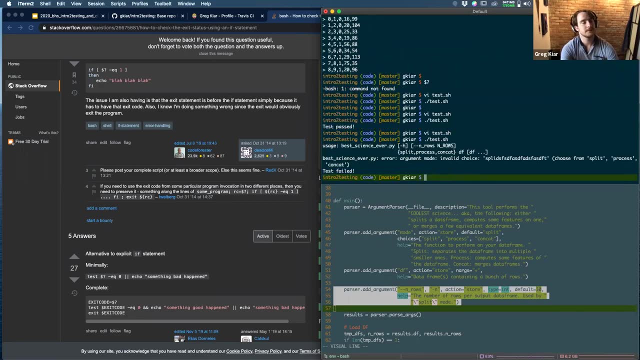 And now I'm going to just make this a garbage command by adding a bunch of garbage characters. We know that that spelling of split is not valid. Um and voila, it ran some stuff, it printed some things to the terminal and we got told: 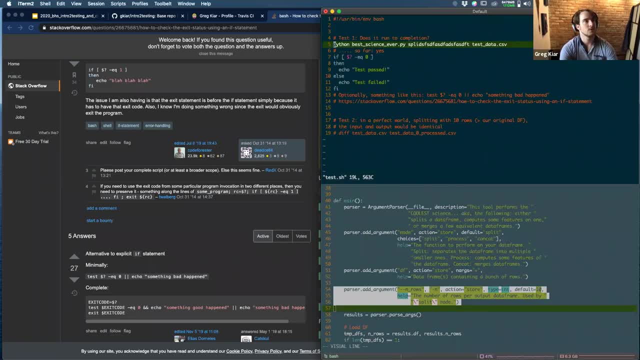 the test failed, Cool, So let's see. All right. So here we're now writing a test where we're running something On this line, here, line five, And then we are saying, well, based on the exit status of this, did it pass or did it? 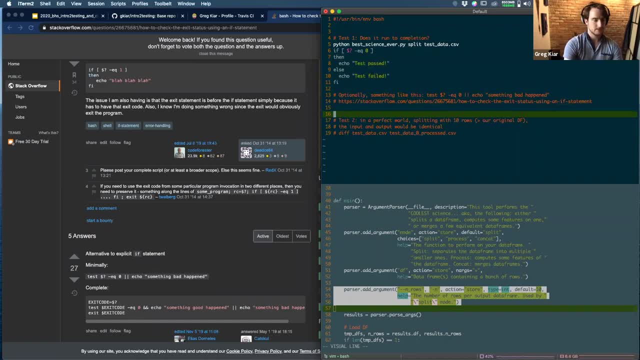 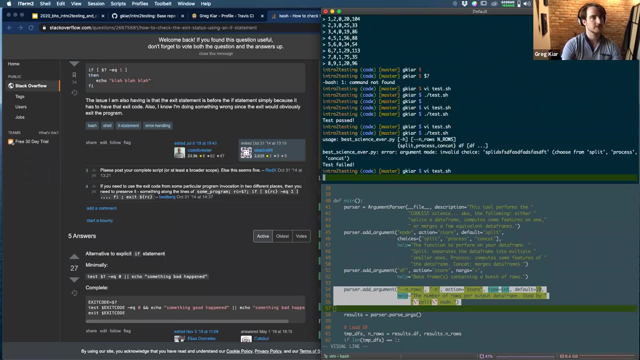 fail Um. so now again we can uh color in this test. again we can. you know, there's, of course, more efficient ways to do this, but we can just put our little um pass fail check there and we can see about both our tests. 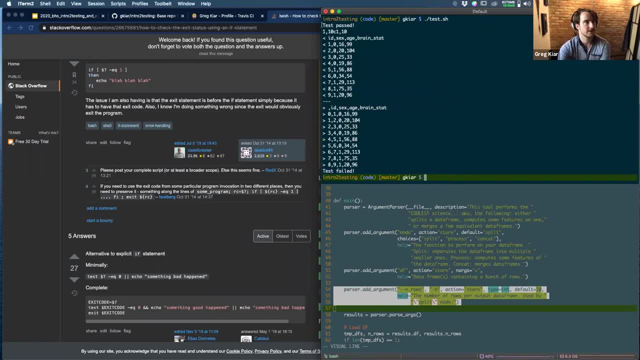 Of course this can be more descriptive, um with, uh, you know, putting like test one past, test two failed, and so on and so forth. But what we see is our first thing passed, Our second one failed, because the things are not the same. but this is probably pretty. 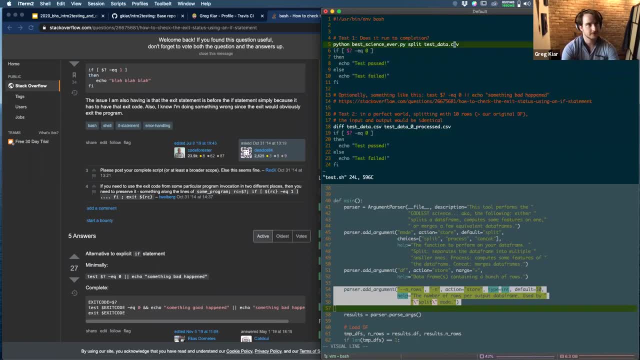 annoying and that we're seeing a bunch of things printed to our screen that we don't necessarily want. What if we just never want to see the output of these, uh, of the, the commands? we just want to know if they passed or failed. 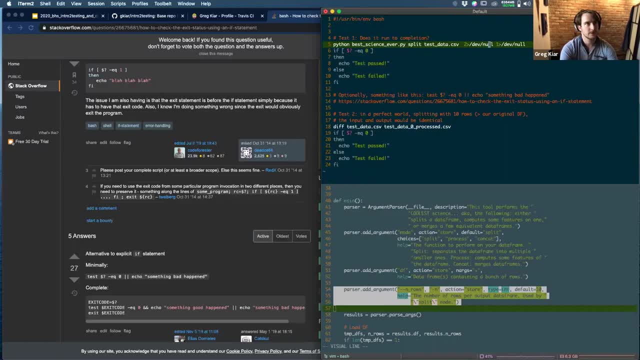 We don't necessarily care how they passed or failed yet, We just want to know the report. So what I'm basically doing here is: um, whoops, uh, actually that's fine- Um w. what I'm basically saying here is: take all of your um, your outputs, basically that. 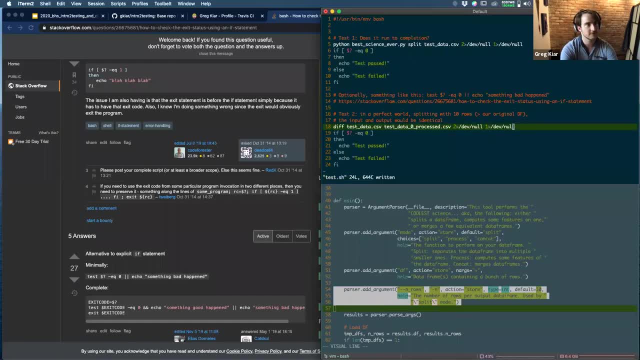 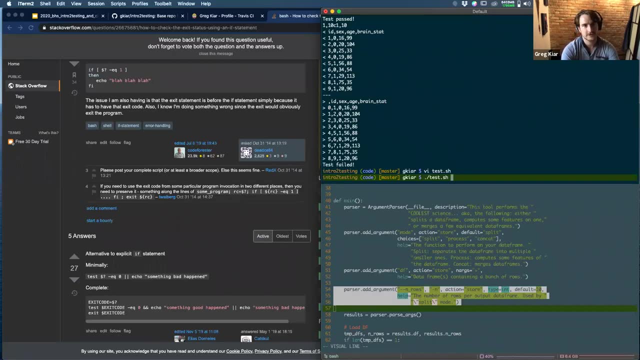 are either the, you know, normal printed outputs or the error messages, and just throw them away, And you're called dev null, which your system has. um, which basically says don't print them to the screen anymore. Um and voila. now, what we're we're doing is we're, you know, running a two tests. 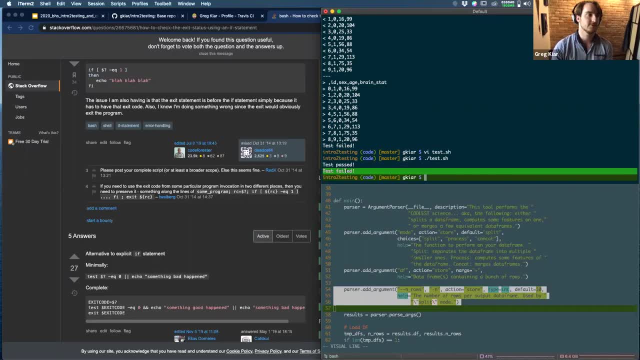 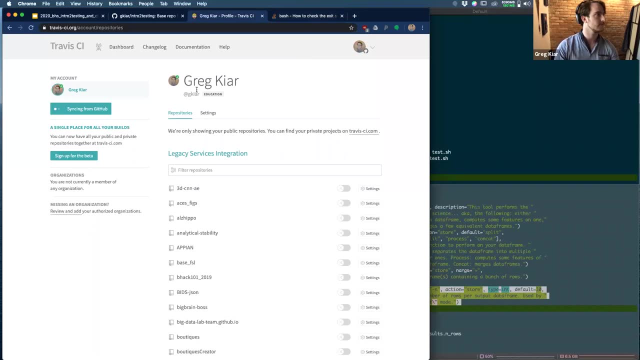 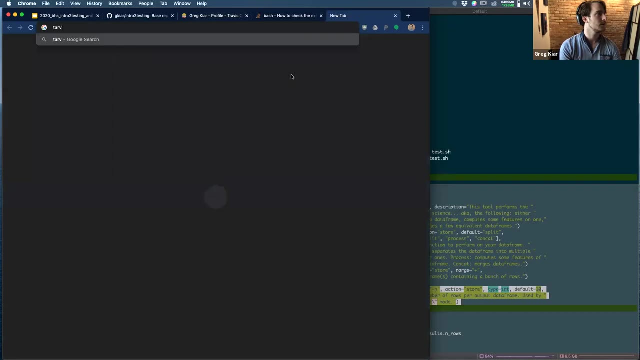 We're saying that it did successfully execute, but the result was not exactly what we wanted. Let's quickly go back and check if Travis has finished syncing. My goodness, I'm going to try traviscicom. Uh, uh, I don't know if there's a dash in that one. 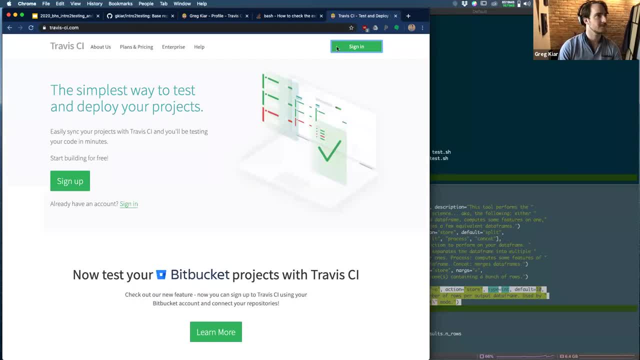 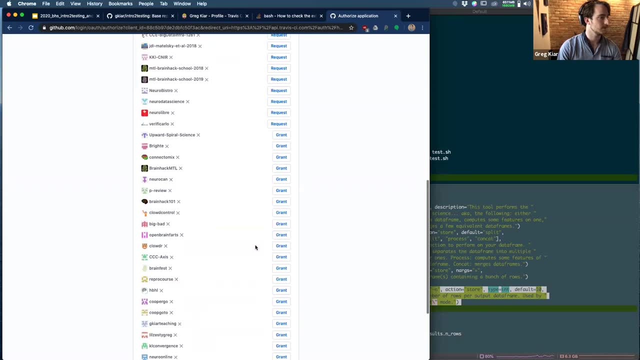 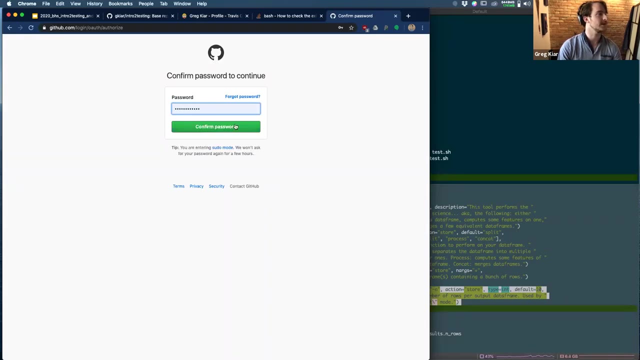 Okay, There is, But they did it for me. Sign in with GitHub. Apparently, I don't use this version often Um too many organizations. Oh well, I don't want to give you guys my password. I mean I like you, but okay, cool. 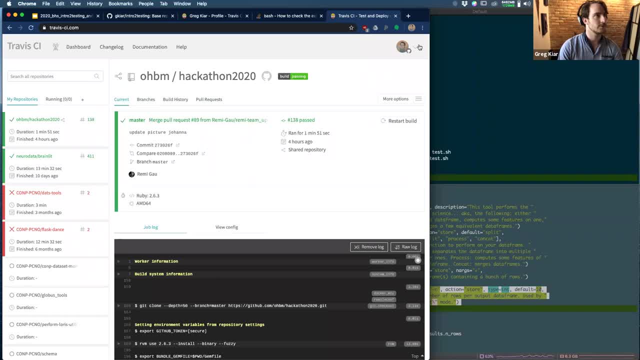 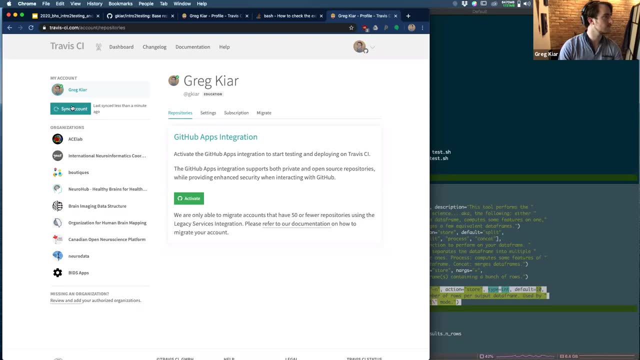 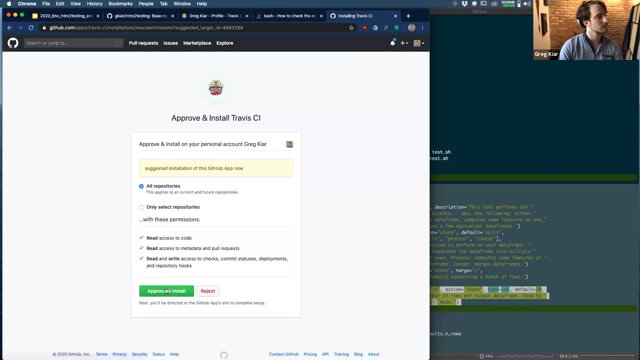 All right, So many more projects. Let's see if this one wants to work for me. So again going to settings: um, I want to uh sync. I want to activate um all repositories, only select. I don't need that many repositories. 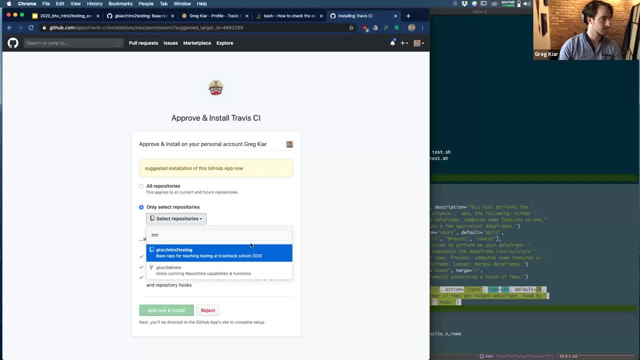 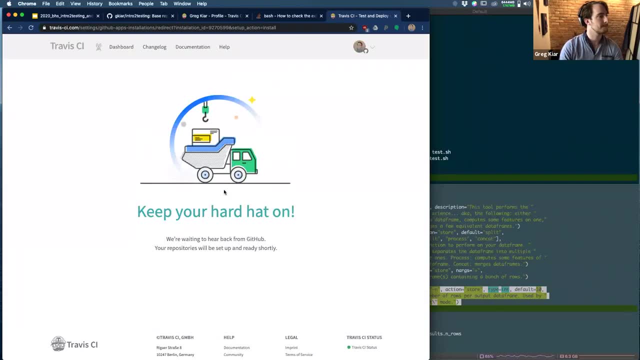 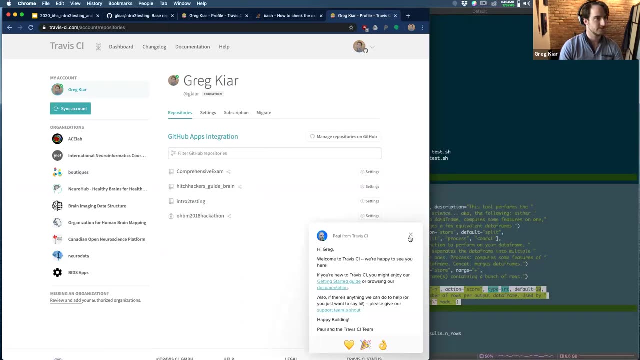 I just need this one for the sake of teaching right now. Okay, Approve and install. That's fine. Okay, All right, Let's see if this wants to work for us. Okay, Cool, Travis is doing something We have. I'm going to ignore the person trying to talk to me. 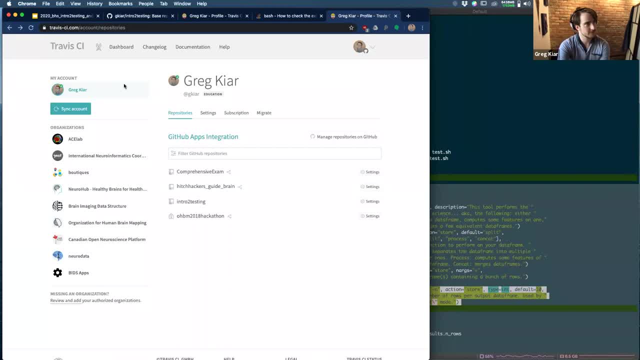 Awesome. So what I just did very quickly was pretty much allowing um Travis to have access to my account. I just again went to the pro version because I have an GitHub education account, um which again I think Sam was mentioning to you earlier in the week that it's a great way to um. free access to a lot of things you'd normally have to pay for, Um, but it seems like this version uh was allowing me to to um to set things up, So here I gave it permission and now it recognizes that my repository exists, but it says the. 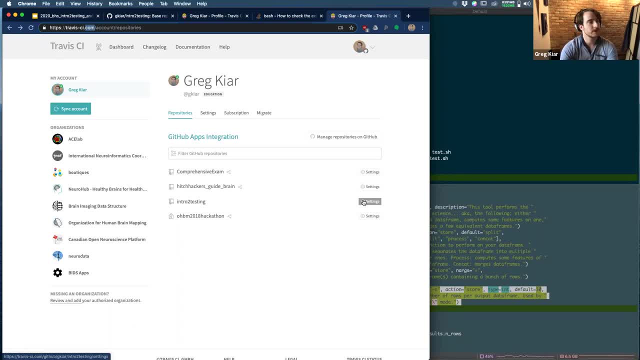 build is unknown. So what I think we'd like to do is, now that we've, you know, written a test, we would probably like to try and install our um installer tool and run this test on, uh, the build. 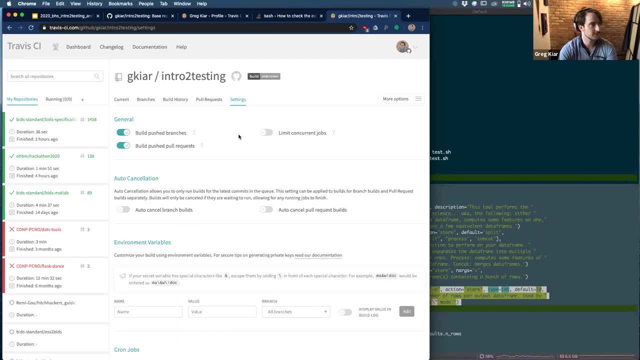 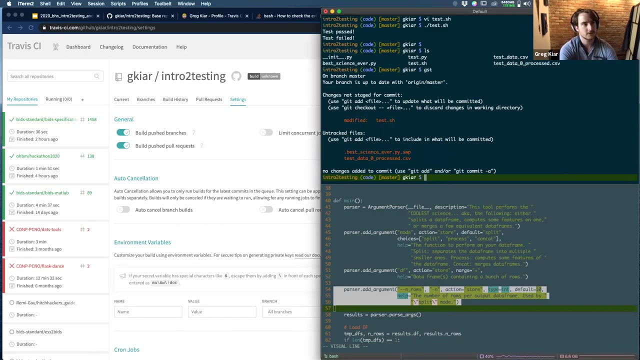 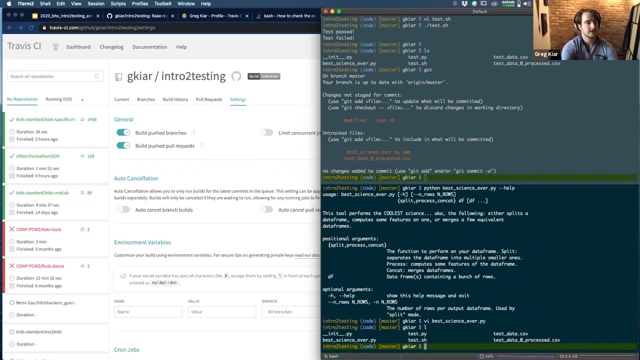 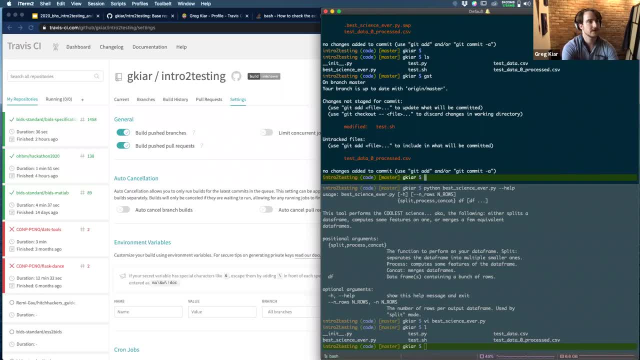 So let's see, Cool, I'm going to. I don't need to add the test data file, but I'm going to just commit my testsh added two tests. um runs successfully and files match. you know that name isn't. 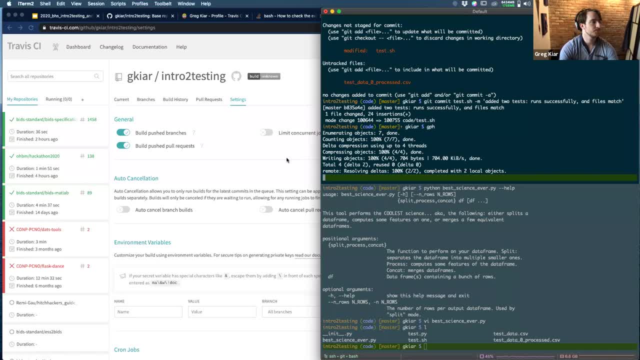 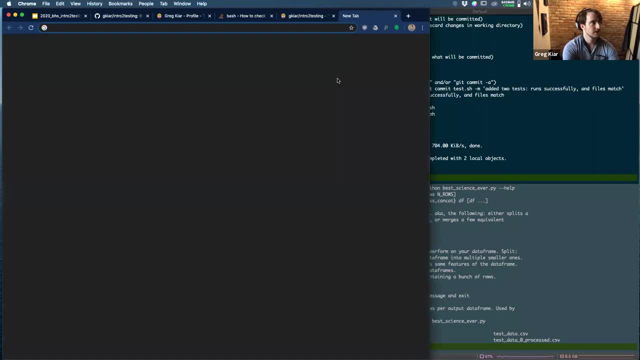 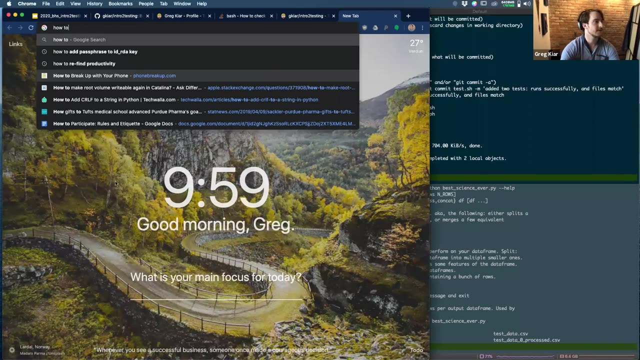 perfect, but it exists, Um cool. So let's see: build unknown. Well, I guess. what's the next step? I suppose how to set up Travis, to build my repository. Set up Travis. Look at that, The first hit on Google. Let's hope it's not just. 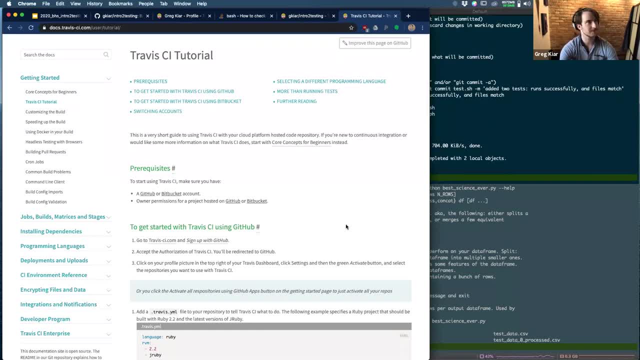 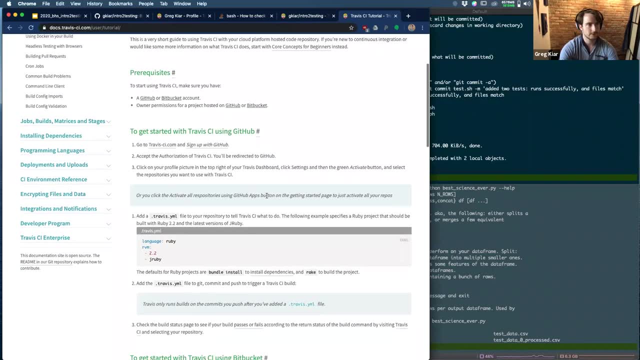 because I Google things like this all the time. I suspect that would be something that you guys would get as well. Again, the getting started guide is pretty simple. Again, I can't stress enough: the reason why I'm going through it this way is to simply illustrate that it's not about. 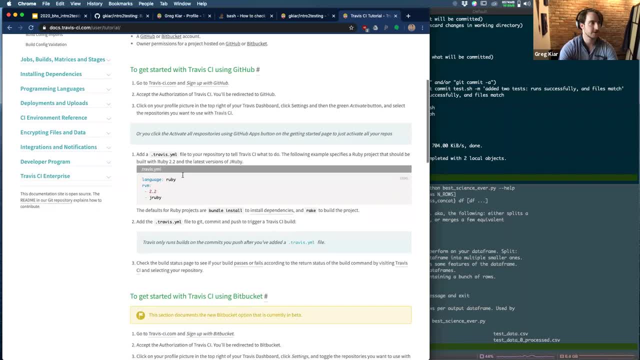 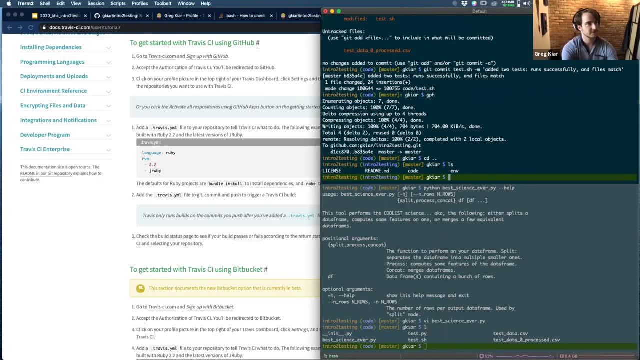 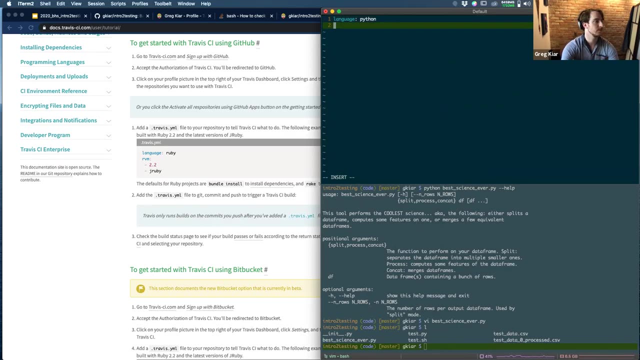 memorizing syntax. It's about just understanding the workflow. What I'm first going to do is we have a Travisyml already. I have that in the base directory of my repository. Inside of it we want to say language. In this case we're Python. I'm going to ignore them there. Then it 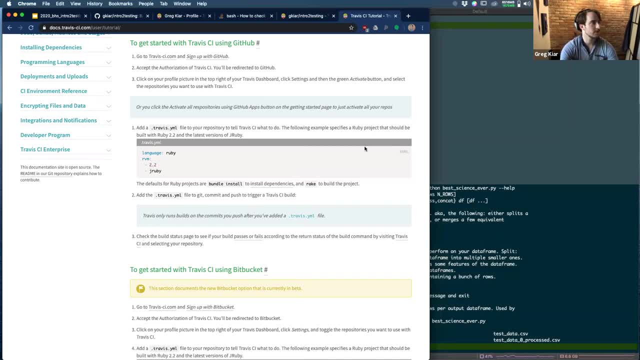 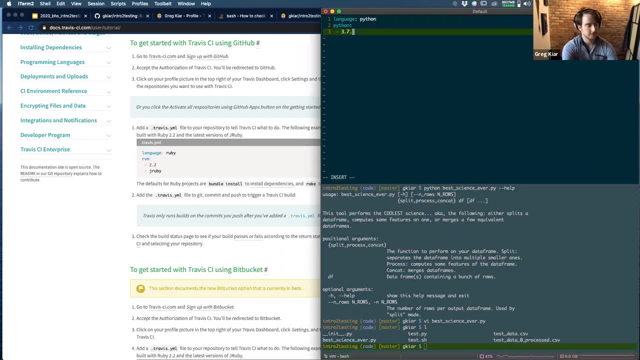 says RVM 2.2 and JRuby. I think what I'm going to do instead is Python and say 3.7.3, because that's the version I have on my local computer from when we typed Python dash, dash version. I'm going to just save my file. 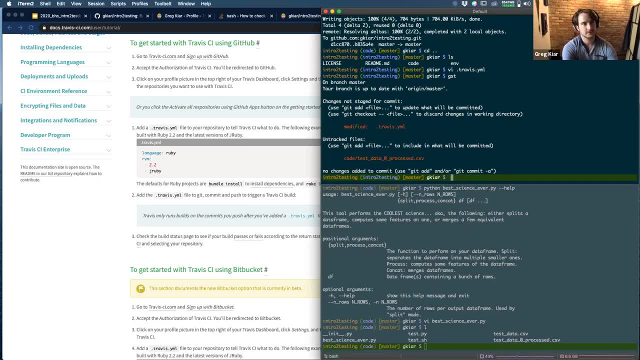 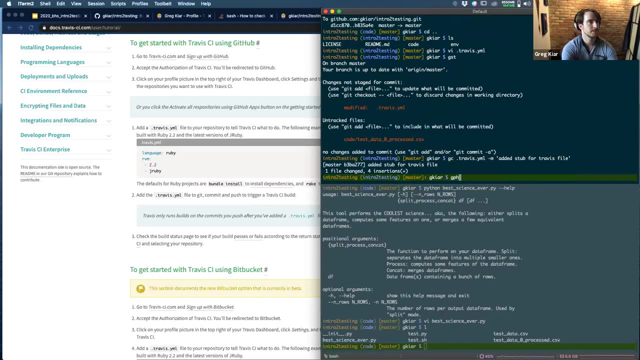 and now I need to commit it. GC, by the way, is just shorthand for git commit, in case you see me typing that on my computer. Then git commit: Travisyml- added stub for Travis file. Then gph is git push. Again, it's just an alias that I set up. 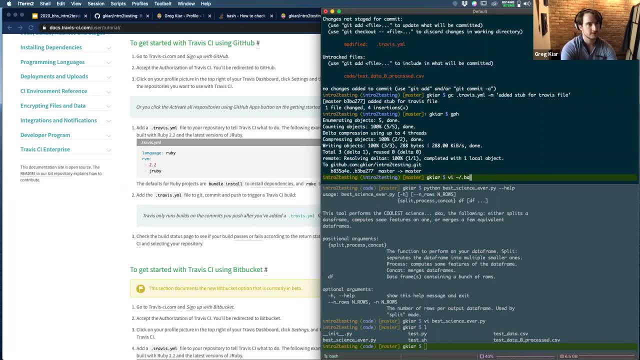 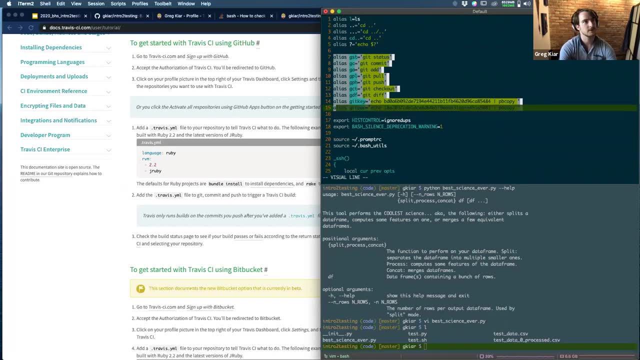 These aren't actual git commands. It's just things that I've set up so that I don't have to type as much, because I'm a very lazy person. I would recommend doing the same thing if you also find yourself using git a lot, because if you only have to type three characters instead of seven and you 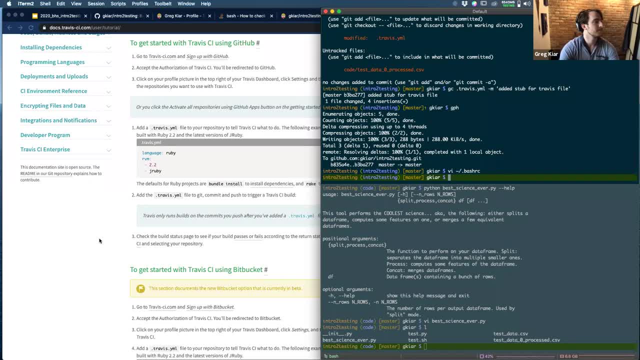 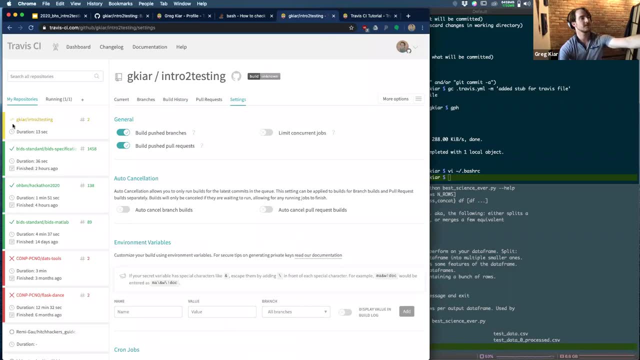 do this a thousand times a day. it adds up, But that's the tangent. So, anyways, we can go back to our repository And oh, look what's happening on the left here. It is building something. It has been running for 18 seconds. 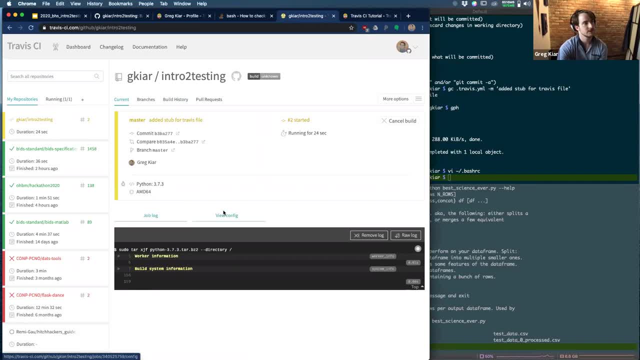 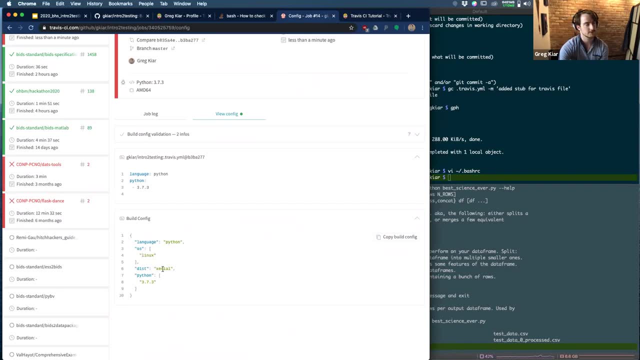 And as soon as I created my little configuration file again, the Travis that I just wrote it recognized that it's going to build a Linux operating system using Xenio, which I think is 18.04 version of Ubuntu. Then you know Python with this language, Python and version 3.7.. So 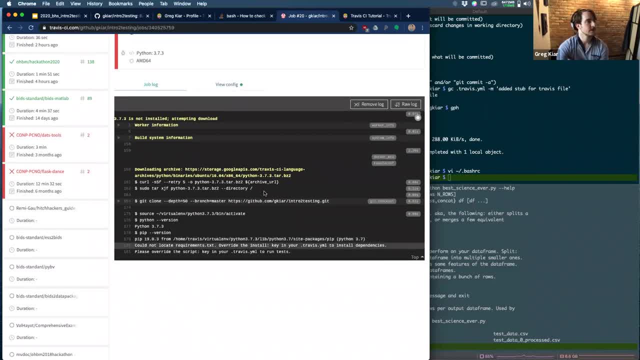 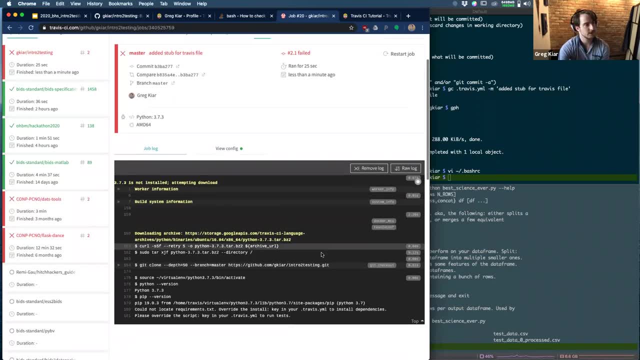 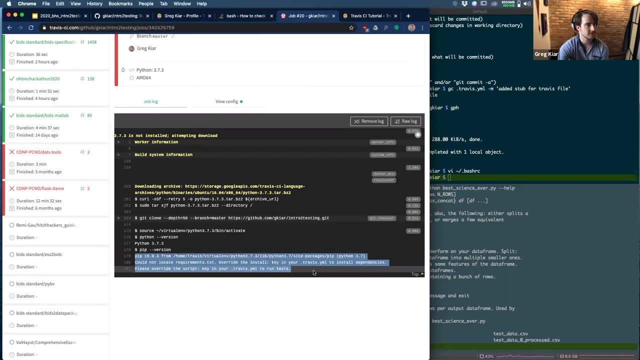 it's basically what I said. It interpreted it correctly. It is: could not install requirements. Okay, So it failed. Why did it fail? It installed Python, fine, And now it says: could not install requirementstxt. Override the install key in your Travis to install dependencies, or just you know. 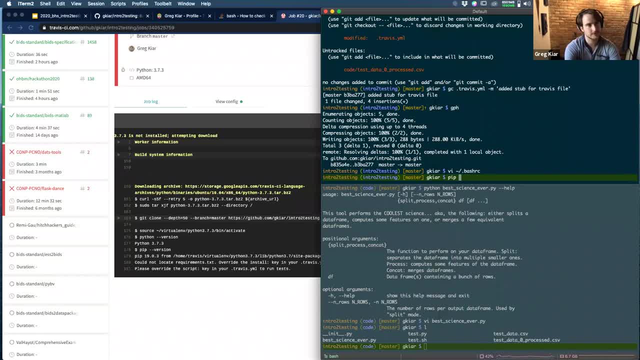 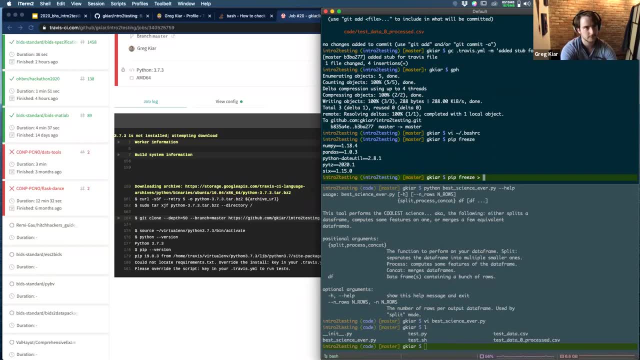 provide a requirements file. So remember the thing that I mentioned earlier. This is again just part of the configuration process. We did pip freeze. Pip freeze shows us the things that are installed. We know that all of this was enough to run our tool. So what I'm 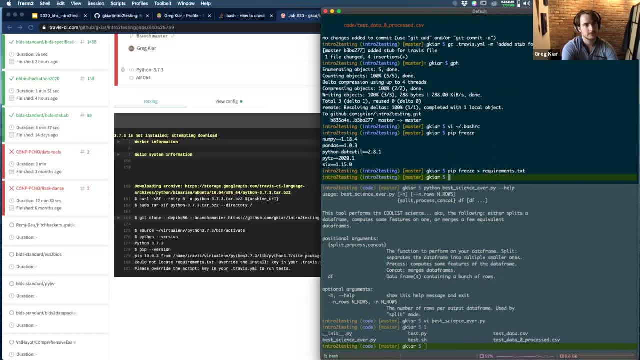 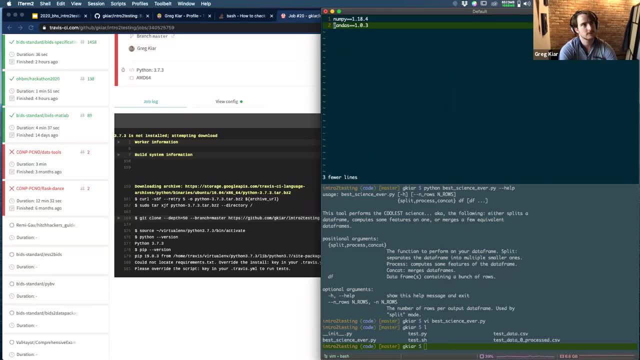 actually going to do is just take the these tools and put them into a requirementstxt file And, as I said, I'm just going to take the tools and put them into a requirementstxt file And, as I said, I actually don't really care about these ones. These aren't really things that we necessarily 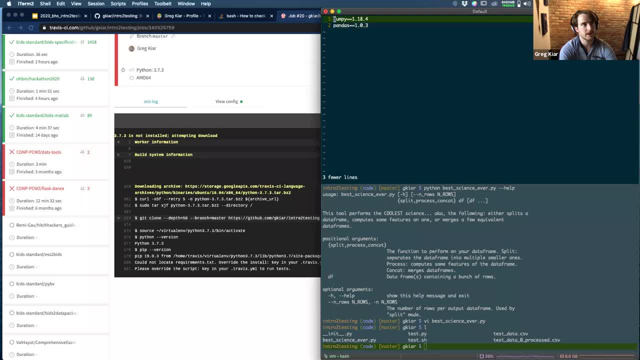 need. They'll be installed anyways, with NumPy and Pandas, But the important thing is we want to keep this file as small as possible, because that way it prevents possible version conflicts. So here, we know that we need NumPy, and we know that we need Pandas, And we know that it needs, you know, we. 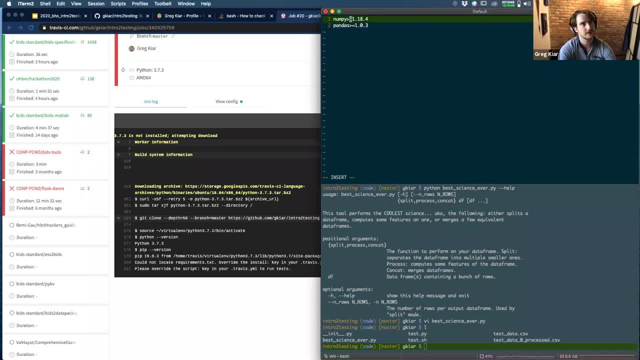 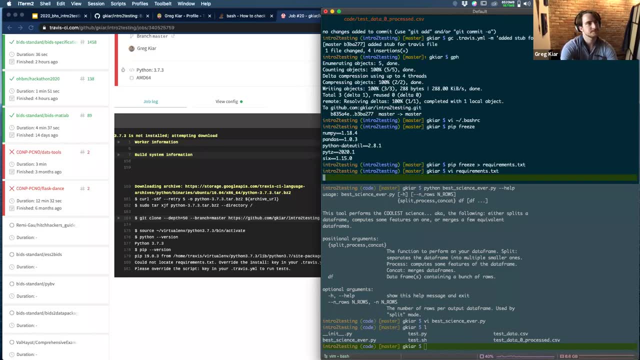 know that it works with these versions, But maybe we'll be a little more generous and we'll say greater than or equal to these instead of exactly these versions. So then that way, if there's a new update, it can grab a newer version. So then what I'm going to do- GST again in my world- is: 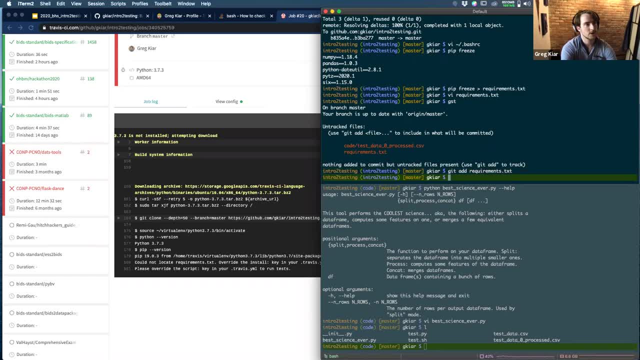 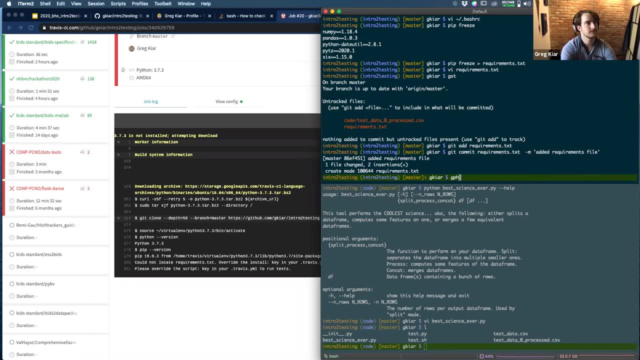 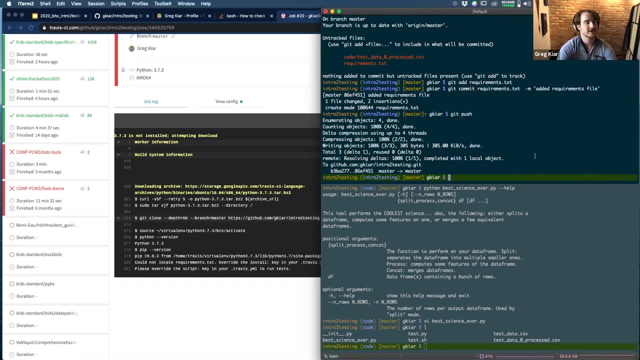 git status. I'm going to do git add requirements, git commit requirements- added requirements file. Again, I'll try and remember to type the long versions to make it more clear. Now I'm pushing. I realize I'm already over time, So I'll try and speed along in the next step. 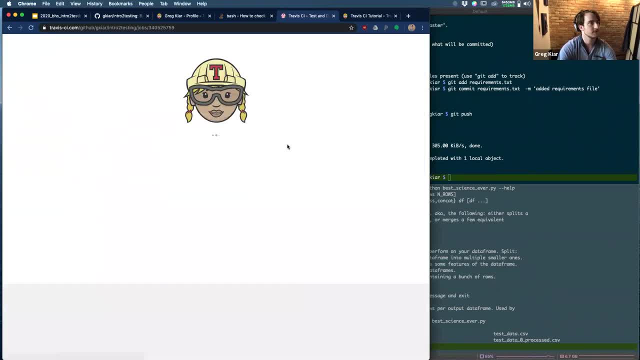 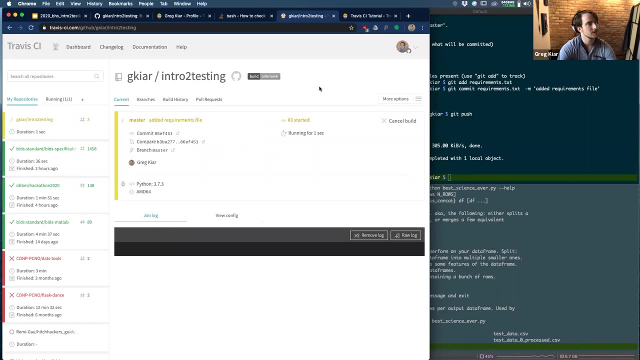 But let's see. So now I've pushed my changes, I'm going to click on this thing again and see when it updates. I'm just going to keep refreshing the page obsessively, Don't mind me. There we go. So the nice thing that you noticed here is that I'm pushing my code to GitHub. You know nothing. 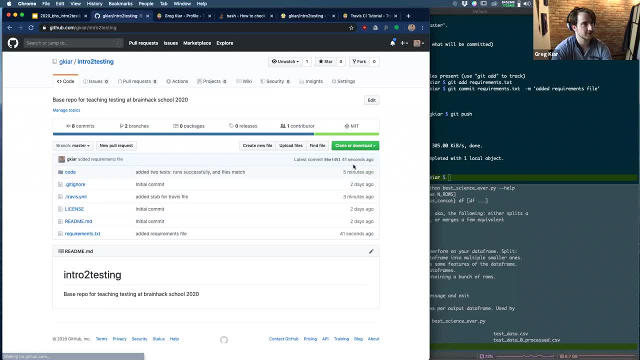 has changed. I can refresh this project and it'll say: you know, commit added 36 seconds ago. Oh, so close 41 seconds. So I'm going to push my code to GitHub. Nothing has changed. I can refresh this. project and it'll say: you know, commit added 36 seconds ago. Oh, so close, 41 seconds. So now I'm going to force my code to GitHub. Oh so close, 41 seconds. So now I'm going to push my code to. 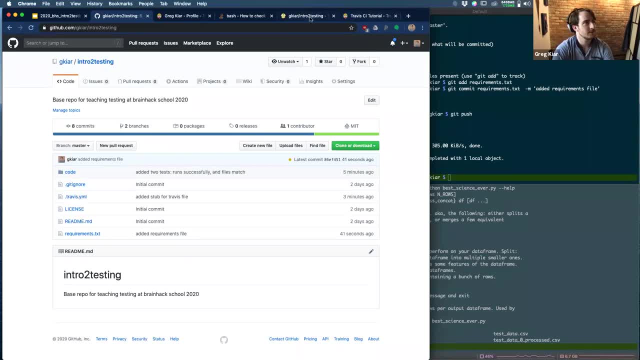 GitHub- Oh so close, 41 seconds. So now I'm going to force my code to GitHub- Oh so close. And then what Travis is doing? is it recognizes? oh, the code changed on GitHub. I'm going to try. 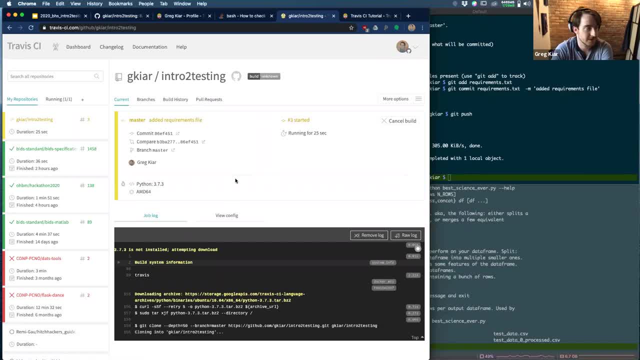 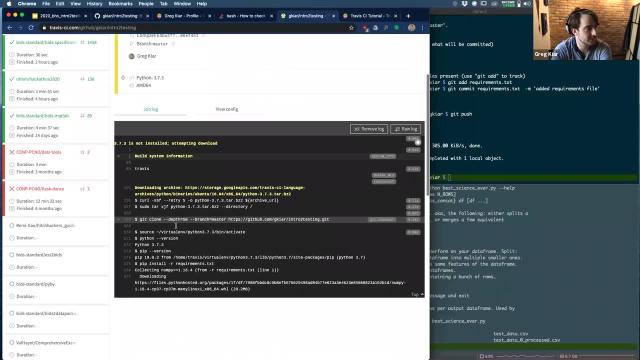 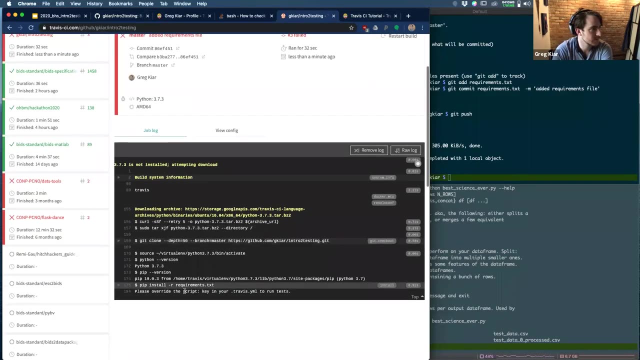 to start building things again. So that's exactly what happens. It again creates an environment with Python, It'll grab the requirements file we created, It'll install things And voila: It failed again. Why is it failing now? Now, what it's saying is: please. 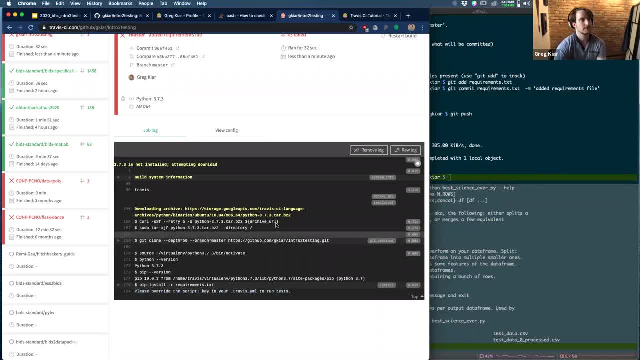 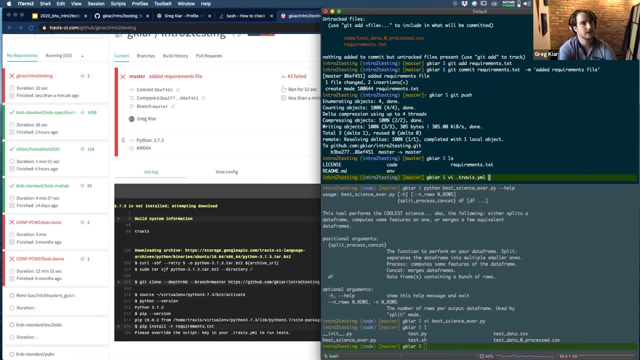 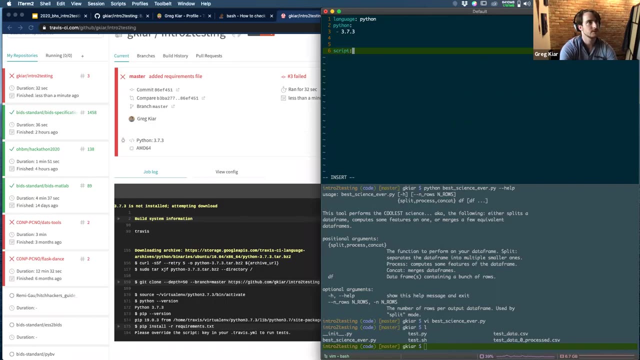 Please override the script key to run tests. Cool, So we may be installing something, but we aren't actually testing anything yet. So what we're going to do now is edit our Travis and do exactly what it says It said: override the script key to run tests. 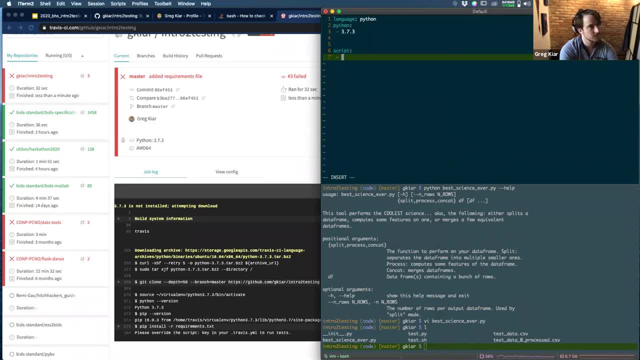 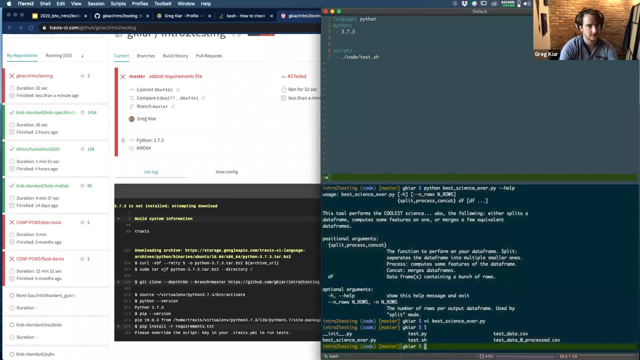 So I'm going to have that be my thing. excuse me, my command is just going to be to run this test. So the test was in the code folder and I think it was testsh. I'll just verify that that's the case by. oh yeah, it is right here. 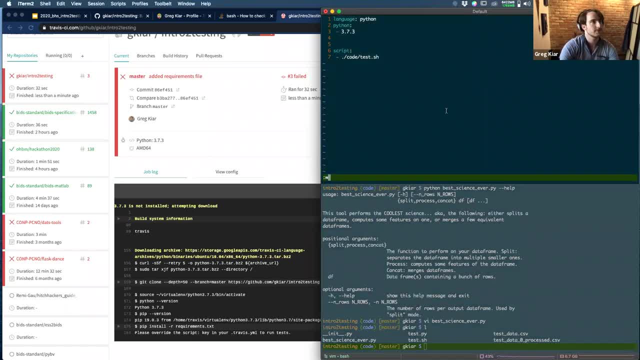 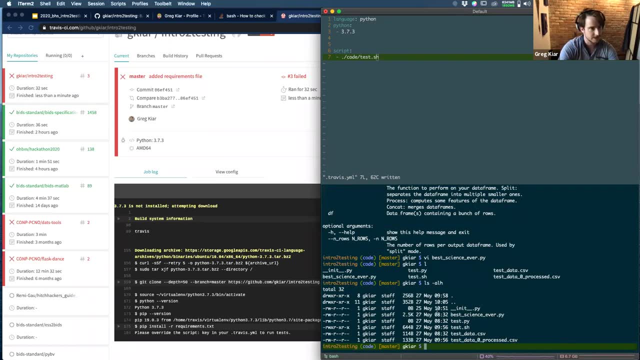 You can see it in my bottom terminal. Cool, Does it have execution permissions? though I believe it does, because I changed it locally and then I recommitted since. But I'll do an LSALH and we can indeed see that it has execution permissions. 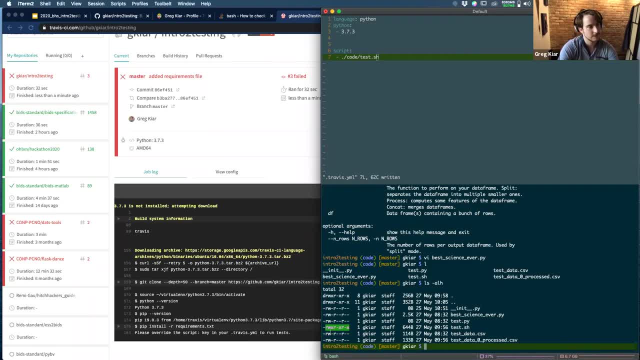 So again, remember- I'm not sure if you guys were taught much about permissions yet, but there are three levels. There's read, write and execute, and there's also three kind of people that these apply to. They can apply to the owner of the file, they can apply to people who are in the group that 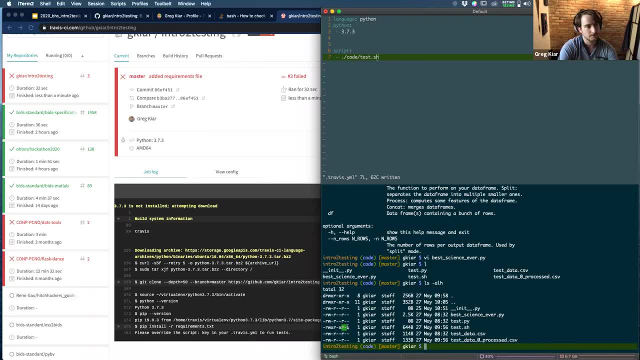 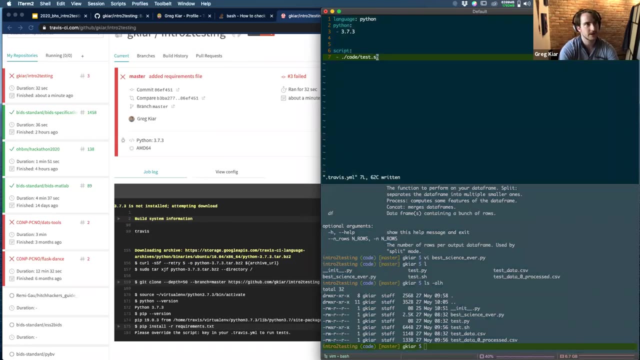 owns the file and they can apply to everyone else. And so when I did chmod plus x, as some of you may have noticed earlier, what I was just saying is add the executable permission across the board to this file. So when I committed the file after that, it kept the permission. 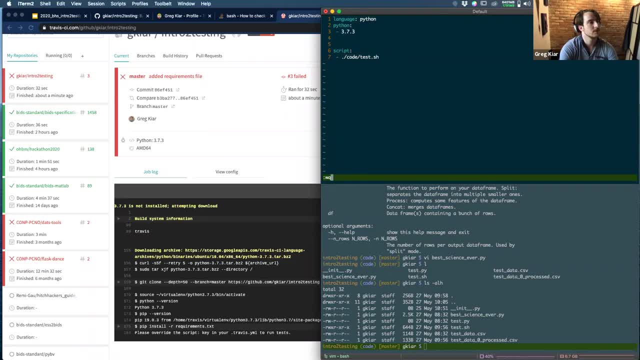 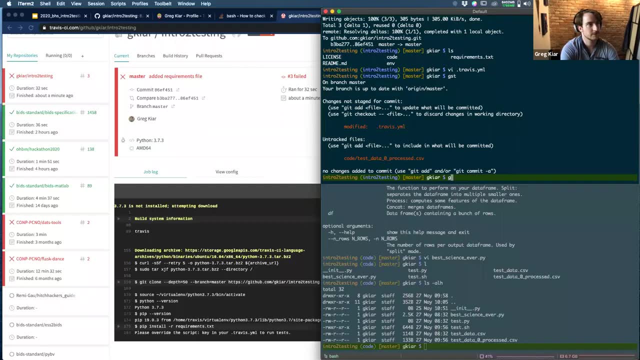 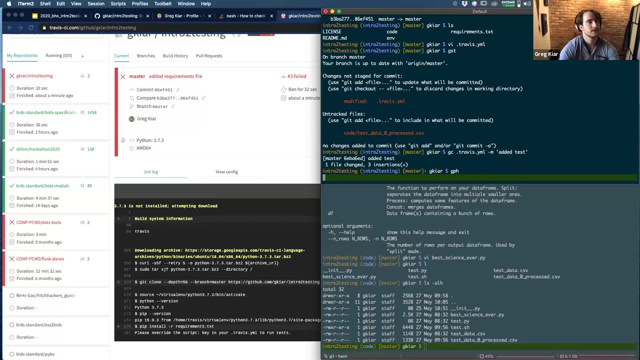 So now I'm going to do this, okay, And let's see git status, git commit, Travis, add a test and push. As you can probably already see, it's much faster for me to type gph than git space push. 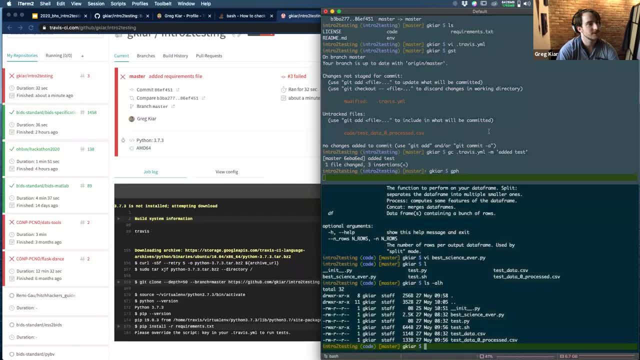 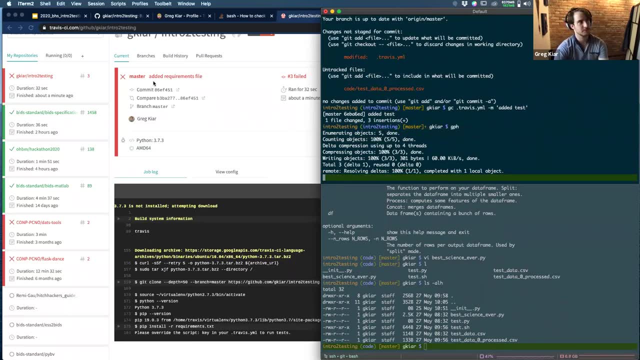 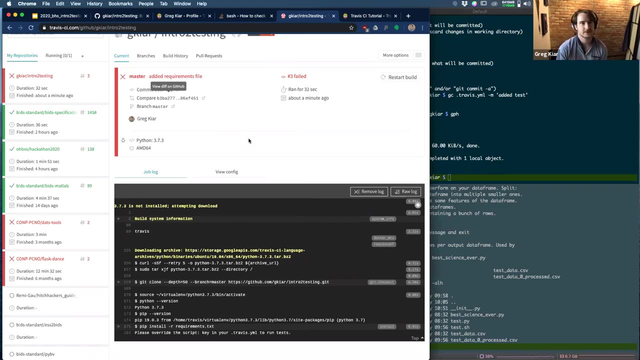 every time. But yeah, When my internet decides to work, it'll work, But hopefully, what you guys are getting a sense of at this point, we will see that the script will run again once this updates and then we can continue to iterate on this. 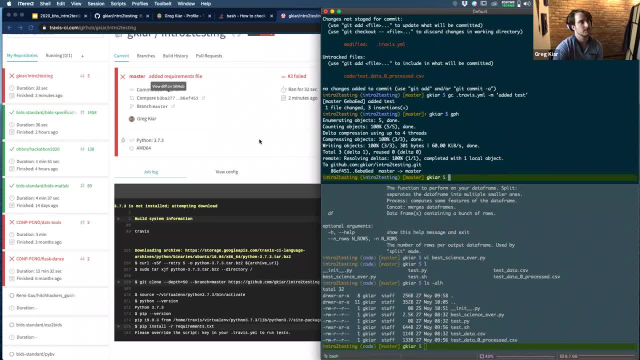 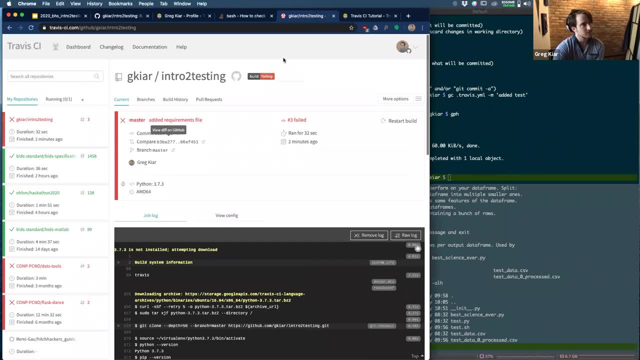 process. We can test more functions of our code. We can test do a better job at comparing things. We can make changes to our script so that the tests all pass. And then one thing that you've no doubt seen on projects is we get this cool little batch. 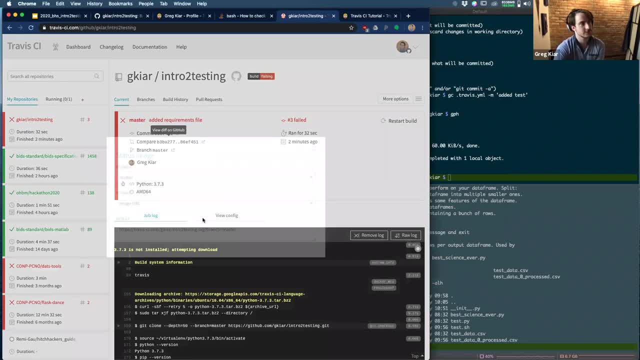 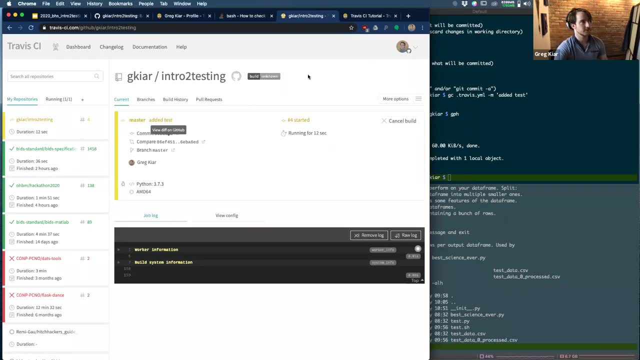 and you can include this in your project So that you and all of your users will know the state of your project, both in terms of is it building successfully- You can get other batches- in terms of how much of your code you're testing and things. 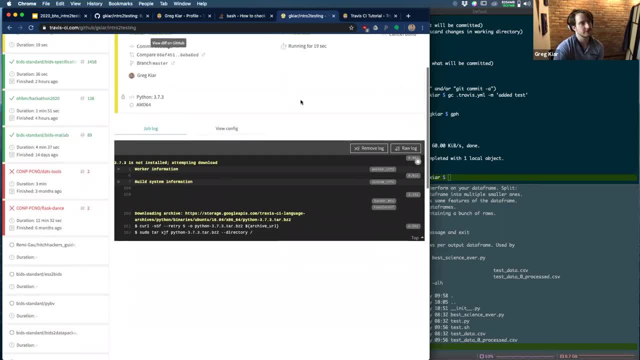 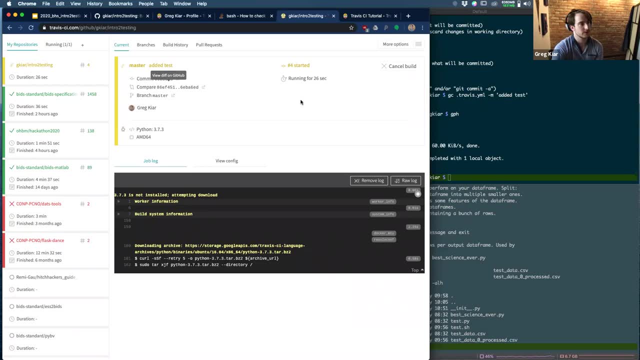 like that, But it's just a nice way to have, like a visual reminder of the state of your project. So again, once this finishes, there's one other point before I let you go that I want to, that I expect we'll run into that- I want to mention. 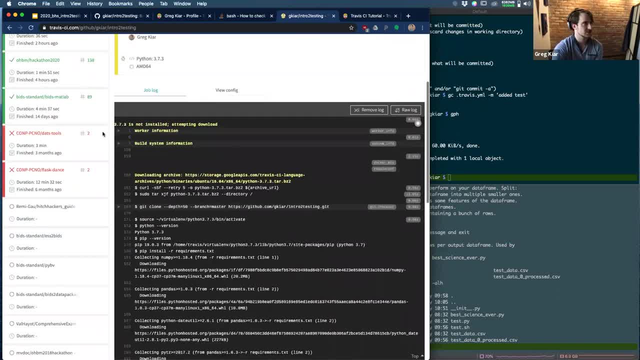 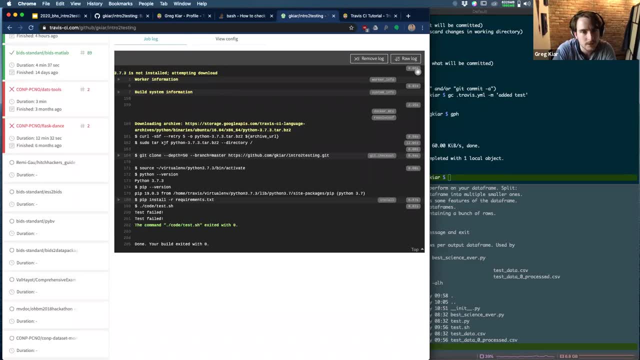 But then we're pretty much done, So I'm going to go ahead and close this. I'm going to go ahead and close this And we're pretty much there. So David asked a question. I can see them now, Yeah, So David asked the question. basically, should we use pip and virtualenv instead of conda? 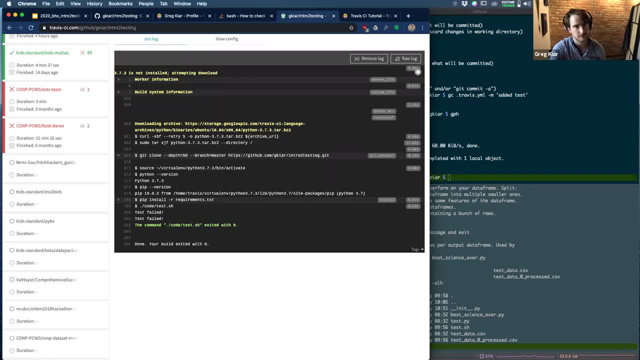 and standalone scripts instead of notebooks if we're using Travis, And what I would say is that- and I'll focus back on what happened here in a second- But what I would say is that in general- and this is an important point- with notebooks, 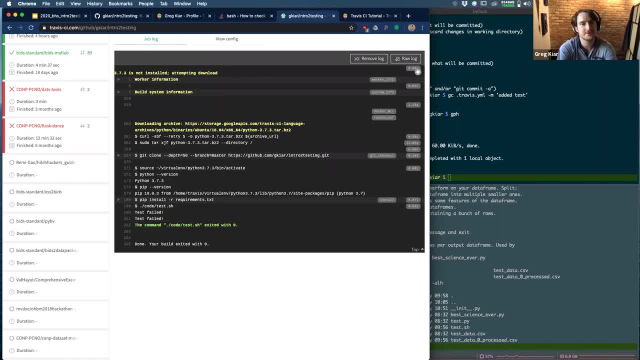 that. I'm not sure what you've been told to date, but I have strong feelings about notebooks and their correct use case, And what I would say is that if you are making something that is to be reused in the sense of like a script applied on new data, a Jupyter notebook may not be the right tool for that. 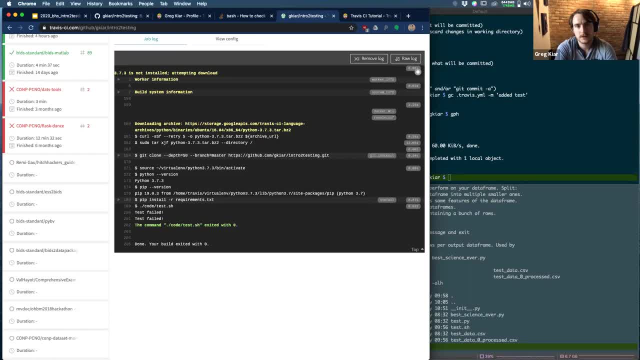 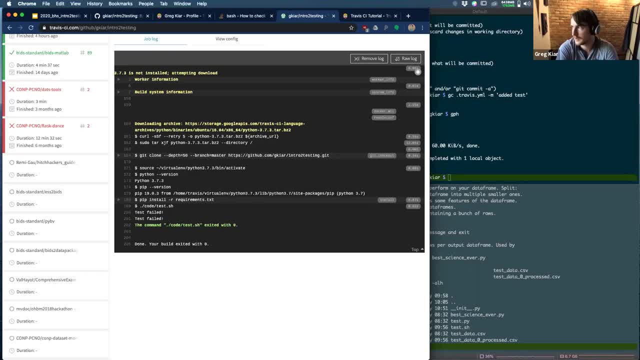 that it really is wrapping something called interactive Python, IPython, which means that really, a Jupyter notebook is a shell. It is a terminal that you're working in with Python and it just happens to keep memory and embed figures for you. so it's pretty and nice to look at. 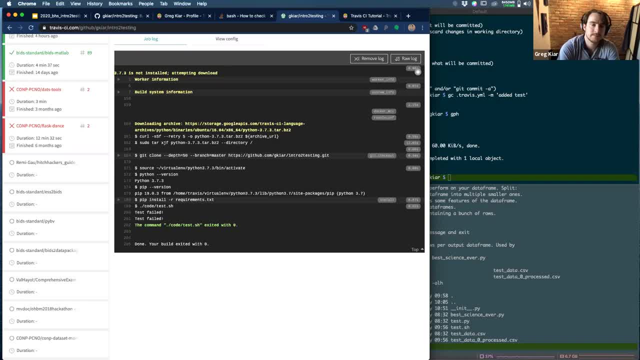 But it is not actually a packaging environment. So if you're trying to make a pipeline, an end-to-end pipeline that you run and reuse and distribute, a Jupyter notebook is not a pipeline. A Jupyter notebook is almost never the correct tool for that, and what you want to do is: 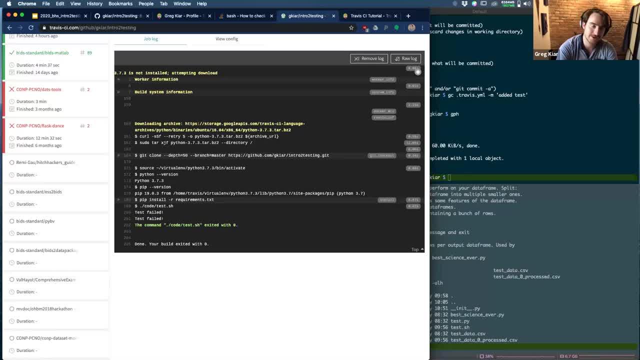 work in scripts And that doesn't mean you can't then import things you wrote in your scripts into your notebooks and use them again there and things like that, and Valerie's going to be talking about packaging tomorrow, so you can see a bit of how you create these scripts and packages. 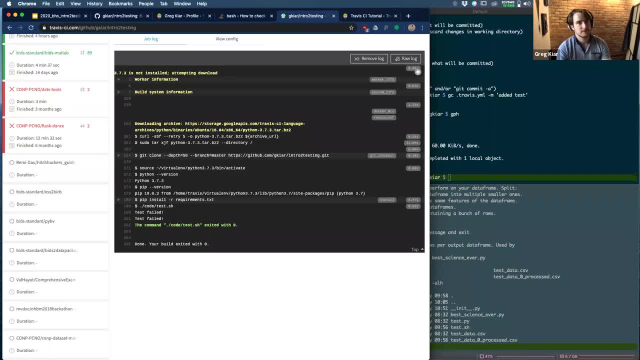 so that they can be imported again either in a notebook or in any other script. But the correct thing to do if you're making, say, like a pipeline or an analysis workflow may not be a Jupyter notebook And it's worth if you're on the fence at all. it's worth asking TAs in this class and 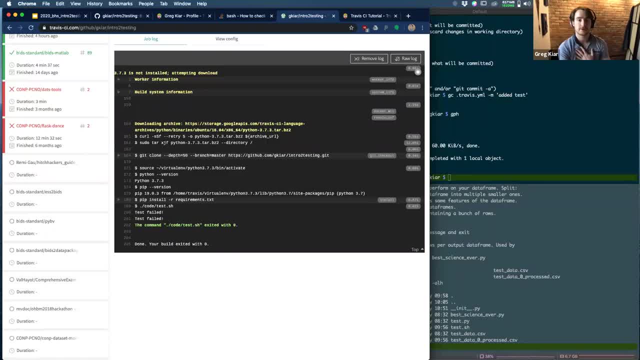 instructors to give their opinion For my own personal use. the only time- the only two times actually- I use notebooks at all- is one for teaching, because it gives you a pretty web interface so I can use the browser, and two if I'm making figures. 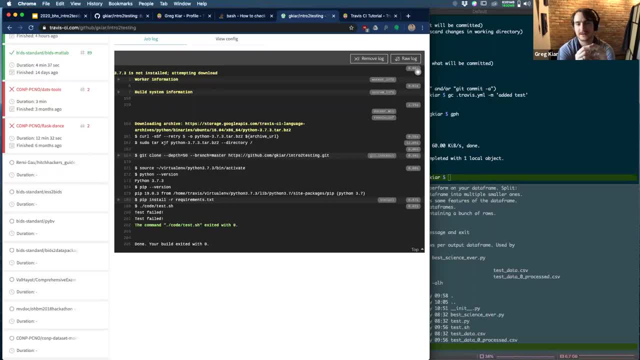 And the reason for making figures is because that's a thing that I would typically do in like a terminal anyways, And this way I get my figures in there. They're in line with my code, Everything else I do in scripts and again, for the main reason being that I can package. 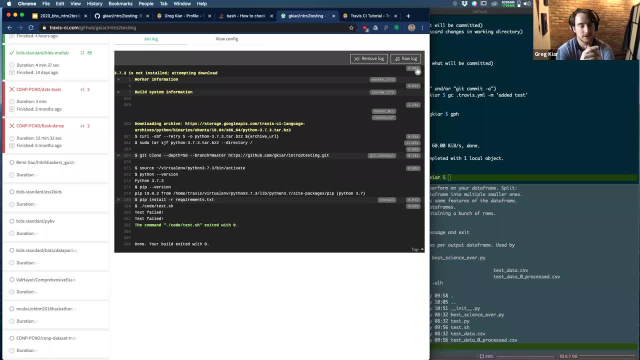 it, I can distribute them, I can reuse them more easily, and so on. So, yeah, so thank you for the question, David. That was very timely And I have noticed that, you know, a lot of people are using notebooks, so just remember. 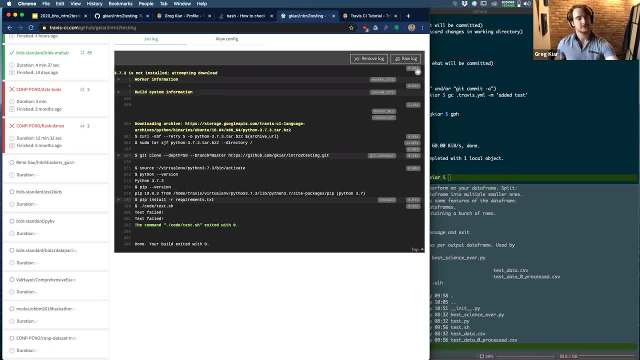 that they are a wonderful tool, but just not for every application. Maybe to complement that it's also possible to: Yeah, If you actually write a Python library that is called from your notebook. So if your analysis becomes too substantial, let's say you start having you know a few. 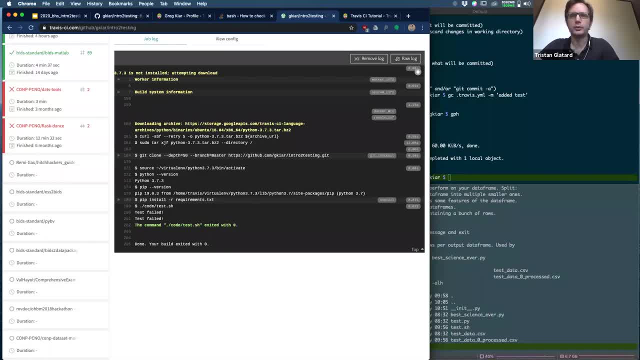 hundred lines of codes, then you know you can also write them in a Python package independently from the notebook and then just call these functions from the notebook And these functions can then be tested on Travis, if need be, independently from the. 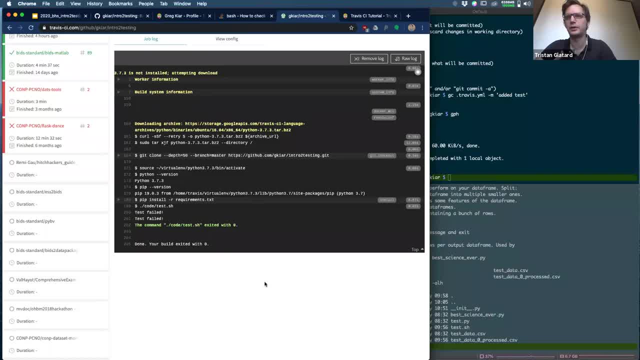 notebook, Because it's true that testing things interactively is going to be difficult, Right Exactly. And again, Valerie will teach you about packaging tomorrow, and that'll make it much more clear how to do all of these pieces and work with them together. 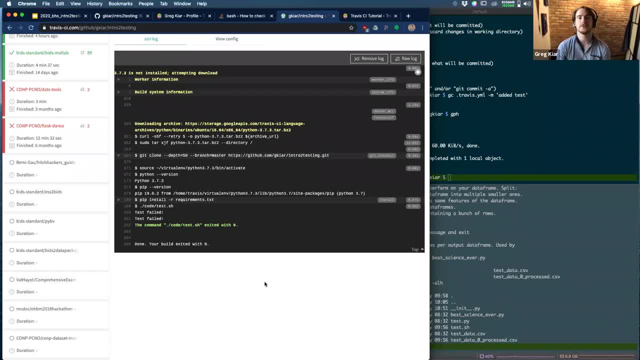 But yeah, in general I will say, for everything you're doing that you want to be reusable at all. avoid notebooks when possible. Oh, it seems, Shimo, just I think copy-pasted the questioning content, Cool. So the last thing that I just want to touch base on here before letting you guys go again. 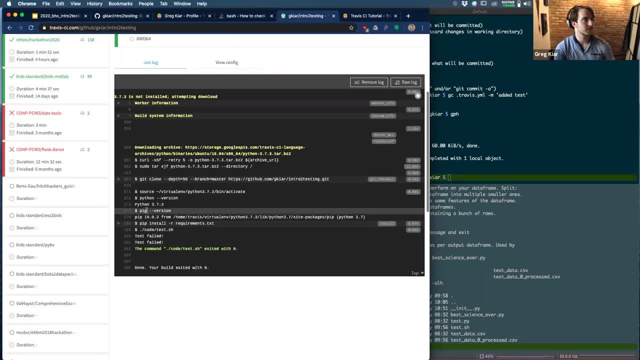 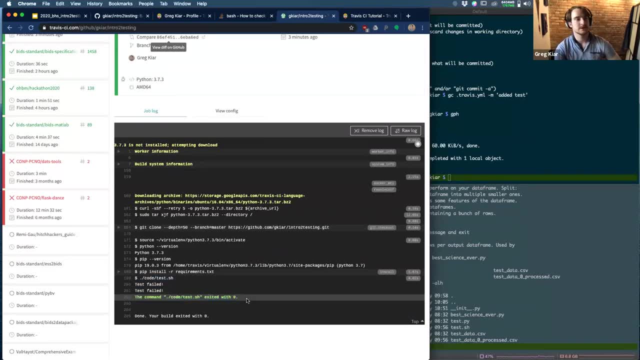 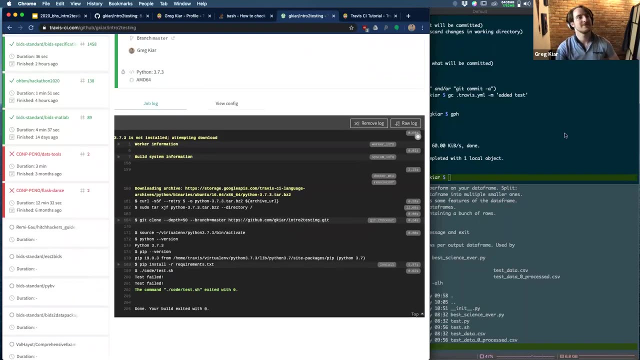 sorry for the delay, Sorry for keeping you. We see two strange things happen here. One, we saw that both our tests were failing now, And two, we saw that our build succeeded. So this seems a bit confusing, So I'll just- rather than again, since I know we're short on time, rather than asking you. 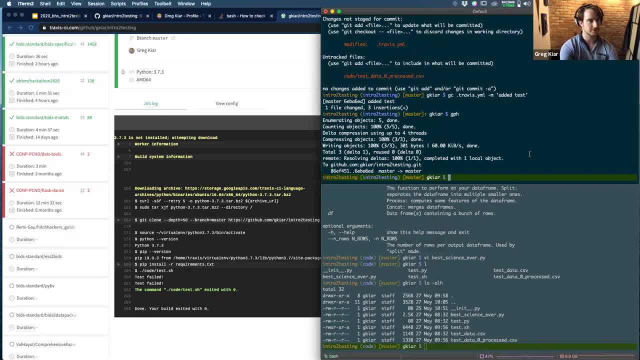 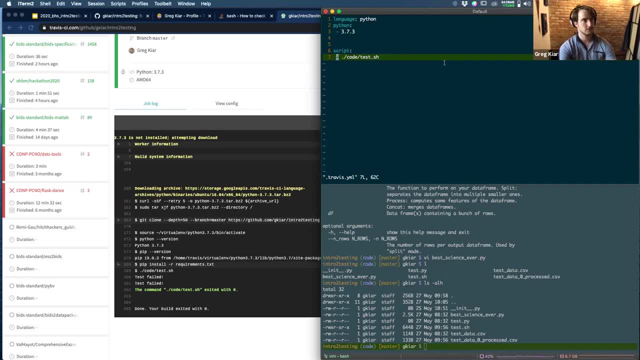 guys to debug with me and figure it out. I'll explain why both of those happened. So again, if we look at our Travis configuration, what we said was run codetest- Sorry- in the code folder testsh- sorry. So I'm going to go inside this folder and see what's happening in it. 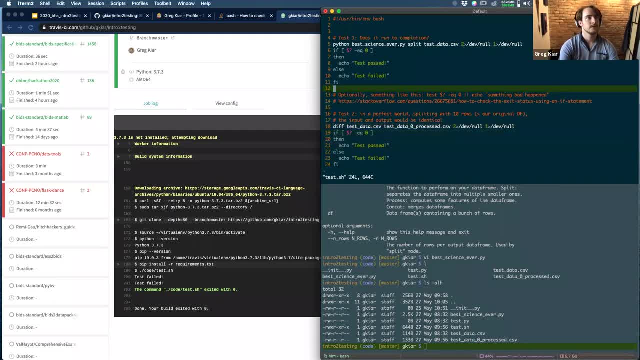 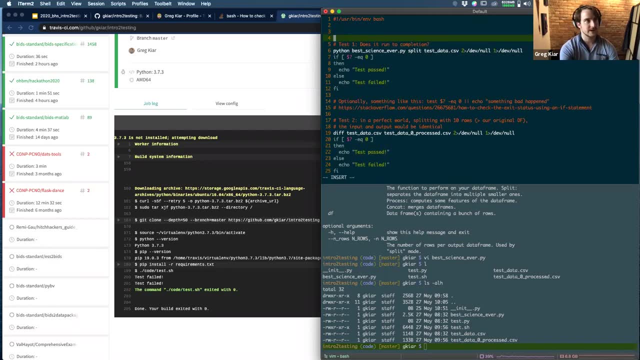 So again, I look in testsh and it's running our script with the mode split and all this stuff. Well, we haven't provided any path to our data yet, So we haven't. actually We're assuming that in the same directory as we're currently in we have bestsignseverpy. 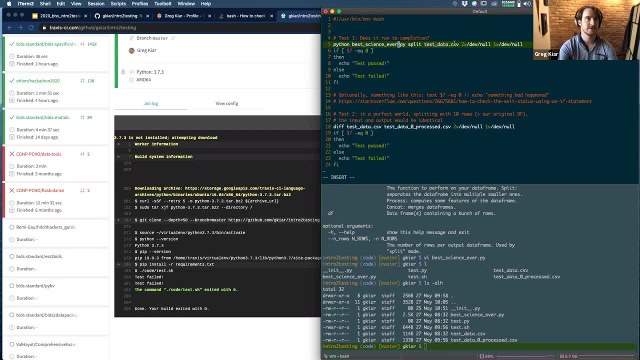 and we're assuming that in the same directory as we're currently in we have bestsignseverpy, and we're assuming that in the same directory as we're currently in we have bestsignseverpy, and then in the same directory we also have test datacsvpy or, sorry, csv. 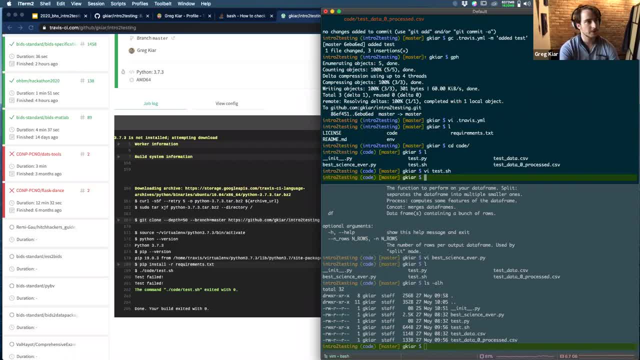 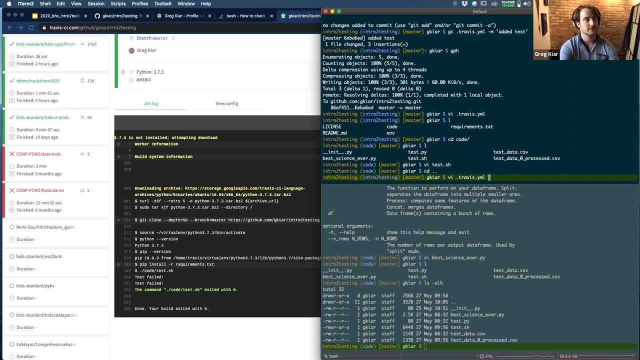 I can't speak anymore, So what we actually need to do in our Travis script is first in order for our It's in the wrong directory. What we first need to do for a Travis script is move to the correct location so that our 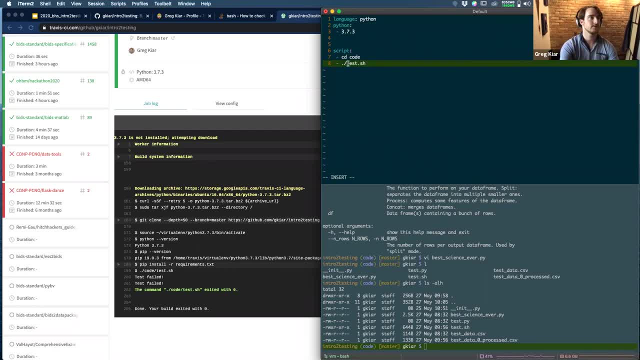 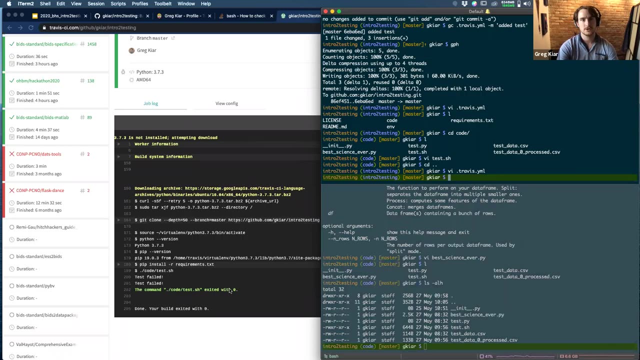 test will actually work, and then I just need to do that. So the first thing is, this will solve the first problem of making both our tests maybe not fail anymore. Now the second problem is that even when our tests failed, it looks like they passed. 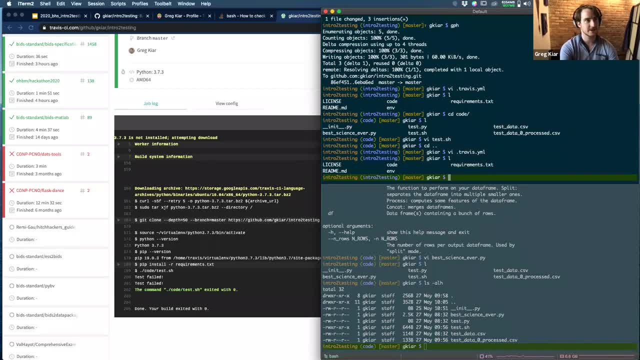 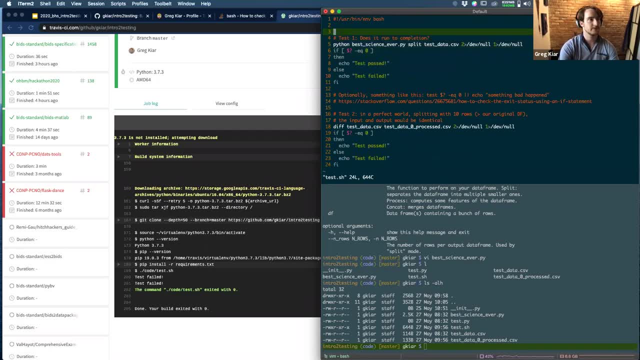 because our script that's running our tests didn't exit with an error code that wasn't zero. So what we're going to do here is we're basically going to say: I'm going to say EC equals zero, Zero, and every time that I get to one of these branches where a test fails, I'm just 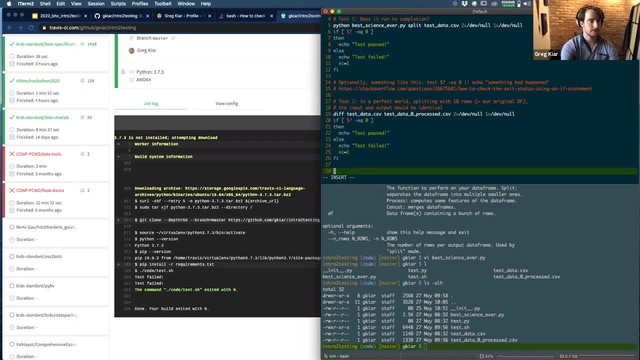 going to add EC equals one, and then I'm going to say exit and I'm going to call that exit with the code here. So basically I will by default say that my tests are passing by setting this line three up here. 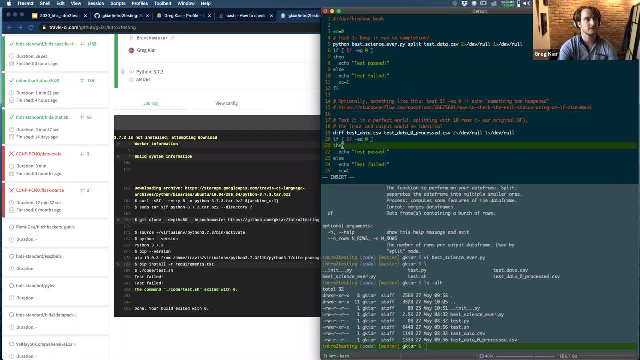 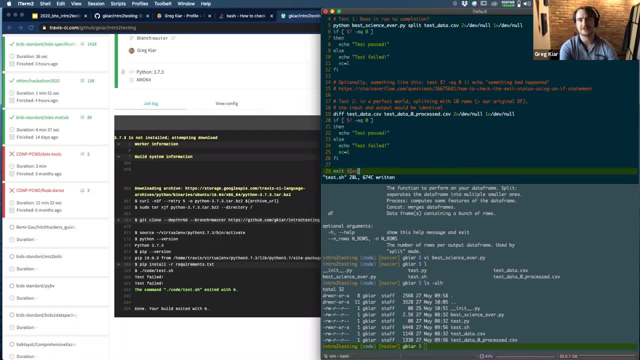 My error code, my exit code, is going to be zero, and every time I fail I just make sure that it's at least set to one, And then we're going to exit with that code, so that if we're actually failing, we're going. 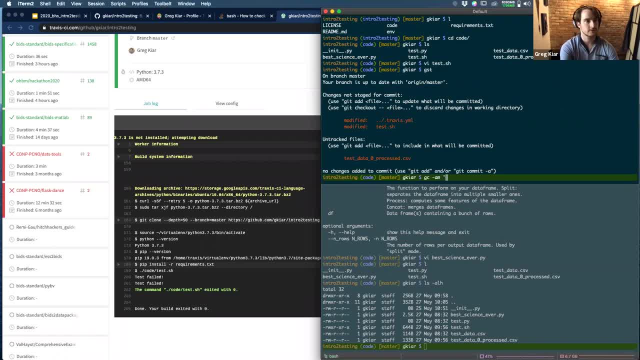 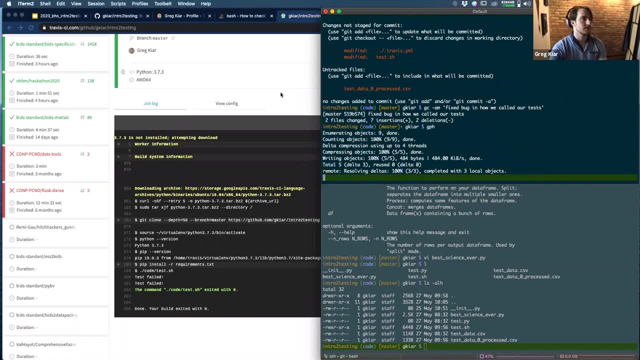 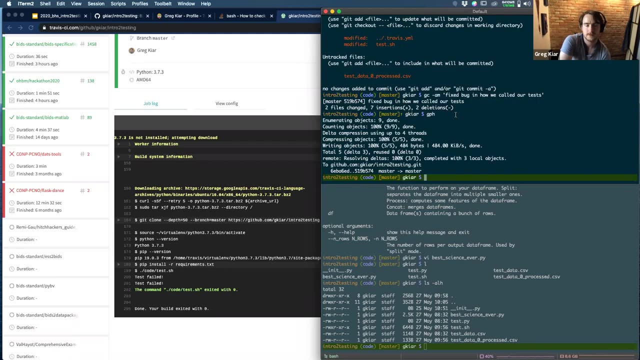 to communicate that properly. So I'm going to just bug in how we called our tests, and then that should solve both of our problems there. So while we're waiting, I guess we can field some remaining questions and then you guys can hop offline and start packing. 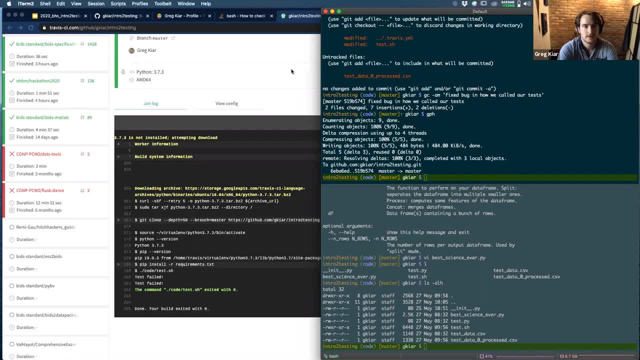 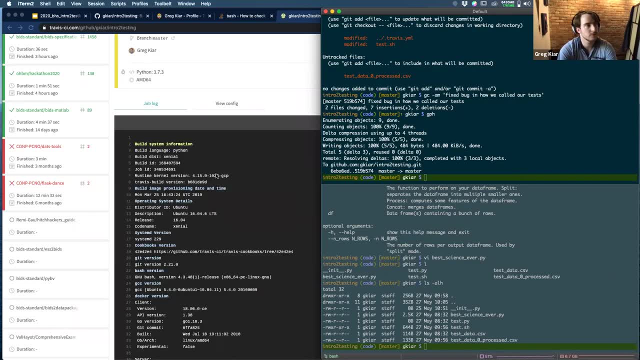 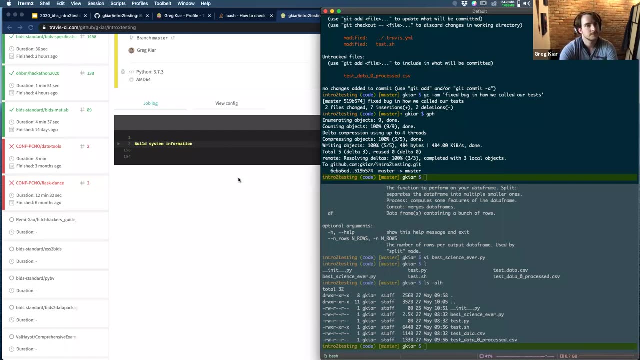 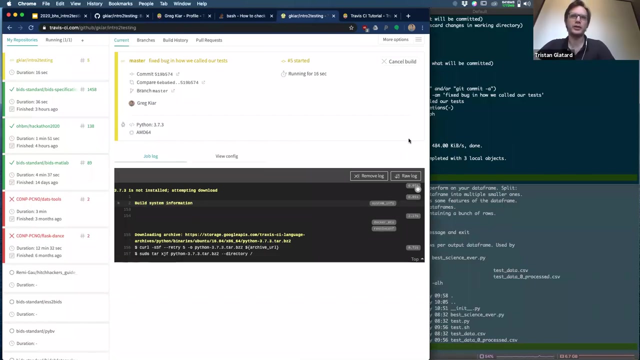 So are there any other questions so far? Again, feel free to unmute if you're more comfortable speaking than typing to whatever works for you guys. Maybe just a comment while people are maybe typing their questions. So typically the setup of continuous integration, the Travis setup in this case, is a one-time 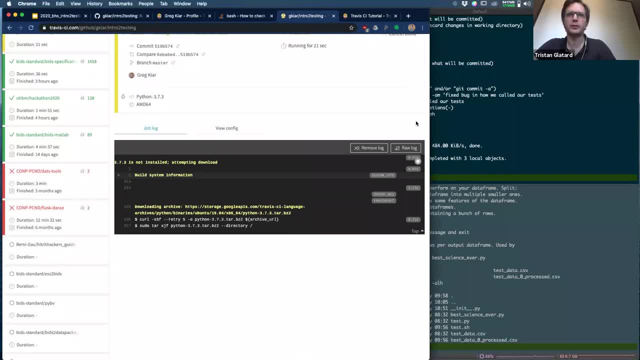 thing. So you would typically set it up at the beginning of your project And then maybe add tests, but the whole setup is done already and often copy-pasted across projects too, because what's important are tests, not really this setup. 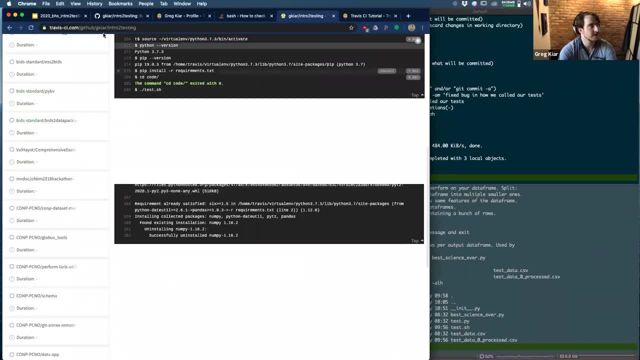 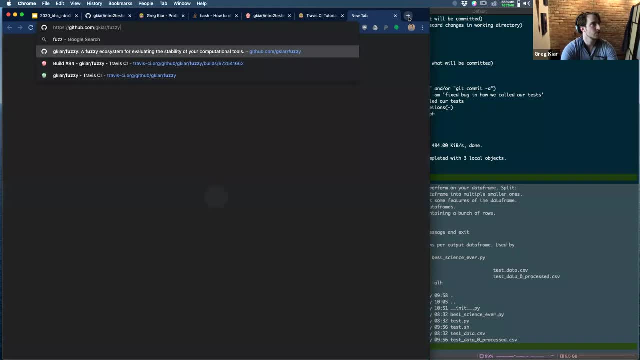 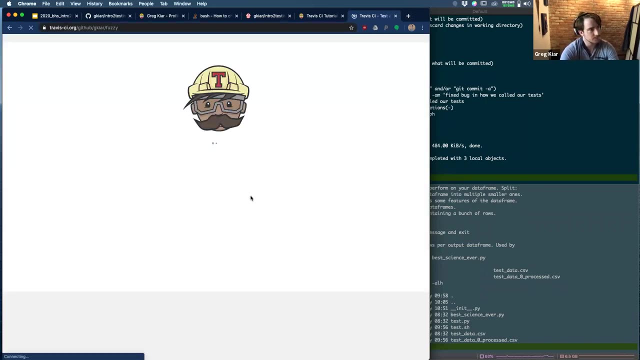 Yeah, that's a very good point And there's some examples that I mentioned. actually, I'll show you where you can do really complicated things and have parallel flows and stuff like that. So if we look at, If we look at this project that I mentioned earlier- you know, I have this project where 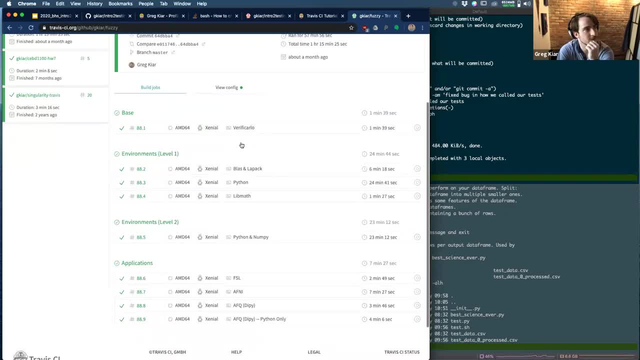 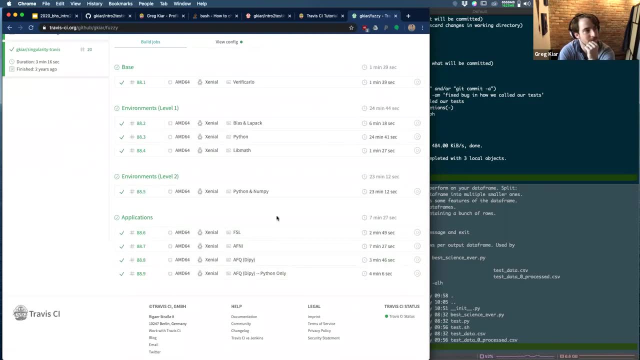 I need to build something and then, once it works, I can build other things upon it, and once those work, I can build other things upon them, and then, once that works, I can build other things upon them. So here we have a bunch of different build stages that are: 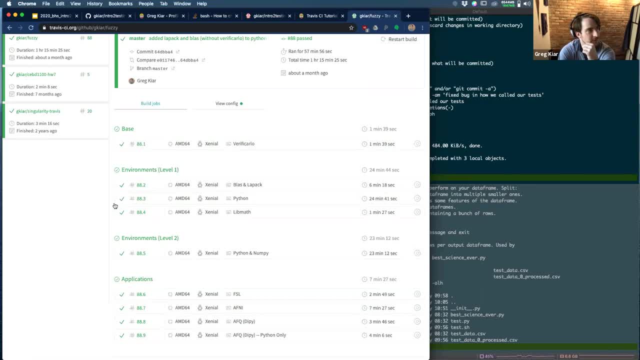 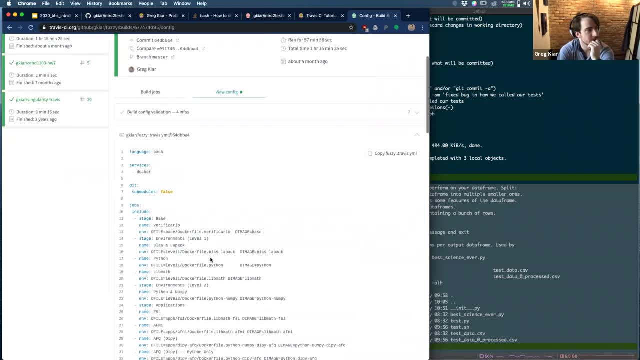 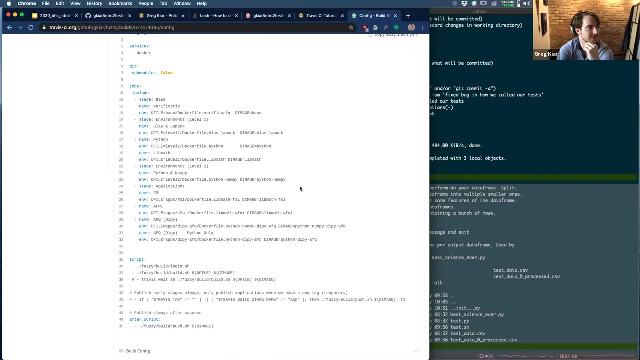 These ones can be parallel. but then the you know base to environments, one to environments two, and applications, those are all having to be sequential. So you can do lots of fancy configurations. So there's tons of you know messy logic that, if you again haven't seen this before, 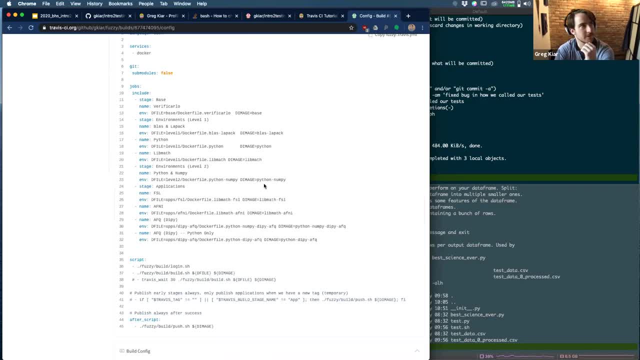 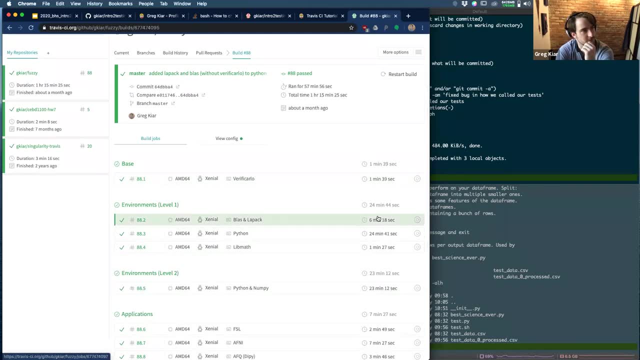 is totally intimidating but allows you to really make these complicated workflows that really let you test things very efficiently, rather than me on my computer having to, you know, build all these things which, as you see, in some cases takes like 25 minutes. 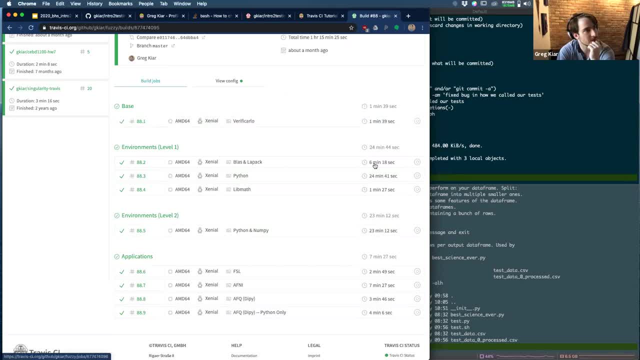 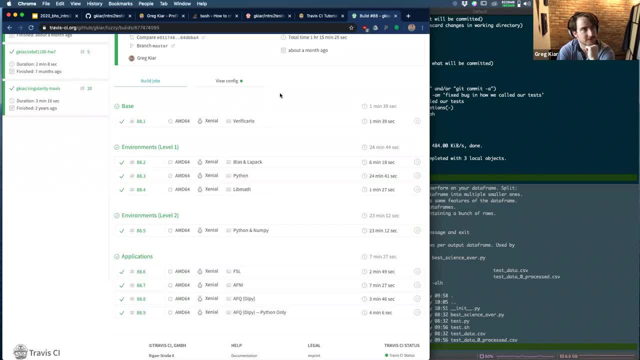 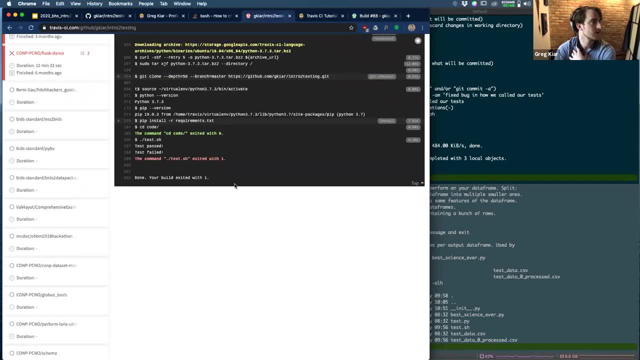 It's a lot of work. It's a lot of work, But again I'm able to get all my tasks completed, And again that's without any of my own time wasted on it. Cool, So now, if we go back to our testing script, the one I was mentioning now, we have exactly. 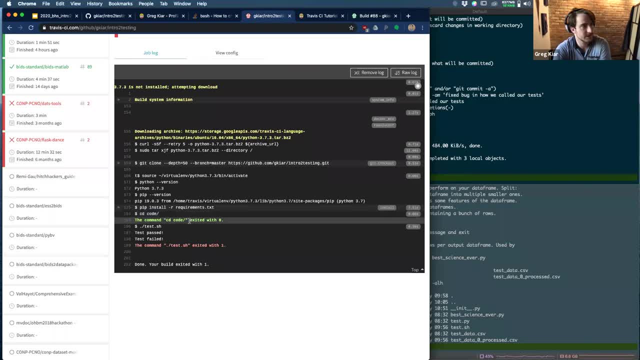 what we expected: We move into the right directory. That succeeded, That's good to know. And now we run our test script And the first test passed. The second test failed And that means that we left our script with the exit code one, meaning we still have a. 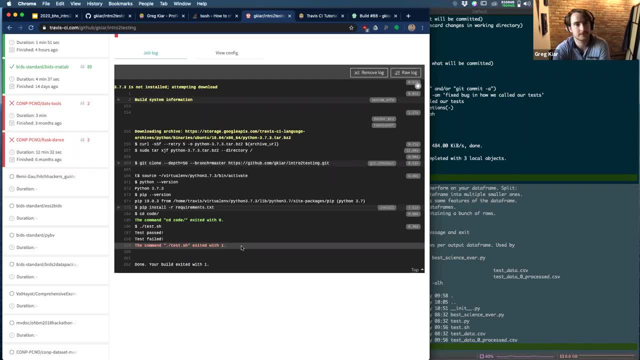 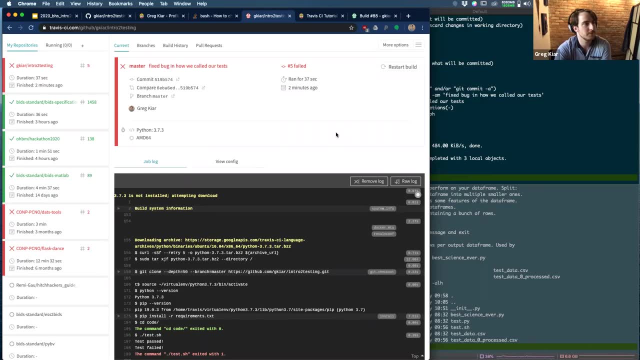 test to fail, And now we have a bug to fix, Or you know a bug to fix, rather. So this is a very basic type of workflow. I haven't even gotten close to talking about, you know, testing, and specifically with Python. 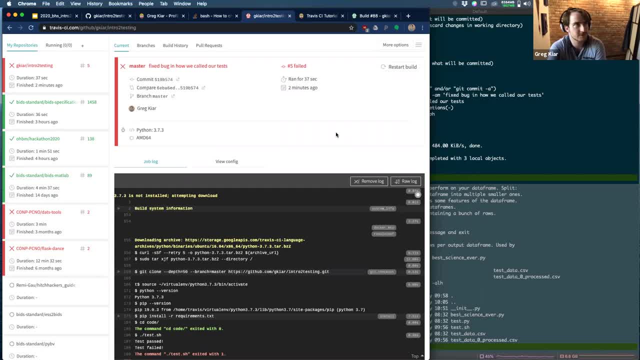 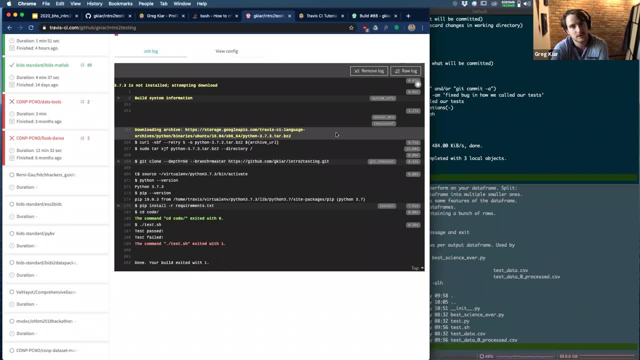 using a tool called PyTest. But again, these are all things that we can sync up on offline if anyone is interested. Testing is a massive topic. So is continuous integration, So this was just meant more to be like a primer on the way to approach it than anything else.